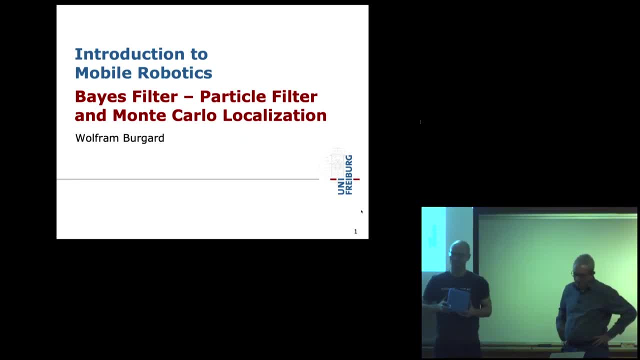 learn directly from the world expert, which is really nice. Please join me in welcoming Wolfram. Thank you Great. So I hope that sound is on. I don't hear it exactly. Yeah, it's good. Oh, we are done, Thanks. Thanks for coming. It's a great pleasure for me to be here and give this. 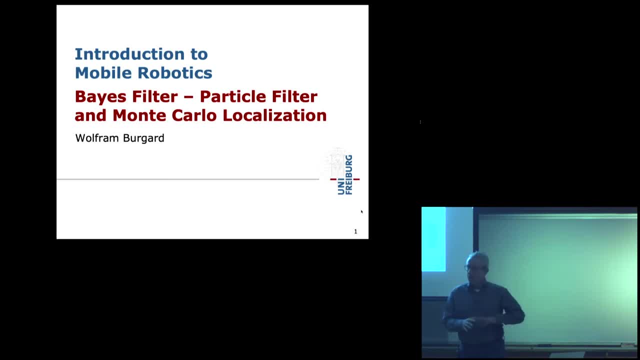 lecture about particle filters. A little bit of the context, and we are going to talk about the math behind it, the algorithms behind them, and then also like seeing a couple of examples of particle filters in practice And, if you want to know about application examples. 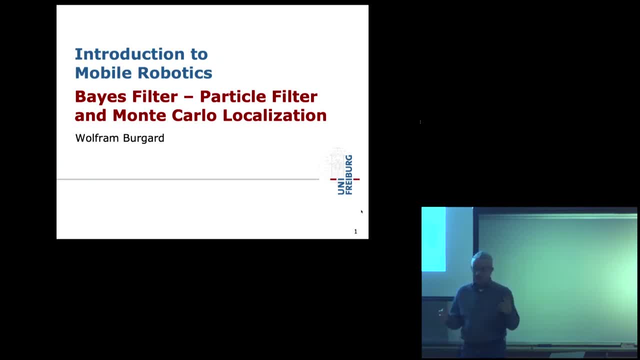 then I can directly tell you about what I'm actually doing here in the Bay Area right now. I'm working for Toyota Research Institute as VP for automated driving technology And, in fact, like building real robots that operate on the ground, So I'm going to talk about the math behind it. 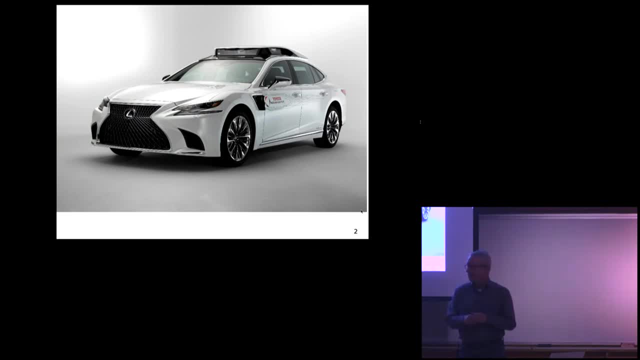 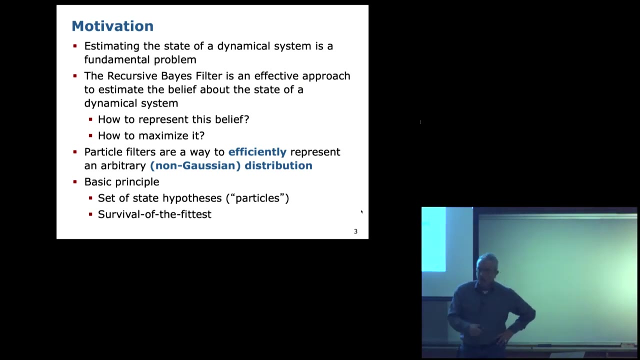 in the real world, like robots, like those over here, for those who need actually basically the technology that we're gonna talk about in this lecture, And if you wanna work with a robot like this, talk to me afterwards, Okay. so what is behind this lecture? 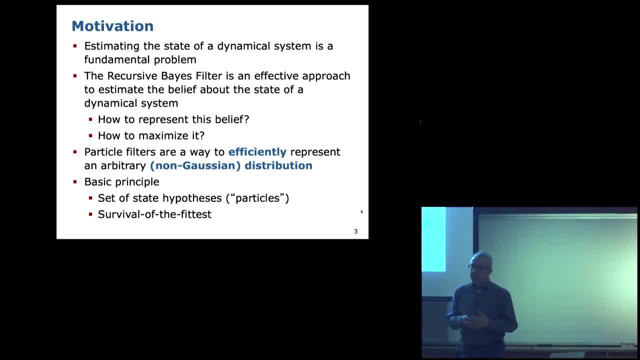 Usually, when you build a robot that needs to operate in an environment and doing this in an autonomous fashion, then it is usually helpful if the robot knows about its own state and maybe also about the state of the environment. Today, we're gonna mostly talk about the state. 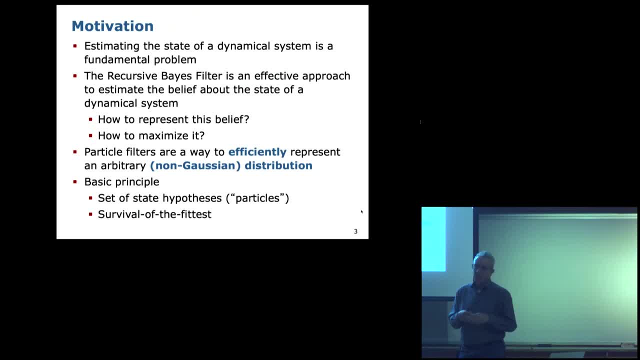 of the vehicle itself And the other, like more extended version of that, is only briefly mentioned, but in principle, the math behind this is exactly the same, as we're gonna talk in this lecture, And the algorithms that are used are also the very same. 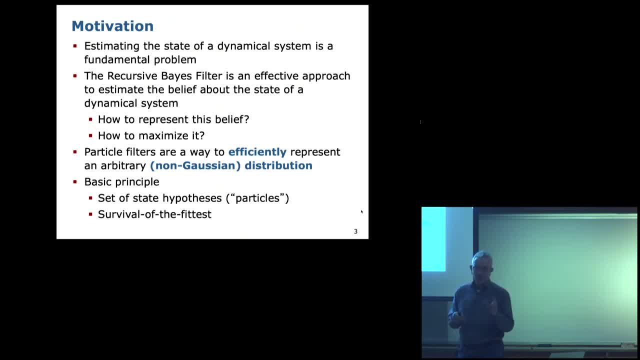 The only difference is the representations, and there's a particular trick that makes a state of the vehicle, the estimation in higher dimensional spaces, more feasible. So we're gonna talk briefly, recap the recursive Bayes filter- hopefully known to all of you, and answer that. 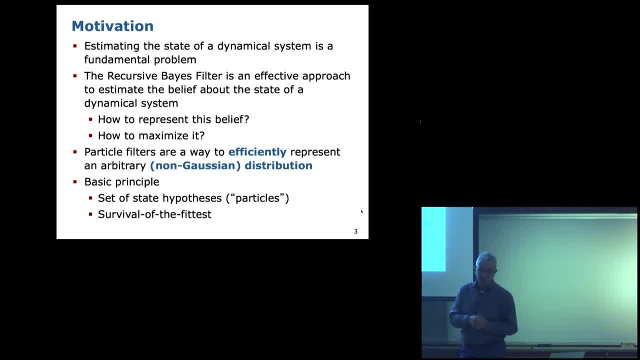 or attack that question of how to actually represent the belief of that as basically a probabilistic way, or probabilistic belief that we are representing equations in a few seconds. Typically, you also wanna know how to maximize it. We are not gonna address this in this course. 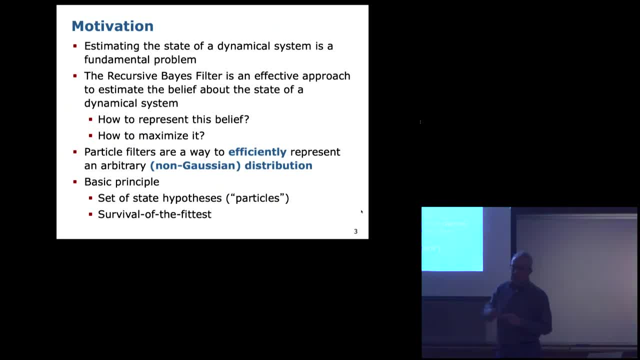 or in this lecture today, but we're going to talk about particle filters as an efficient way of representing such a probabilistic belief And, in particular, in situations where this belief doesn't look like a bell-shaped curve and it's rather a non-Gaussian distribution. 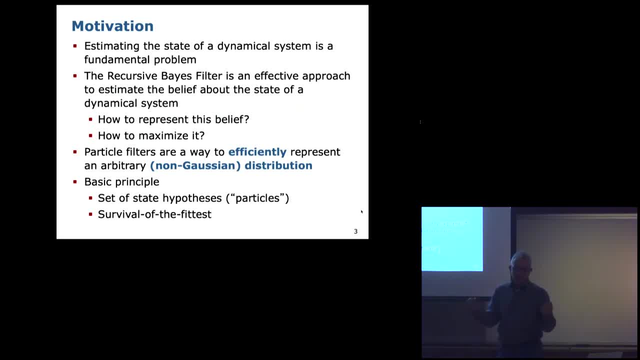 The key principle of that is that we're gonna have a discrete approximation of that belief by the so-called set of hypotheses or particles. Mathematically, it's actually not a set, it's a multi-set, because you cannot guarantee that two hypotheses are exactly. 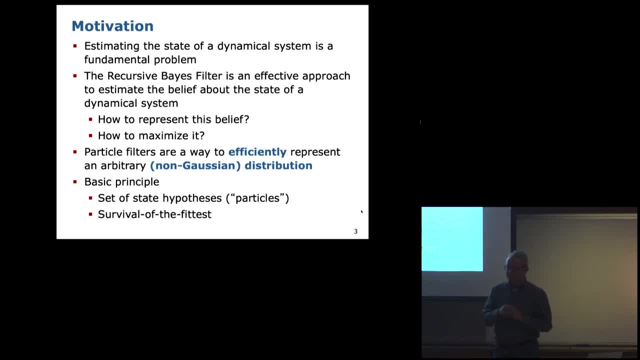 the same, So please apologize for the slight inaccuracy of notation there, But it is actually easier to speak, And what we, additionally, are going to use is the so-called survival of the fittest scheme. Maybe if you have heard about genetic algorithms or evolutionary strategies, it's very, very similar. 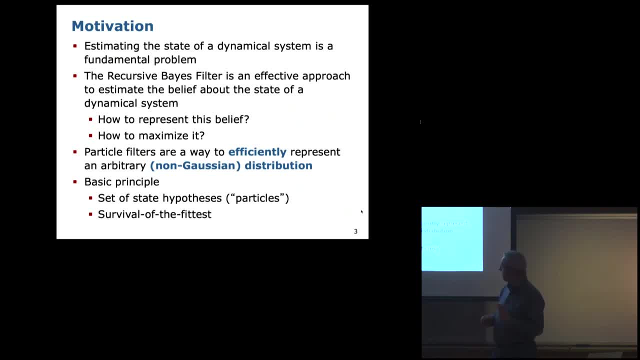 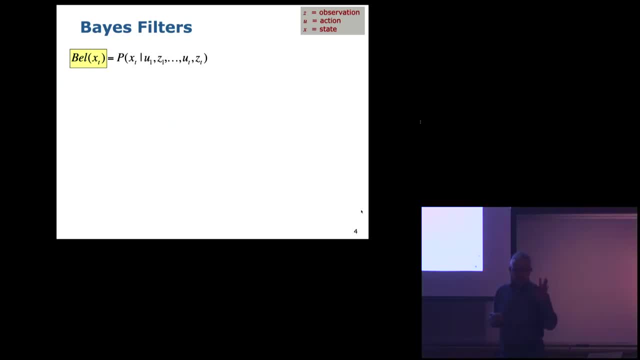 but what is going on in that representation in particle filters? Brief recap about Bayes filters. what we are interested in typically is: we wanna know, wanna have a belief about the state of the dynamical system, And this is basically something like a posterior distribution. 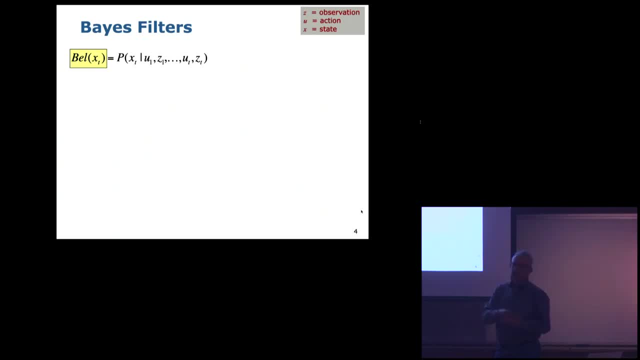 about the state, given all the actions that that system has carried out and all the observations it has made. And so u's are the actions and z's are the observations. Could be camera features and camera images, distances recorded by lidars, ultrasound sensors- whatever sensor you have. 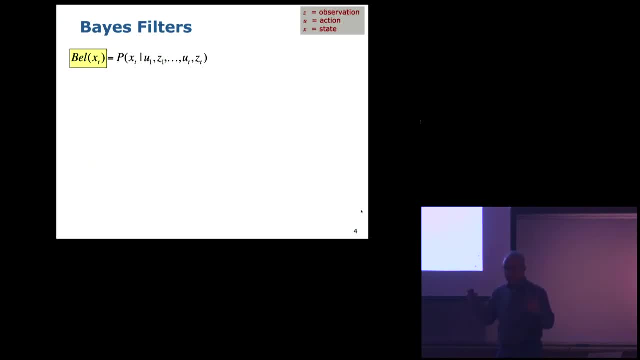 this could be the perceptions and the actions of a mobile robot, for example, are like the wheel turns, and that then, using odometry or odometers, are like, turned into like angles per second, And from that you can actually calculate what action the robot might have carried out. 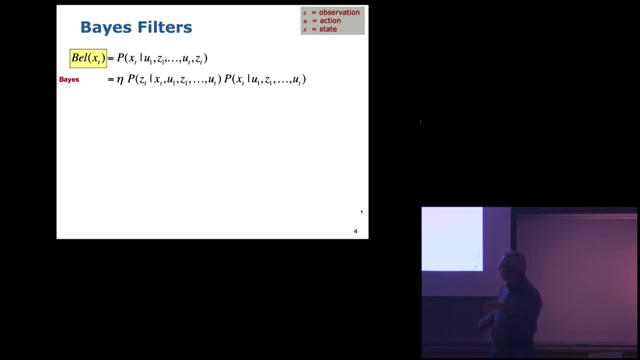 based on these wheel turns, All right, and using a couple of like mathematical derivations based theory, a couple of independence assumptions, law of total probability, another two Markov assumptions, you end up basically with this equation down here. And the nice aspect of this equation- 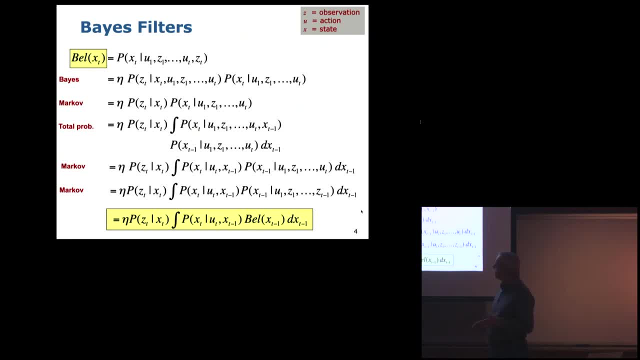 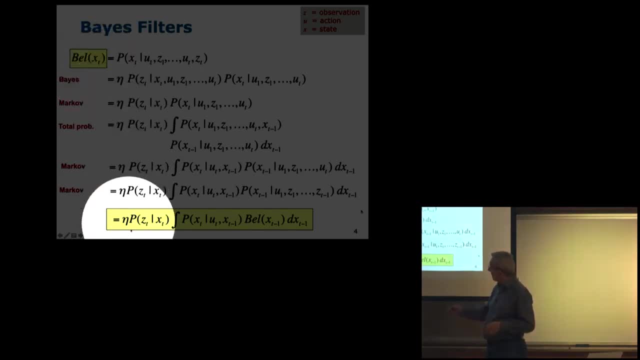 is that it is actually recursive. So what we're interested in is the belief, or here we are, the belief at state at time t, And we can reduce this to this equation over here, where we do have the belief at time t minus one. 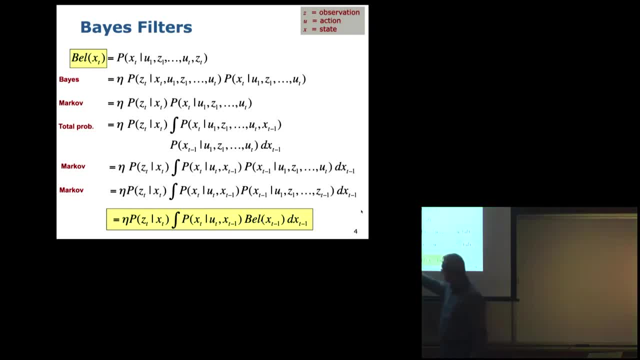 And there are two components in here. The first one is this: integral, integral, and. and the second one is like this: multiplication on the on the left hand side, and the terms are this one over here is we call this a transition model. it's basically the probability that you end up in state XT, given you. 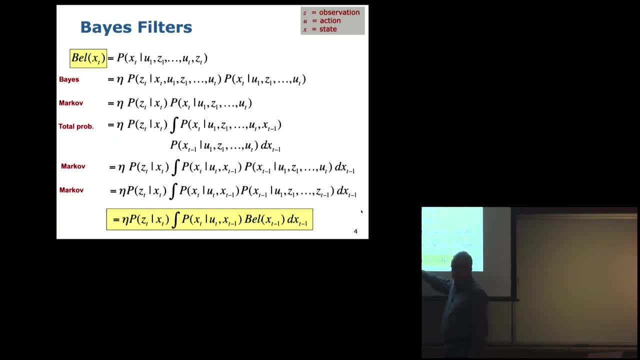 executed action, you at time T and we're at in state XT minus 1 before. it's a probabilistic way of representing the actions you know. so if you carry out an action and I want to actually describe the distribution about where I might end up, given I was in XT before and executed that action, so it's a known form mark of 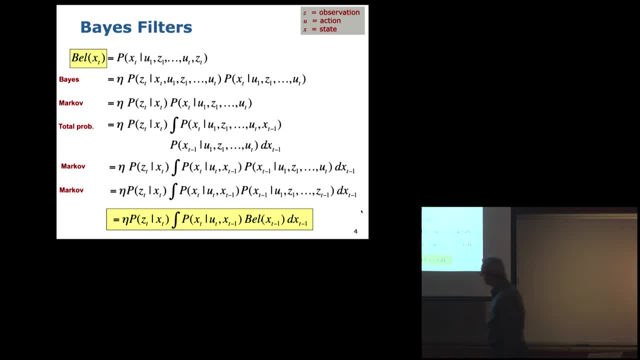 decision processes, reinforcement, learning, all these kinds of approaches, and this term over here is a so-called observation likelihood. which method measure which is the likelihood of observing this measurement? that at time T, given we are in state X at time T and you can see that we are in state X at time T and we are in state X at time T and? 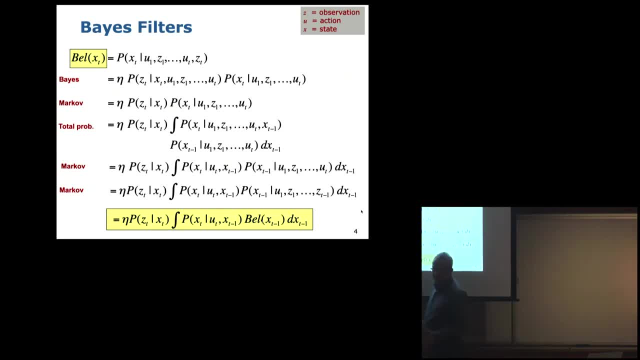 you can see that we are in state X at time T and we are in state X at time T and for those of you who are like neural networks, there's one operation that is also like typically present in neural networks. this is this part. this integral over here is basically nothing else in a convolution of that previous belief over. 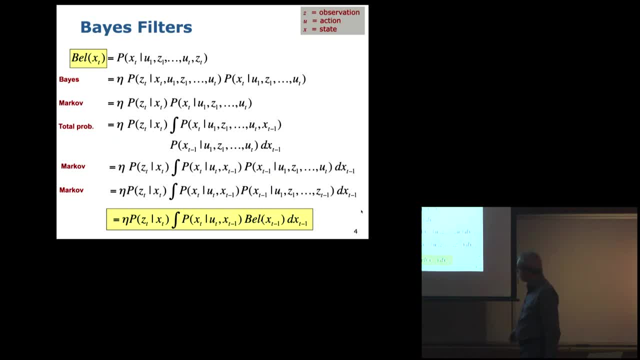 here with this probabilistic transition model of motion model. so we basically integrate over all potential prior states, multiply that those are the probability that we end up being in X, T, given that prior state, and then we multiply that resulting state with the likelihood of that observation. 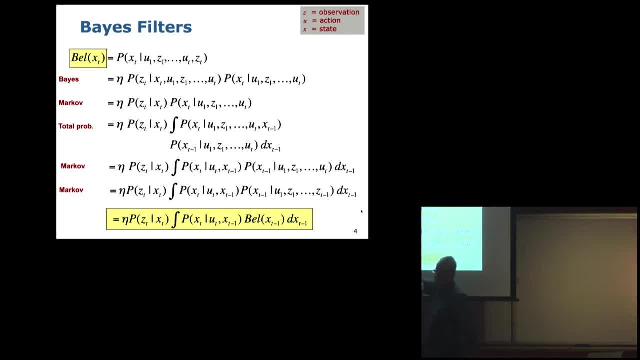 And this eta over here is a normalizer, making sure that the belief sums up to an overall xt And it falls out of this base theorem. It actually can also be analytically calculated And in implementations of this it actually falls off while you actually do this calculation. 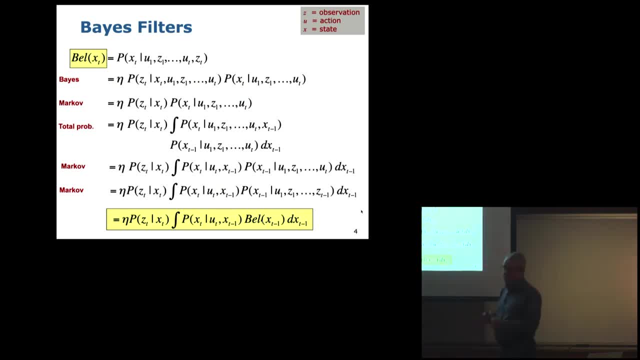 So even in the particle filter implementation we will later see this normalization happening in the algorithm. So this is basically how you can do like OGG, like concursive base filtering estimation for the estimation of the state of a dynamical system. That doesn't answer everything. 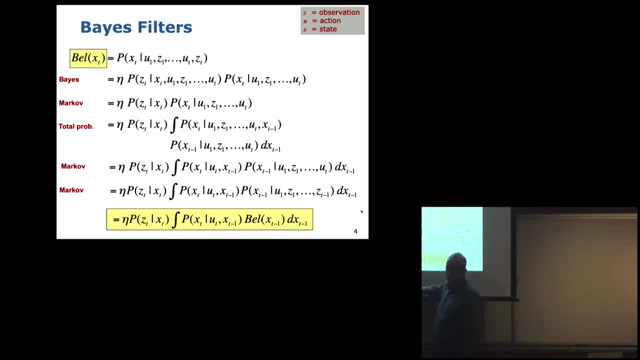 So typically what we need to specify for actually making that work on a real system is that model over here, the transition model- We will briefly speak about how they can be represented- And also the observation likelihood function. What is the likelihood? 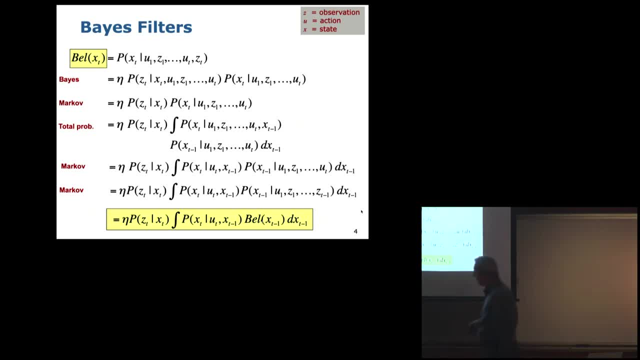 The likelihood of making a specific observation, given we are in a specific state. Both are really complicated typically, And the best way of obtaining them is to use statistics, making lots of experiments and figuring out how they actually look like so that we can, in the end, use them in this recursive Bayesian. 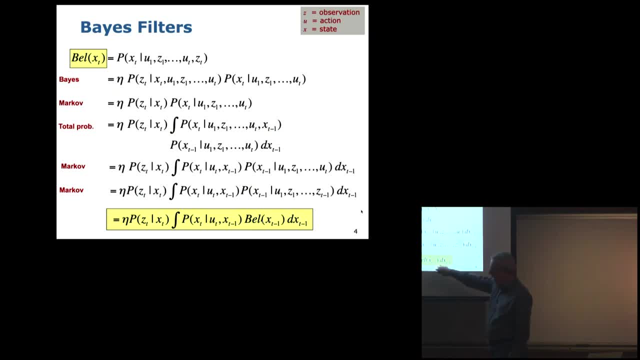 filtering scheme. In addition, what is unknown is what the prior is. So usually, if you do not know anything about the state of the system, you would assume that this is a uniform distribution, So robot can be everywhere or the system can be in every state with an equal probability. 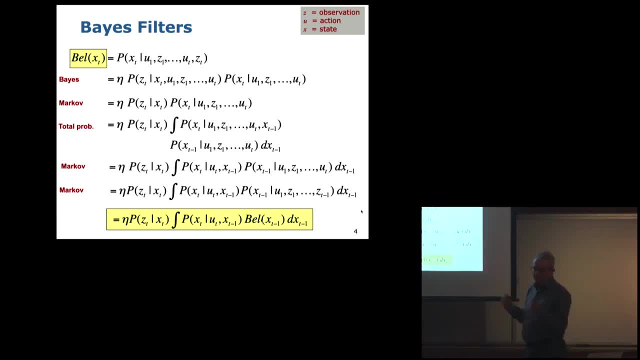 But the final question is how to actually represent this belief. What is the data structure that we are using in order to represent that belief? And there are a couple of implementations on the market, And one of the most popular ones actually is the so-called Paragfit. 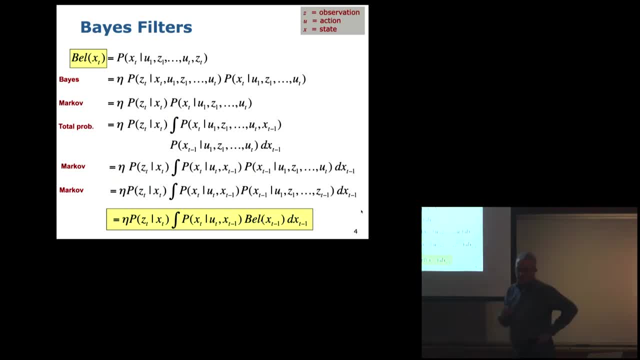 But what we are not going to discuss in detail here is how to maximize this belief. So we will actually, if you are interested in the maximum likelihood, answer based on all the information that you got. that is something that we are not going to cover in that lecture. 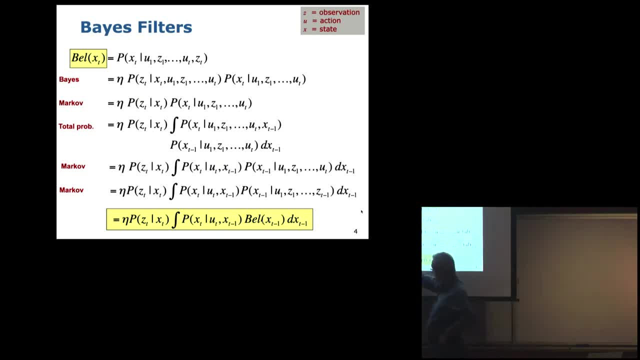 It actually requires another additional lecture, Even things like this transition model or the likelihood model. you can dive very, very deep into those and to have separate lectures about how to actually properly represent these type of models or more advanced versions of those. So if you think about an application of this, 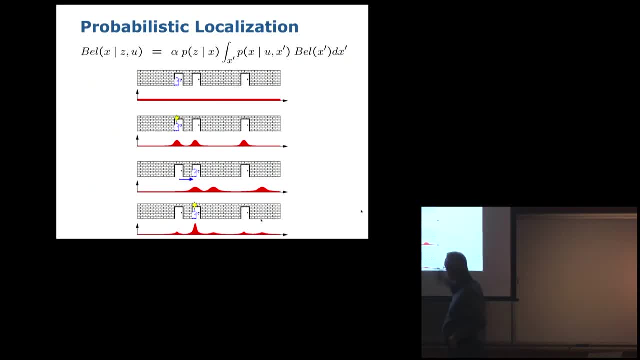 in the context of robot localization. this is a very, very simplistic example of a robot living in a one-dimensional corridor And all that the robot can do is actually moving forward and backward in that corridor. You could imagine this being a cleaning robot- vacuum cleaning. 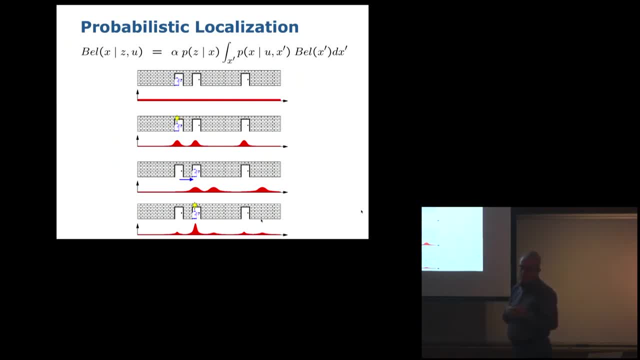 robot that does nothing else than collecting all the dirt in the corridor, And if you want to do this in a systematic fashion and not just moving around randomly, then you might use the position of the vehicle in order to figure out which places you covered and which not. 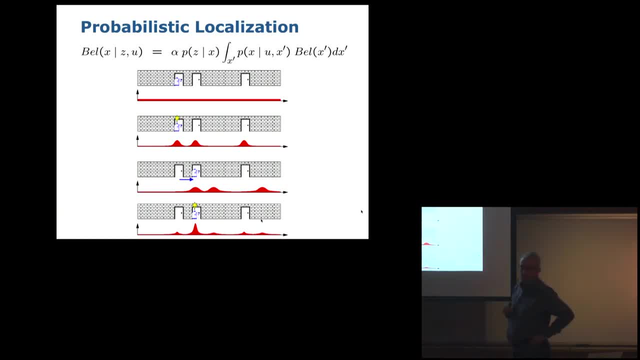 And for that the robot actually needs something like a probabilistic belief. And if you imagine that you switch the robot on in the morning- robot doesn't know anything about where you put it- then it might have something like a uniform belief about its current pose in that one-dimensional corridor. 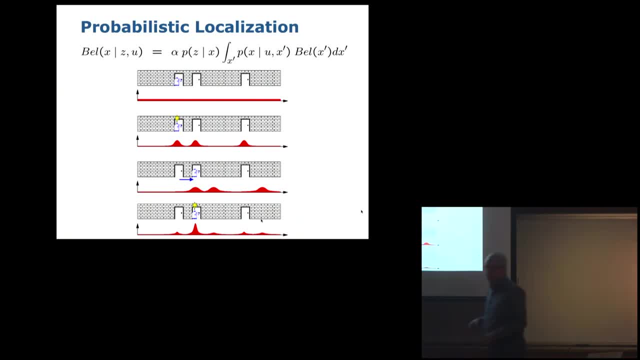 So the robot in addition has a sensor, And someone programmed a relatively simplistic likelihood model for us which basically says: when there's a door in the camera image, then the system says yes, I'm in front of the door, And when it's not, then the hope is at least. 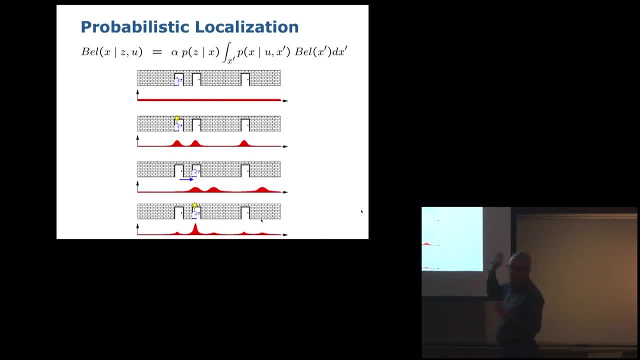 that the camera, that this system says I'm not in front of the door, But we are only using door detections here, And because we have also created some sort of statistics how often this door detector actually fires, And this is basically nothing else but that function. 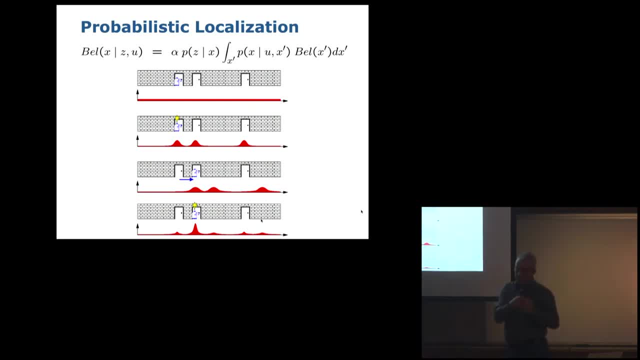 over here. Basically, the closer you are to a door, the more often it fires. So this is basically the likelihood of observing a door given that detector, depending on the state of the vehicle in the corridor. So now let's assume that we switch the robot on. 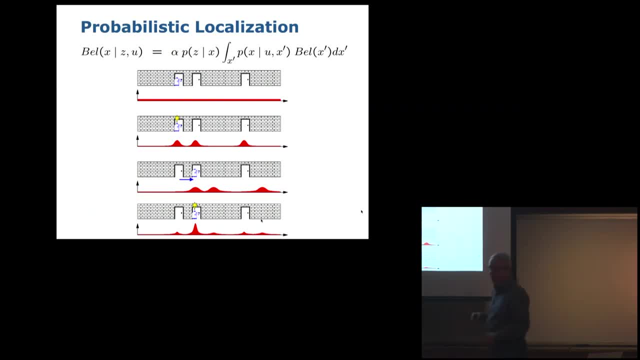 Just by chance, it is in front of a door. The camera fires and says: hey, I see a door. So it's basically that what we are observing is this measurement over here, this z. So our likelihood model looks exactly like this. 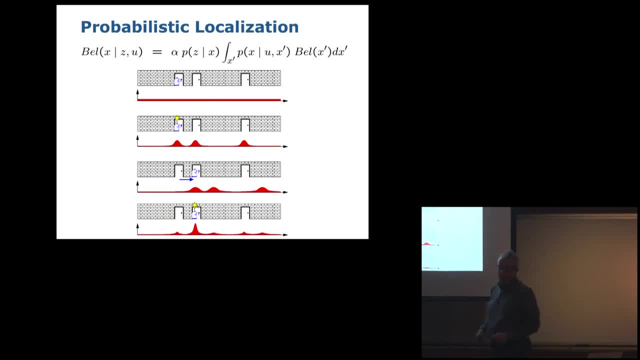 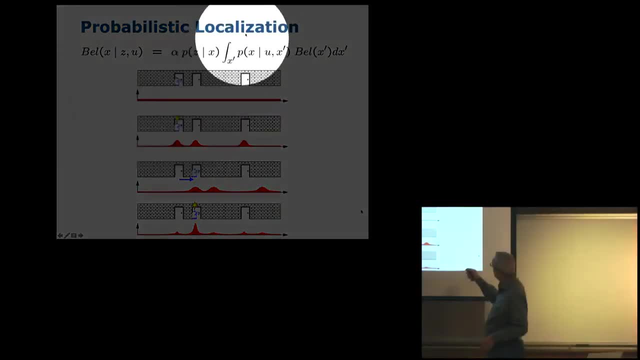 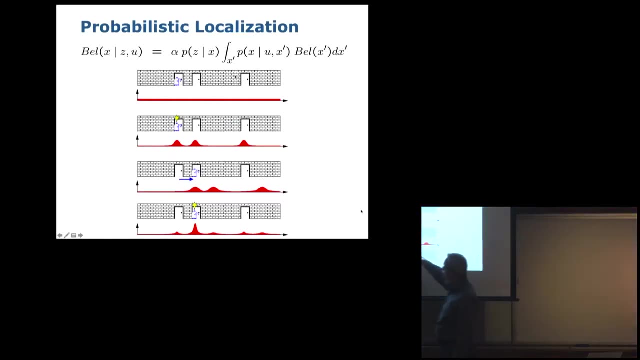 And we are now starting with the left-hand side of that equation. We're basically inferring from that, given that we had a uniform prior which is, instead of this, integral, here we are having nothing else but this uniform function, And p of z, given x is a function that basically 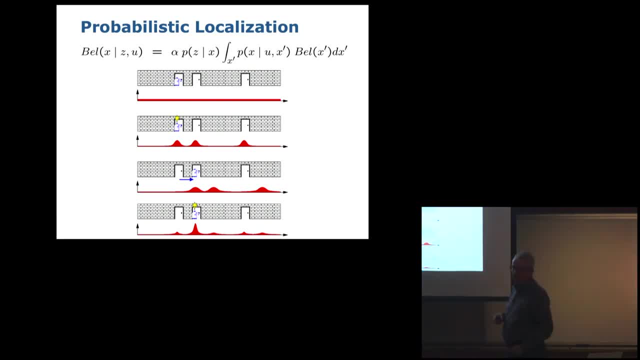 looks like this one over here. It's actually proportional to that. What we do now is we multiply our prior with our observation likelihood model and normalize it using this constant that I named alpha in this term, And what we end up having is a distribution like this: 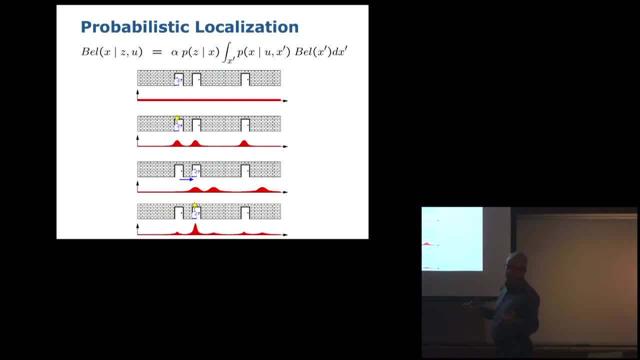 over here. All right, So It's actually the belief, then does not look any different than the observation likelihood model, apart from a constant factor. So now let's assume that the robot moves forward. The robot starts actually moving And typically actions increase uncertainty in most cases. 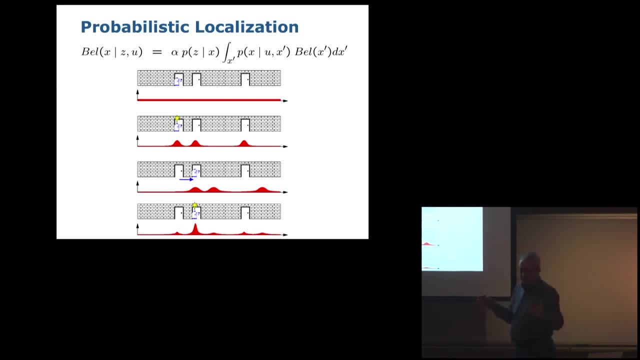 There are exceptions. So if I keep going, if I don't know where I am and I keep going for an hour forward, then it's very, very likely that I'm stuck in front of a wall in this room. But usually 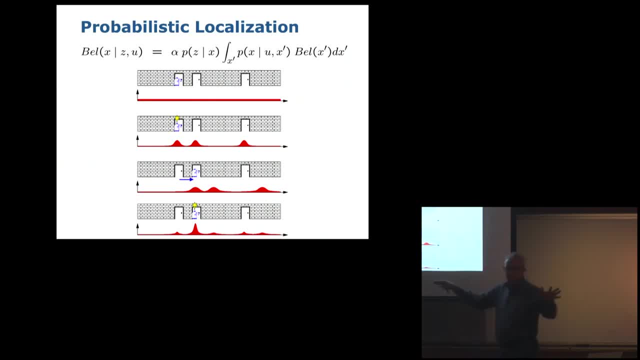 It increases uncertainty. So if there's only free space and I keep moving, then because of the uncertainty in my movements I will increase the uncertainty about my pose, And you can regard this as a convolution operation. It's basically this integral that you 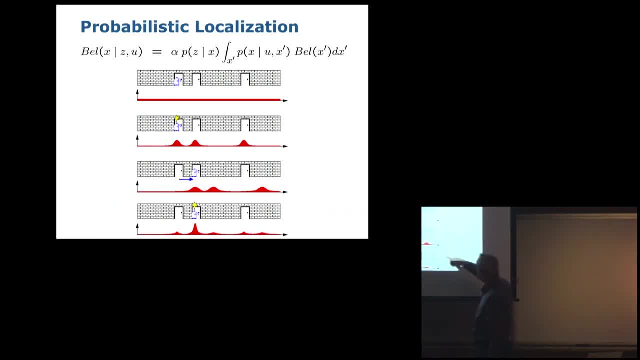 see on the right-hand side, What we're doing is we're taking our Kant belief and convolving it with this transition model. All right, We are basically calculating For every position, taking the belief that we have been at another position before and multiplying this with the transition model. 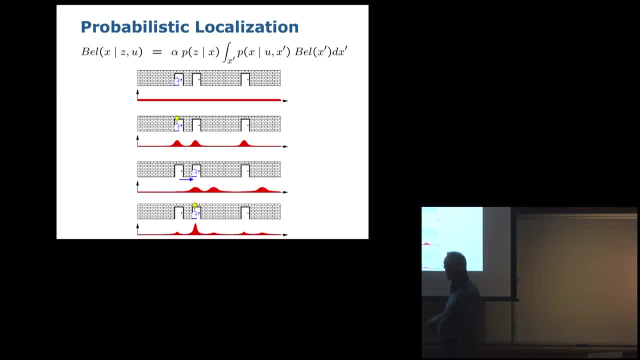 that we end up in x, given we were in x prime before. There's nothing else but convolving this, Or you can imagine this as a process of convolving this distribution over here and shifting it according to the movement. It would be a very, very naive implementation of this. 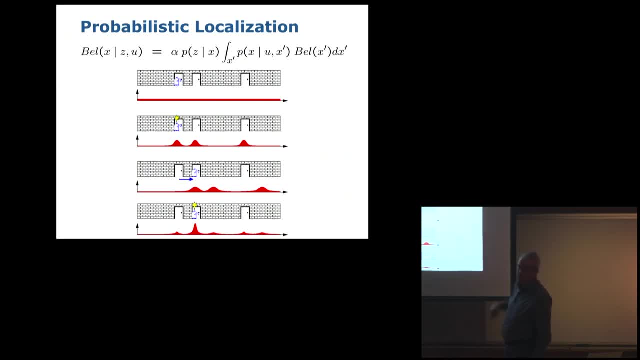 But in principle you basically need to calculate this integral over here, OK. And which means that this convolution operation can typically smooth things out and you get a distribution that is shifted and a little bit more flat, So the peaks are not that high anymore. 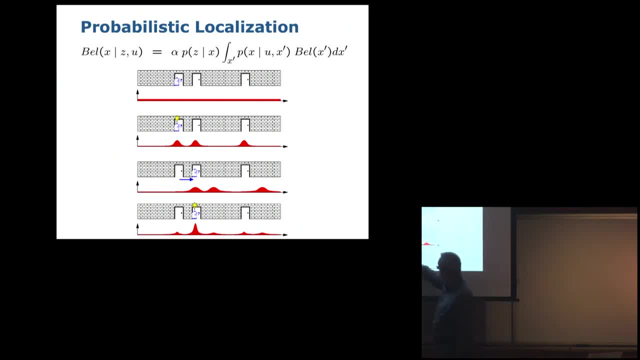 meaning uncertainty has increased. Now, let's assume, when the robot passes the other door, the next door, the sensor, the camera fires again. And what we need to do now? we are right now in that we calculated this integral over there. It's basically this function: 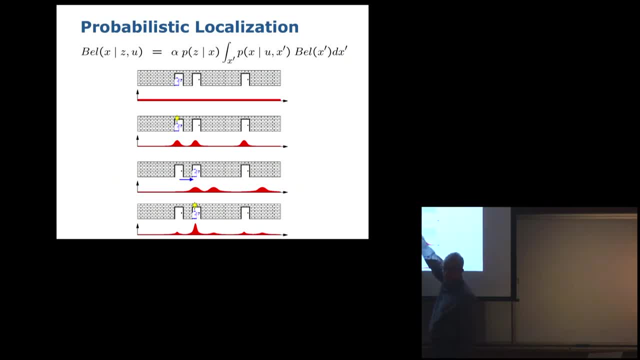 You get another observation. We basically need to perform this multiplication on the left-hand side And what we are basically doing now is we are multiplying those two functions over here to obtain this one down here. So this is basically that operation of the Bayes filter. 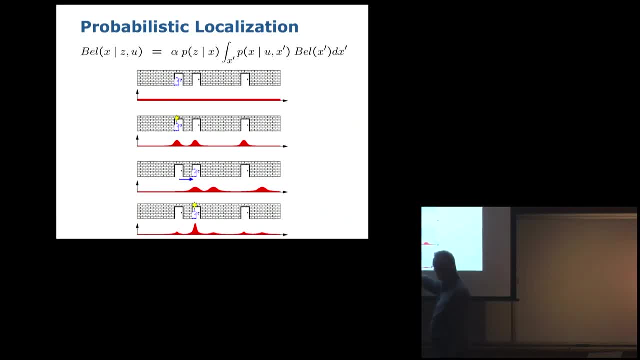 And once we normalize this, then we end up having this function over here And what you can see from it is we end up having five peaks in that distribution. Like one is consistent with two observations, There's this one over here And the other four are only consistent with just one. 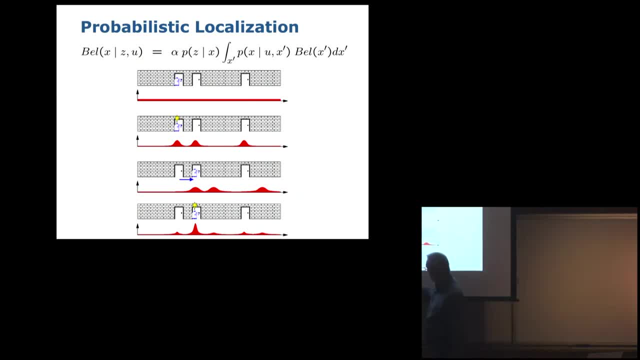 observation, And the interesting aspect is some are a little bit smoother than the others because they were the first observations And after movement, so they have been convolved, whereas those have not been convolved. That's fine. This is like how this function, how we obtain this function. 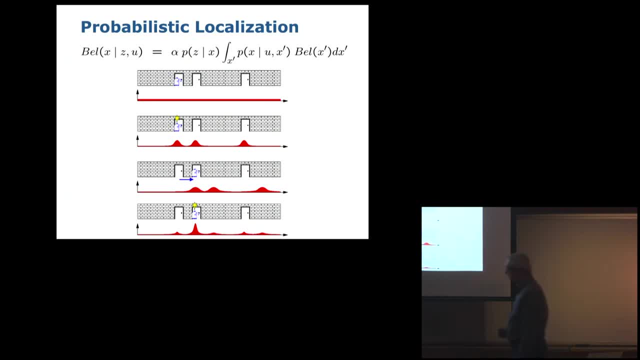 Because that really comes out of this equation up there, And the hope is that That we don't need this instant over and over and over again, because this distribution is consistent. So, yeah, So memory, Who knew that way? that the sixth order? 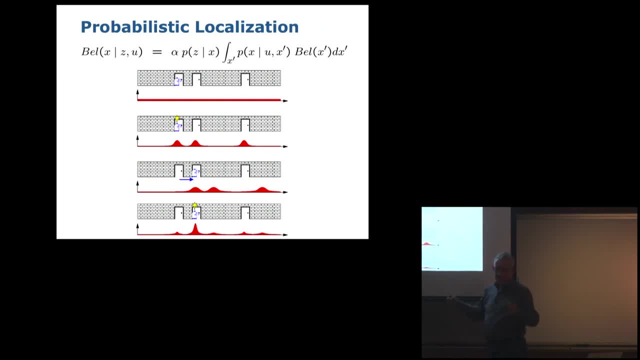 'd be actually hormones. That's really possible because it's the same amount of time right now, Because what happens is, as time goes by, in order to collect all the measurements and move around, the robot will get more and more certain, meaning that the distribution peaks in one state. so we can actually have a high certainty about what the current state of the vehicle is, That it doesn't necessarily need to be. It can even be that in ambiguous worlds, that the robots actually doesn't know in which state the robot is, because two rooms are absolutely identical, and keeps moving in in one of these two rooms. 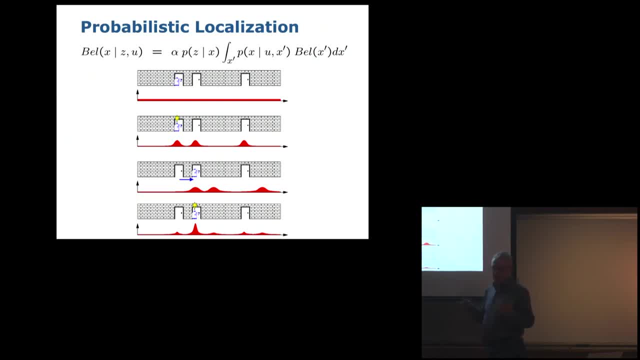 rooms, and then the robot actually cannot tell in which of the two rooms it would be, and that means that this distribution has actually two peaks. and then there's nothing the robot can actually do other than reasoning about its uncertainty and trying to figure out which actions it needs to carry out in order to minimize 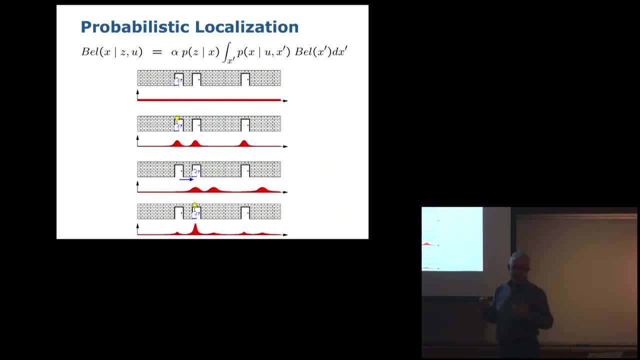 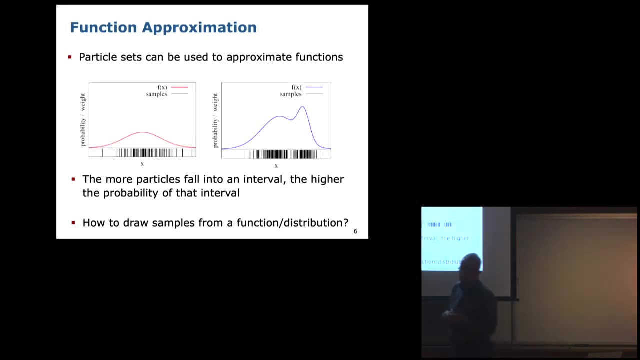 that uncertainty, which is kind of like that, what people do in active vision, for example. so key question is- and that's what we are going to answer in this course- is how can we represent such a distribution? and it means that we need to do some function approximation and an interesting way of representing 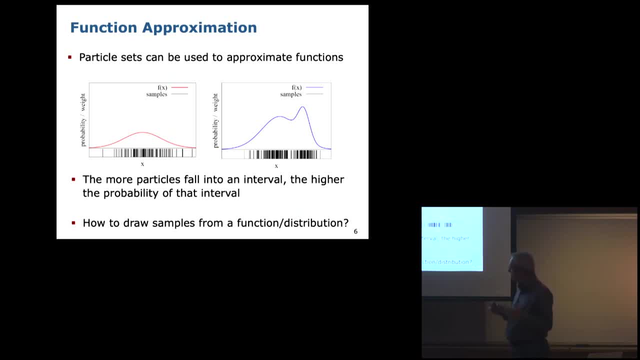 distributions is using particles or so-called samples. so imagine that we, like have a distribution like this function F over here and you want to represent these by samples, this distribution or function, then that what we basically, what we can do, is basically have higher density of hypotheses or particles in places where the function has a high 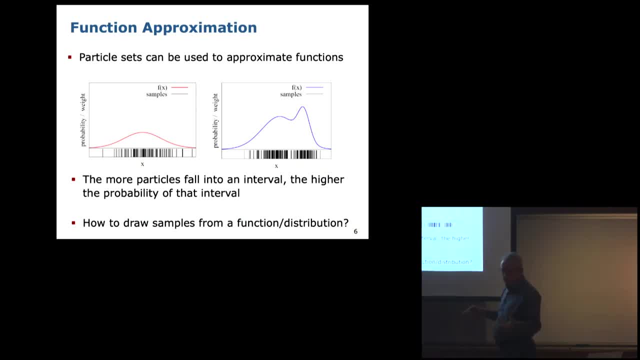 value and lower and a lower density where it has a low value. so basically, what that means is that if we integrate locally or we count the number of hypotheses locally and that gives us an approximation about, like what the actual function value is, all right so, and you can do this with. 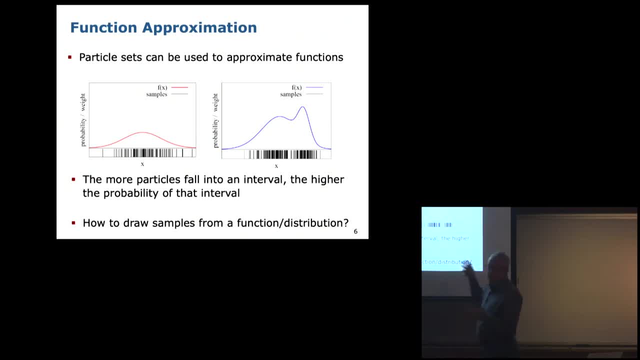 arbitrarily shaped function. techniques like these are used, for example, in if, when you do integration- Monte Carlo integration is, if you know, this is very, very similar to that- basically sample randomly and then you evaluate the function and this gives you, in the end, the area under the curve. but there's 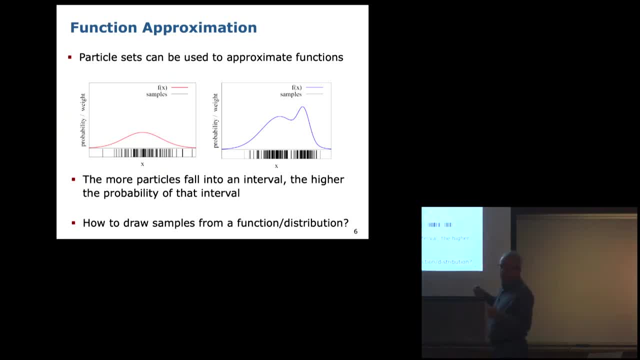 something here. we just collect these or have samples that are actually more dense in places where the function has a high value and and less dense everywhere else. the question is, how can we get such a distribution? so how we can we get hypotheses or samples that are distributed according to a specific 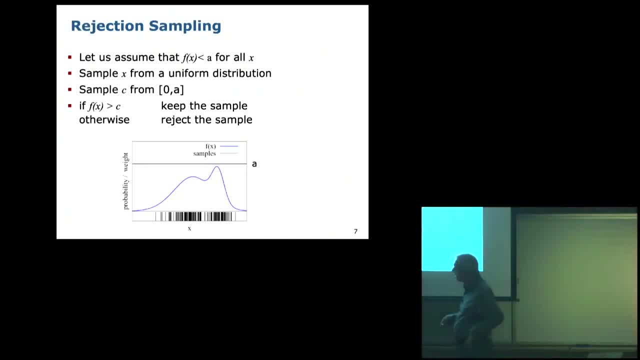 function different ways. for doing this, one very, very popular approach is the so called rejection sampling approach. so let's assume we have this function F over here and you want to have samples that are distributed according to that function, and usually you apply schemes like this for functions that are easy to. 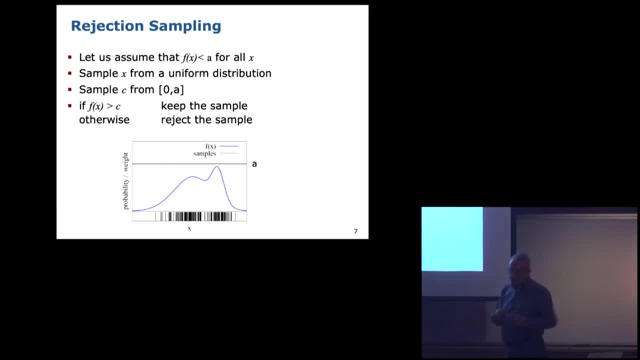 evaluate but hard to sample from which, for example, is the case for a motion model. that can be an enormously complex model that you can like. an analytical function you can easily evaluate, but it's hard to actually generate a distribution of particles from that function and rejection sampling works as 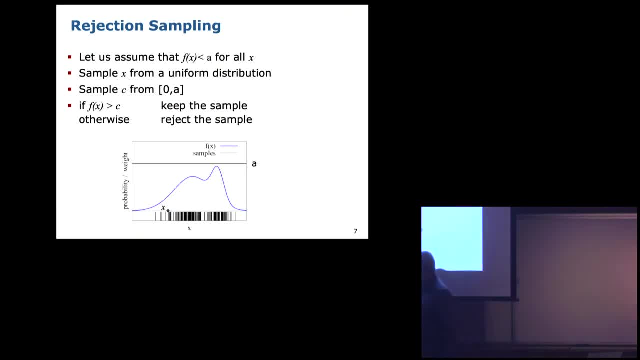 follows right. you basically sample in that interval of interest like a uniform value. let's assume that is X in this case again, sample another value, that's a so called Y value, that is, lies between the max of that function and 0. that will be like this: F of X, this would be this constant C over here, and then you make a. 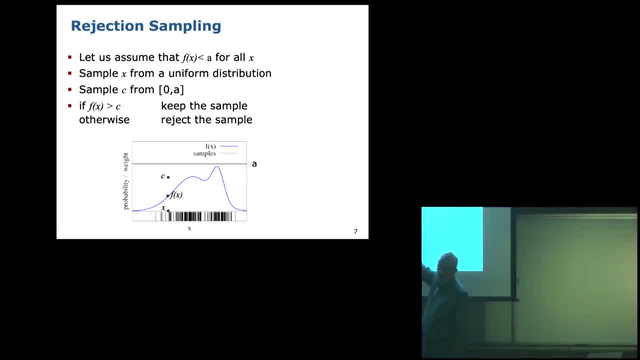 very, very simplistic test. mainly, if F is larger than C, then we keep the sample, otherwise we reject it. which means that if this comparison over there make sure that in places where this function is very, very low, there's a very high likelihood that this sample is rejected. 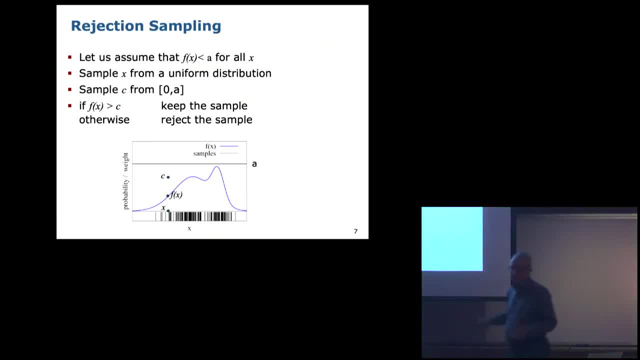 And so in cases where the function's high, there's a higher probability that it is kept. So you direct that x, we draw another x, like we have f of x over there, x prime, and we sample c and then f of x prime. 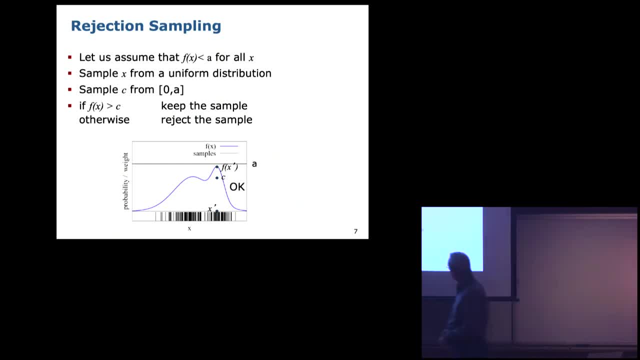 is larger than c over there, so we keep that x. So this is basically rejection sampling. Any idea which type of function is the worst case for this scheme? The professor was first, but I'd ask the student: A uniform distribution? Let's assume we have a uniform distribution. 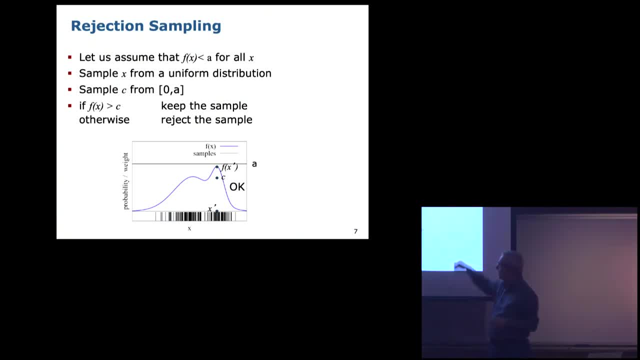 So it's a constant value. We do have any type of constant that is beyond that. Let's say that the max of that uniform distribution is a. the max that we sample from is b. The ratio that we keep that sample then is: 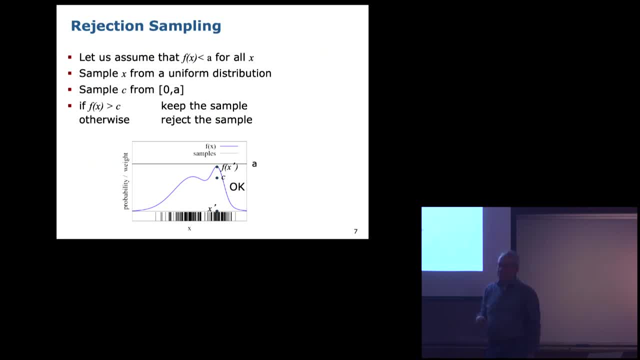 I think a divided by b, something like that. That is depending on where b is. it's not that bad If b is close to a. if b equals a, then it's actually the probability is one that we keep it right. 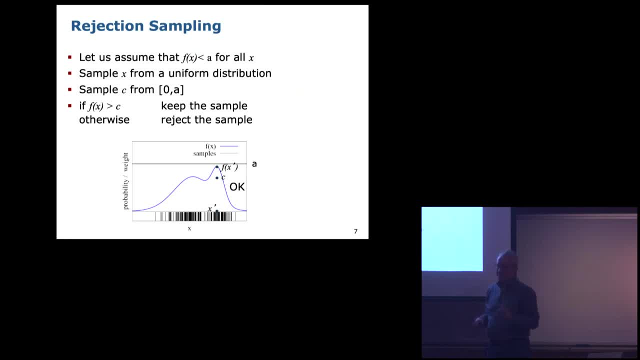 That is actually relative, Relatively, basically the best case that can happen, right. But what is the opposite of that uniform? What? Yeah, it's a Dirac distribution right, Or it can be like a sum of Dirac distributions. 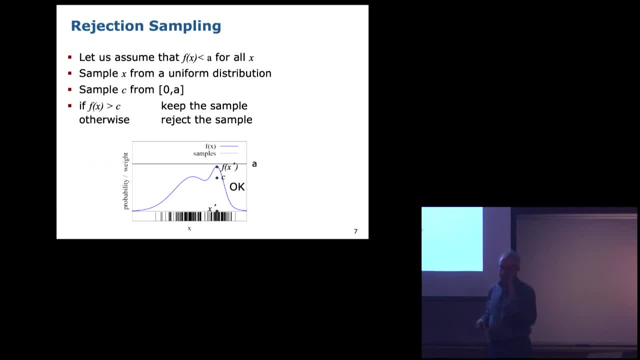 like, if you have only one peak where all the probability mass accumulates, right, You basically so that you have just one peak over here and if you have this gonna be sample one over here, it's zero, you withdraw it, right? 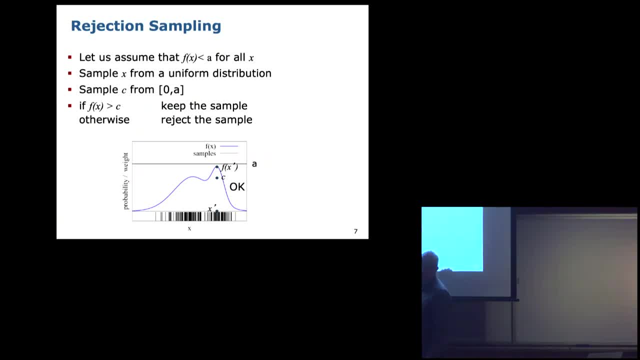 So the probability we hit exactly that peak in a continuous world is virtually zero, right? How long will this algorithm run? Forever, good. So you actually need to keep track of that right When you implement it. So don't be naive, right? 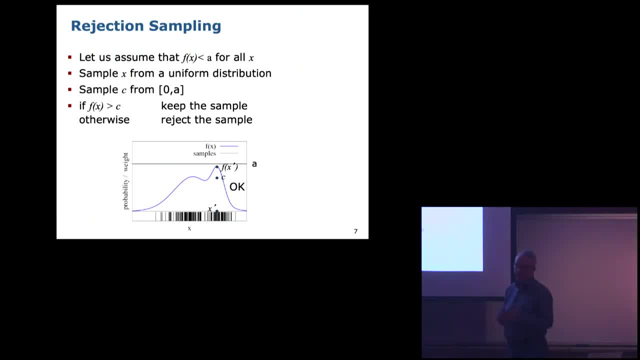 If you use it, it can actually, depending on what your function looks like, can be enormously complex, But the advantage of that is you can sample from an arbitrary, arbitrary distribution, which is pretty cool. The other thing is like here in this: 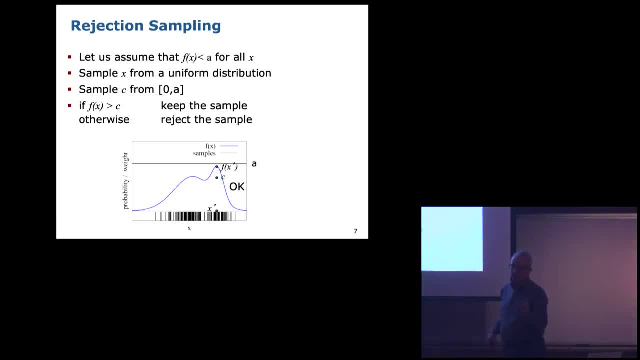 and this is why this is important. in a computer, every programming language typically has a way to sample from a uniform distribution. It's your RAND operation or whatever that is called in your favorite programming language. Samples from a uniform distribution, But sampling from any other distribution, right. 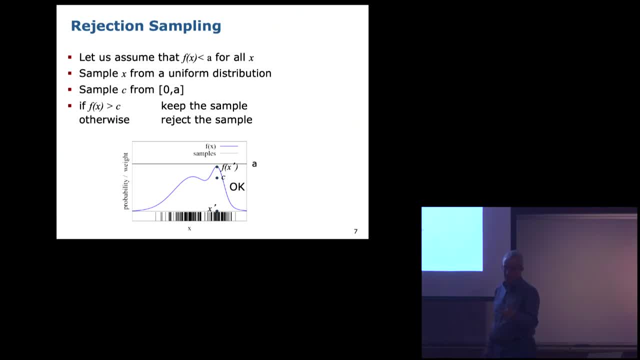 We don't have a random number generator for or a sampler for, right, So this is basically a way. if you want to sample from, for example, a Gaussian distribution, you can exactly use this scheme. There are more efficient ones, pretty cool ones as well. 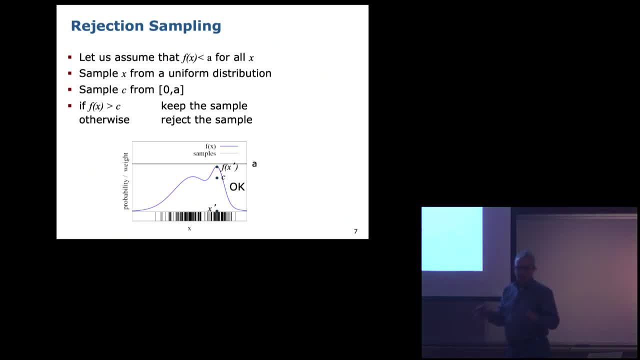 But if you want to do this, then you can actually sample from an arbitrary distribution. It's important here to see that we sample from a uniform one in that case, So, but there is a way to actually use non-uniform distributions as well. 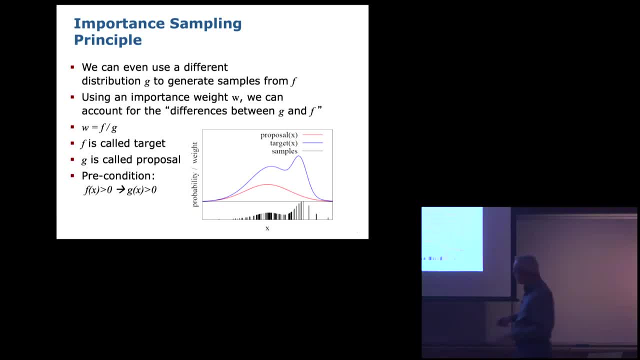 And this is the importance of sampling principle, So like, if you want to sample from this distribution, we do not need to sample from a uniform. Let's assume we do have a way of sample from a more informed distribution, right Like the most informed distribution would be. 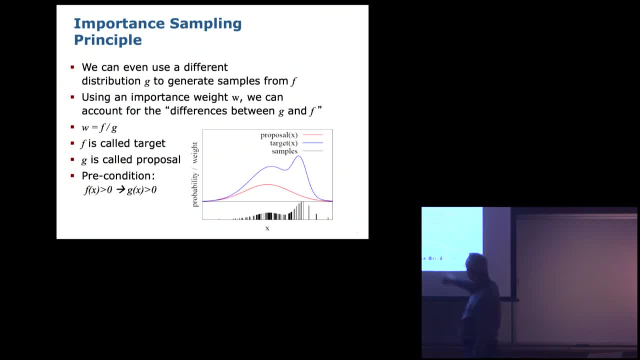 the target itself F itself right. So what we are using is the proposal- this is the red one here- to actually, and the hope is that with the proposal we get as close as possible to the target, because then we get the samples already in places. 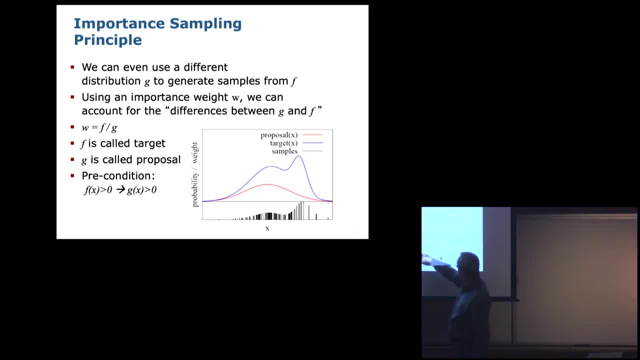 where we want to keep them. So, but the idea here is that we can we have a different distribution that looks more closely than F, than the uniform distribution. The only thing that we need to do now in addition to that is take into account. 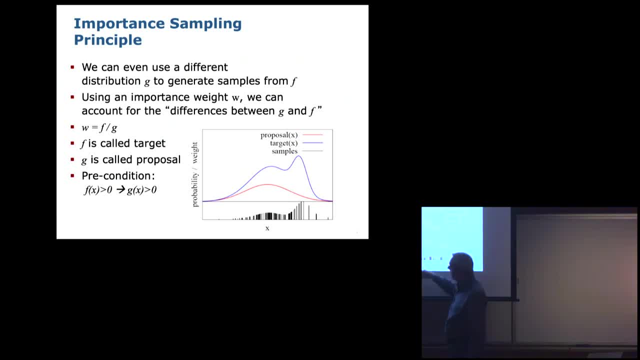 that we didn't sample from a uniform one, And in order to do this, we calculate a so-called importance weight. So we give these samples a height of they look like like towers right all of a sudden, And this is basically nothing else but the. 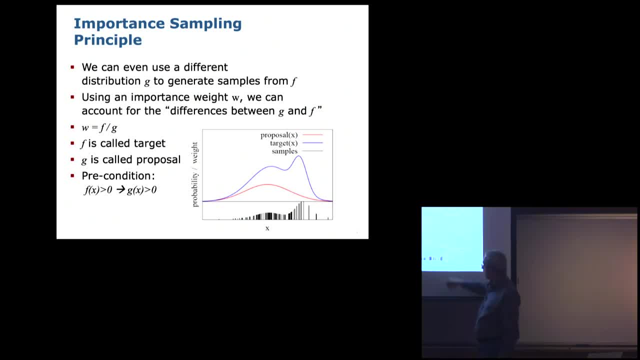 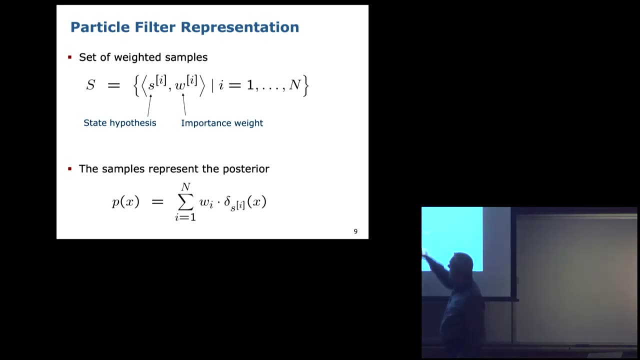 the ratio of F divided by G, right, That's basically the height of these samples. So, and this principle is basically underlying, mathematically underlying, the particle filter algorithm. So what we need in particle filters, the representation, is nothing else but a set. 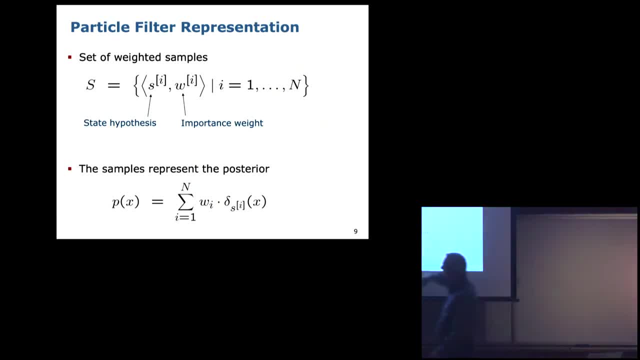 a multi-set, mathematically correct, of hypotheses And importance weights, and one weight for every, for every particle or hypotheses. Mathematically right, because these are just peaks. right, We have this, this weighted sum of these Dirac distributions, over here, right? 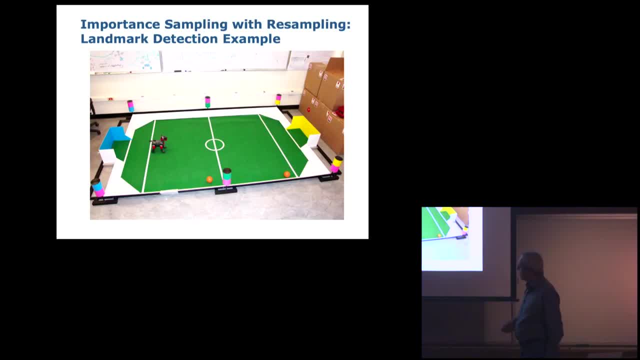 So this is basically the posterior that we're having, Just to give you one primitive example of how that works. it's actually an example generated by Dieter Fox. It's the old times of RoboSoccer with AIBO robots. 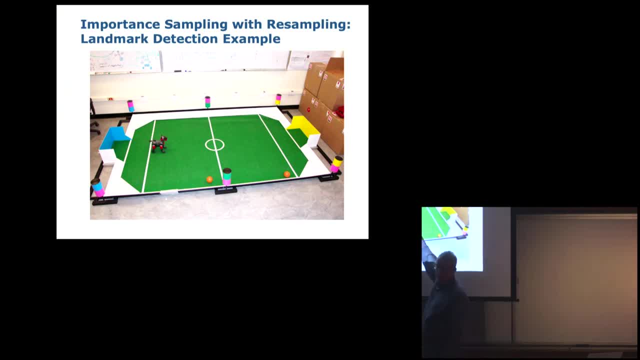 And at that time they had the soccer fields with landmarks and they had relatively simplistic landmark detectors, which was just using the color code And you can actually estimate the distance to that based on the size of that of that color coded field or segment in your image. 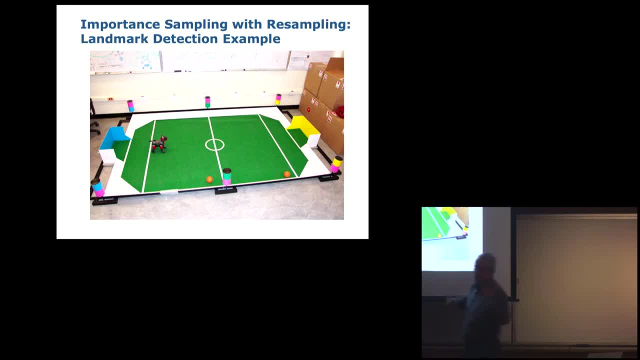 And so then you get some information about the distance, but what you don't get- because these are circular landmarks- you do not actually. you only get the bearing to the landmark. you get actually bearing and distance, which means that you usually, when you observe a landmark, 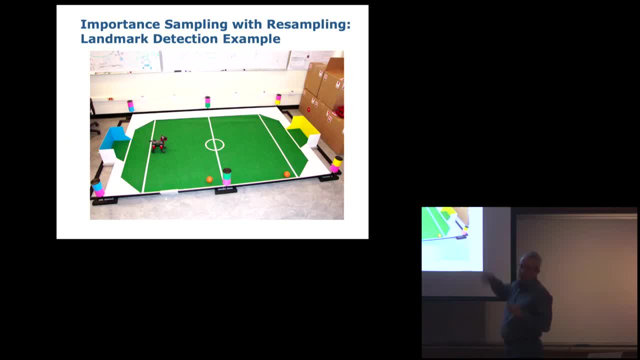 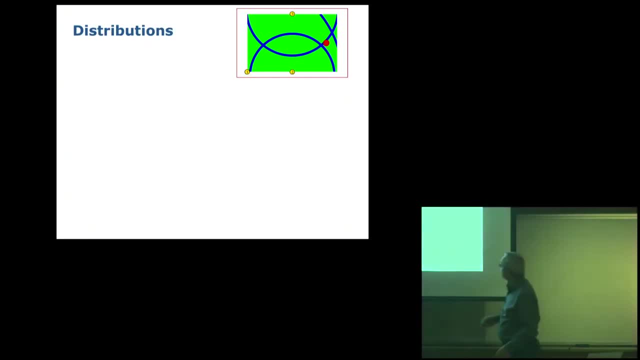 you get something like a circular distribution around that landmark and the radius of that distribution is given by the estimated distance. So geometrically for an observation, like when you see, when we see those three landmarks, one, two and three, 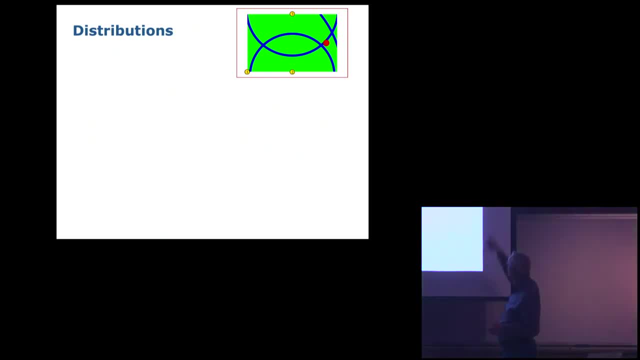 and like get the appropriate distances calculated by the size of the segment, then geometrically they would look like this over here, And what we're interested in now is like getting a probabilistic belief about where the vehicle might be or the robot might be right. 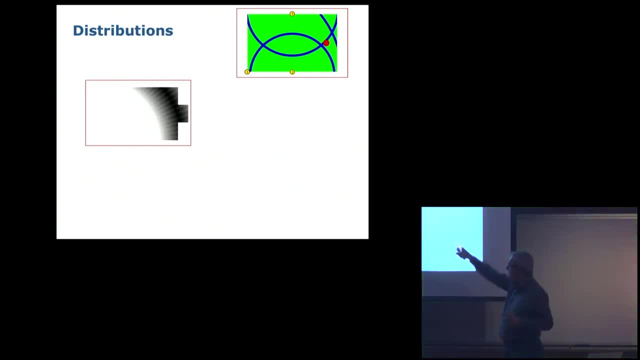 And if we do this, like in a probabilistic fashion, let's assume this is our P of Z given X, there's actually that function expressed here in a discrete fashion and you can actually see that by these pixels, that in the image right. 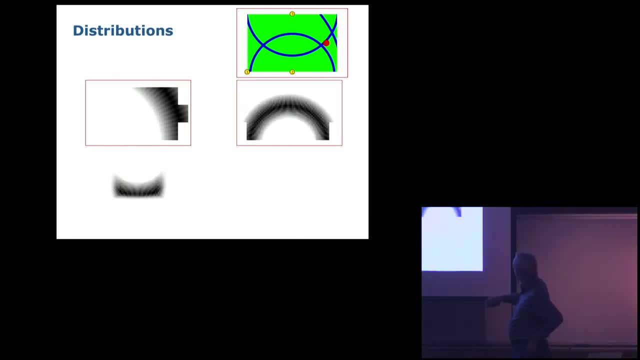 So again, like for distribution for the landmark two and for landmark three, and normally like, if we were able to just like get these directly right, Then we can multiply the three and then we get this distribution over here as a posterior about where the vehicle might be. 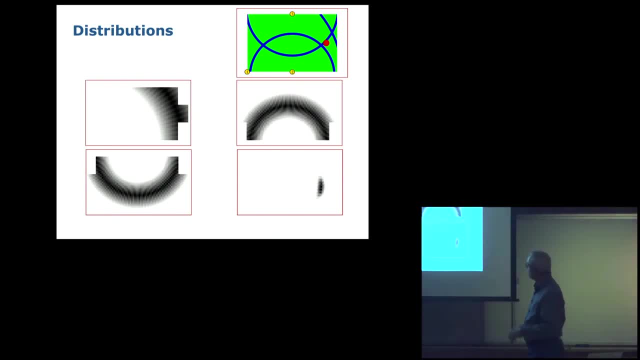 based on just no movement, just the multiplication of these distributions. But now, in a sampling-based world where we have particles, like we cannot directly do this anymore because we do have these particles or we want to reason about these particles and what we need to do now is like stay in this representation. 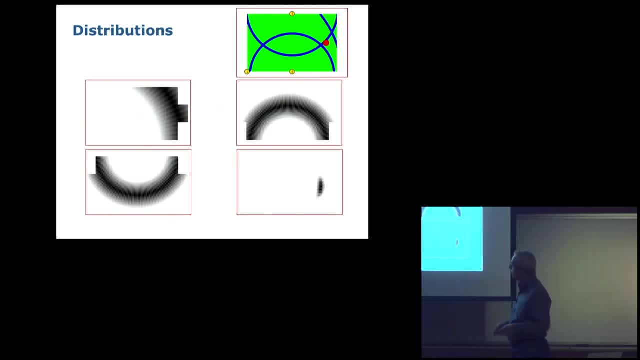 and keep these particles as the belief over the state of the vehicle. And here is where what we want to have. you want to have samples that are distributed according to those three distributions. In fact, we could now, like, take those three distributions and multiply them and then sample from that result. 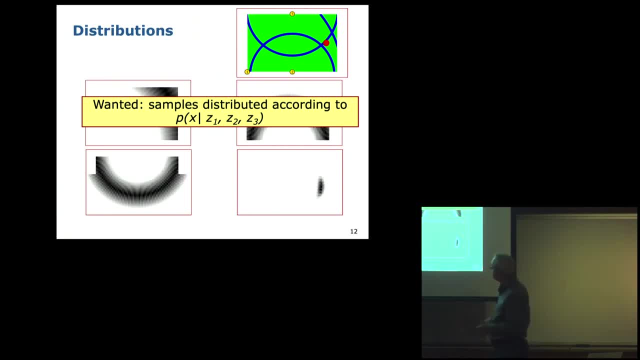 but then that's actually not that what we would like to do, simply because the maintaining such distributions can actually be enormously complex. Now, because it need, like this is a two dimensional field that we need to hear about in higher dimension cases, This can actually be. 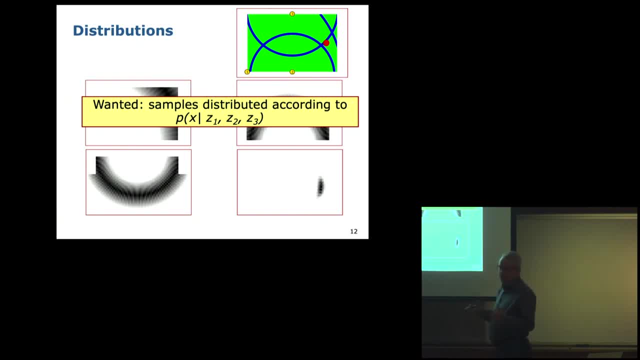 hardly tractable, And so we are actually interested in just using particles and just evaluating those likelihood functions, And this is that what we are, that we want to have. So the idea is is now to basically generate a set of particles from one observation. 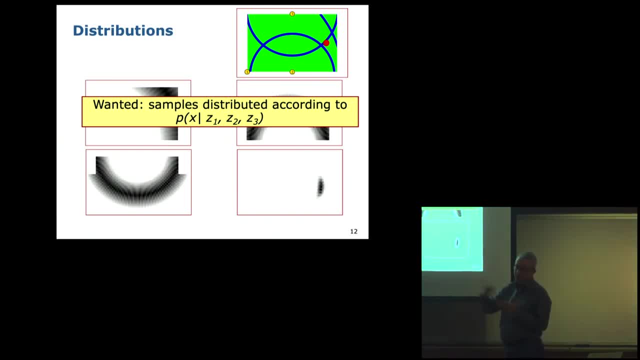 and then this is our proposal distribution and then using the others, like the multiplication of the other two, as the target distribution of all the three as a target distribution, and then get the other two and then basically divide those the resulting, like the importance, weight. 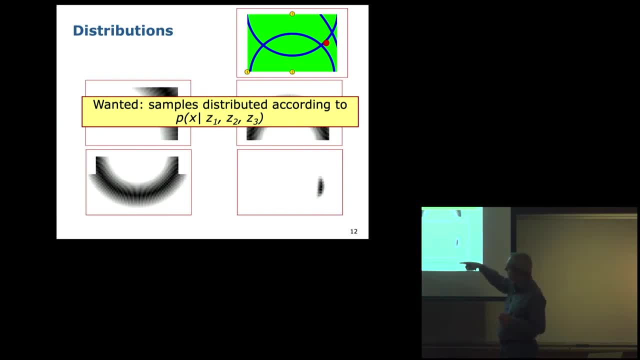 of the first ones, which is uniform by the, or have the importance weights set to the likelihood of those two observations. It's basically that what we are doing, So mathematically. we'll see this in a second so we can sample from each of those. 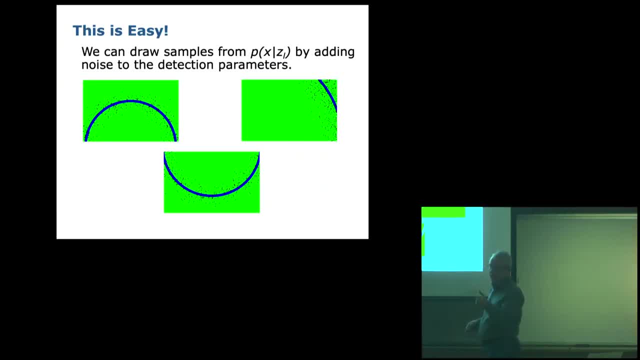 and let's assume we sample from one and what we were now interested in calculating importance weights. let's assume we sample from the left-hand side one first and then we calculate importance weights for those hypotheses over there based on those two distributions. 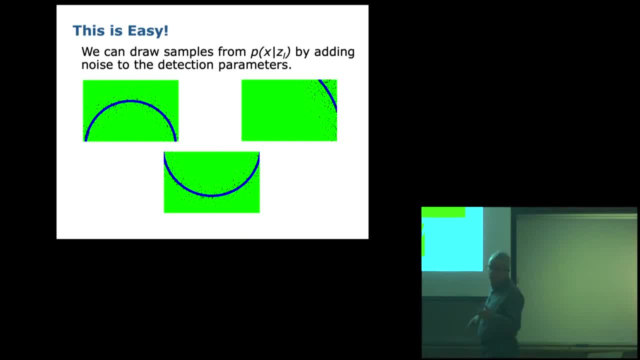 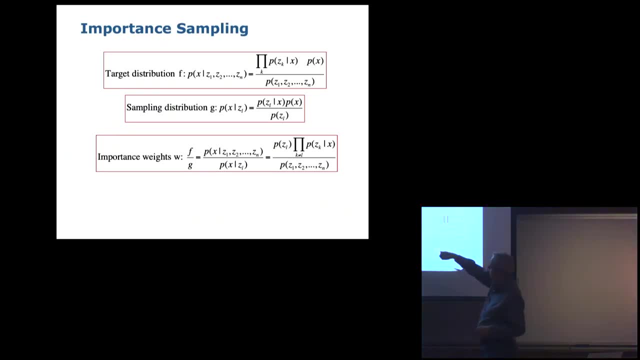 But because of symmetry we can use any of the three and then calculate the importance weights based on the other two. Mathematically, we are interested in a target distribution about where the vehicle might be given all three observations. We do have a sampling distribution. 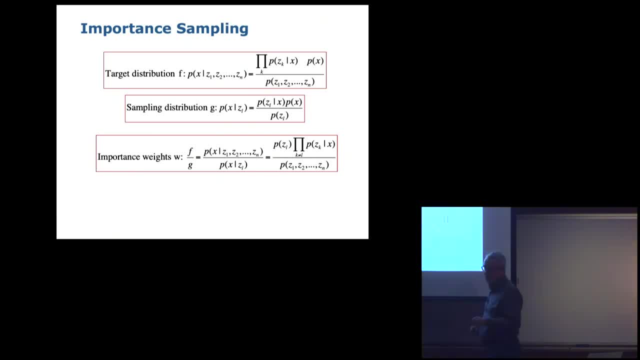 We sample, create samples from one observation, for example, this rejection, sampling principle- and then, in order to calculate the true distribution, we need to calculate the importance: weights which turn out to be, for instance, which turn out to be the product of the likelihoods. 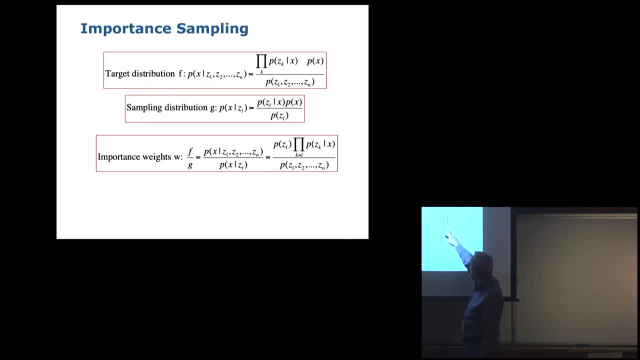 of all the other two, of the all the other observations, apart from the one we sampled from. It's basically, in our case, the other two arcs or arc-like distributions. So, and if you do this right, that would be the weighted samples for all three. 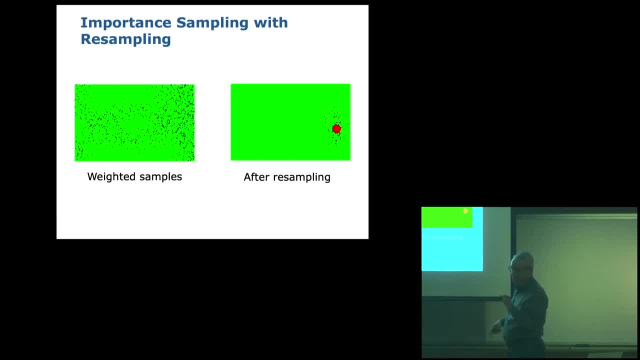 In principle, what we do is we sample from one of the, or we take one of the three and then calculate the importance, weights of the other, and the resulting distribution might then look like this over here. So the key principle is we have kind of like: 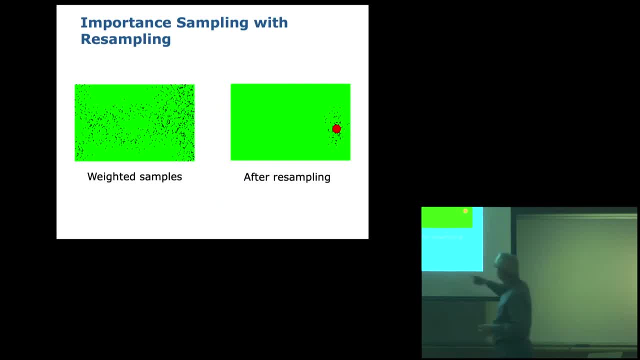 a set of hypotheses and we calculate importance weights for those, and you can now think about the result over here as something like a resulting set of hypotheses generated according to the importance weights. It's kind of like you could think about the result as being a deck of cards. 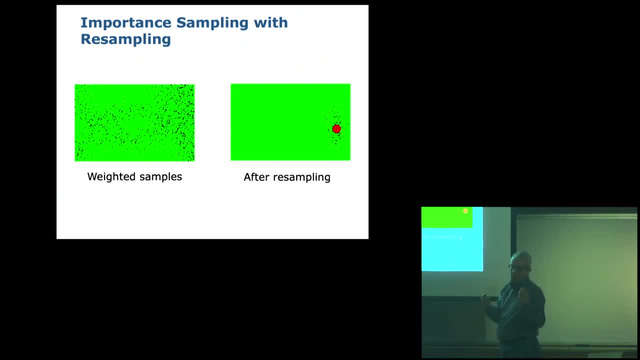 where you actually multiply every card, according to where you actually multiply every card, according to where you actually multiply every card according to its importance weight. So the frequency of a card depends on the importance weight that you have, right. 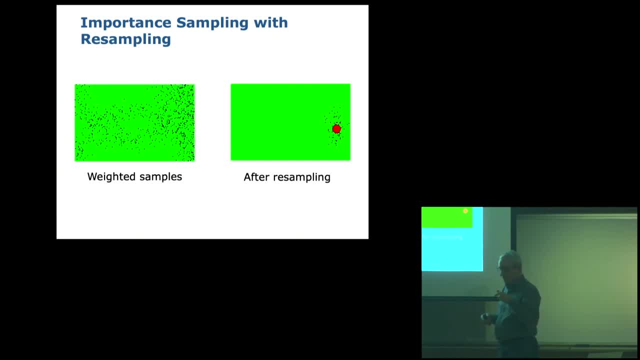 And then when you draw then from that deck of cards with replacement, you put it back in right, You in the end get a distribution that is proportional to these importance weights, And that's gonna be the algorithm that we are basically going to use. 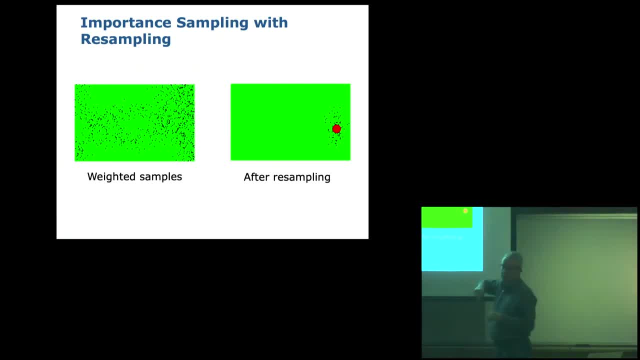 In principle this is how it works, right, And then you get this type of representation in the end. You could also regard of this that you increase the transparency of a particle with or decreasing importance weight, So the lower the importance weight is. 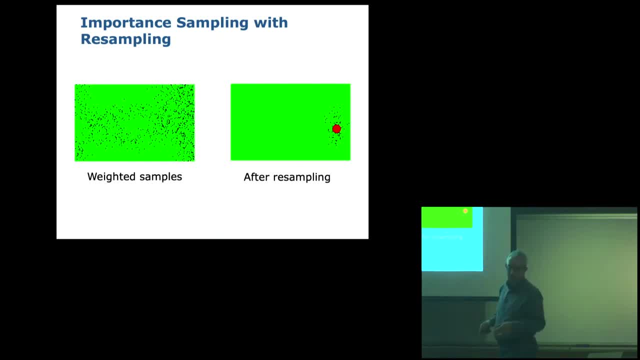 the more transparent it is, and the result would look very, very similar to that one over here. I mean, you don't see semi-transparent particles here, but in principle it's a very same. So how does particle filter localization work? 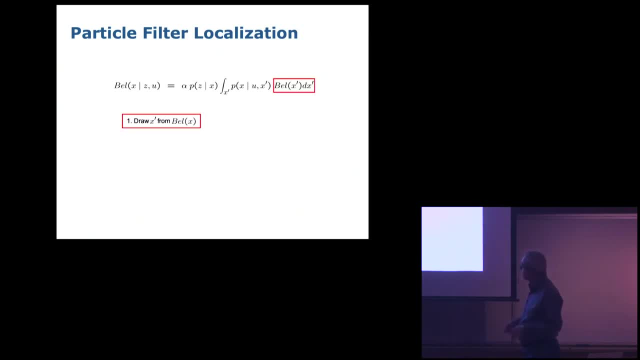 So basically, you represent our belief by a set of hypotheses, right? You take one of these hypotheses out of the hypothesis set, right One of the particles. we draw it from that set, And then comes this step where we actually calculate. 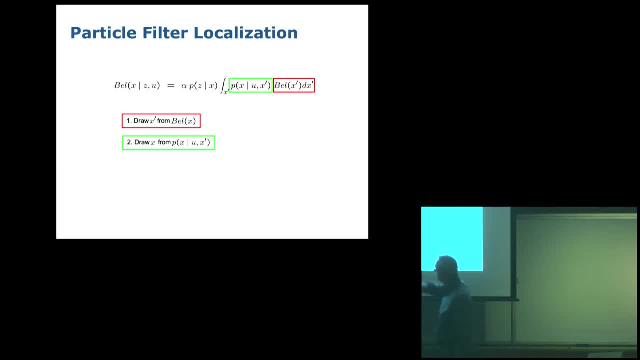 a potentially new place for that particle. Basically we say we propagate it through the motion model, Like X. prime is the one that we get from this, this big current belief, one of the particles in the particle set right. We like sample, a new, like potential place for that. 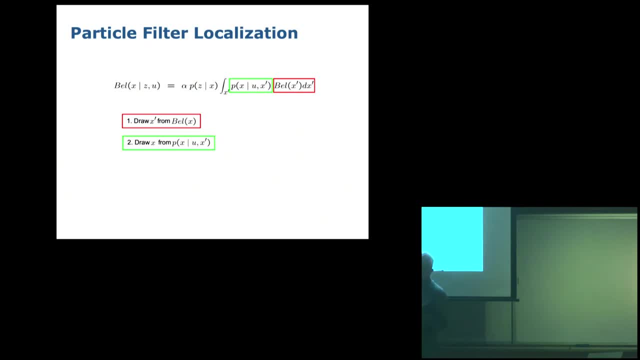 that particle or state for that particle In robot localization. it would be a hypothesis where the robot might be given the motion that it executed. So this is something that we basically we draw that according to that distribution. Next one is we calculate the importance weight. 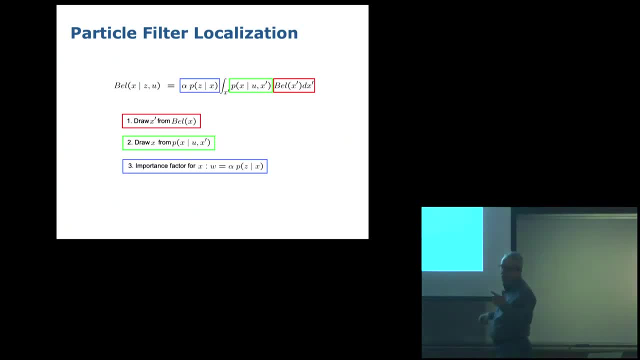 based on the observation likelihood. We look into our camera or whatever sensor we have and calculate what is the likelihood of that observation. given that state that we just calculated, All right, So that gives our importance weight And the next step is that we perform. 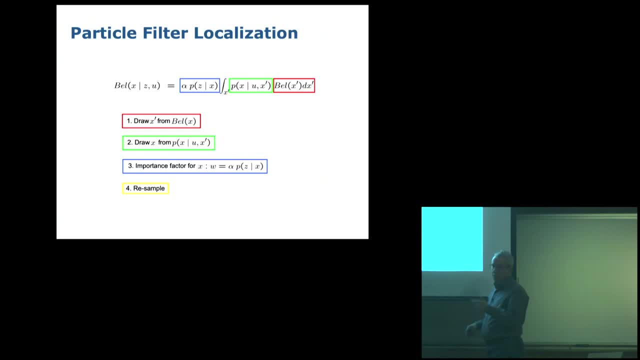 and this is why we call this the survival of the fittest operation. We resample from that set- and we will later discuss how that works- exactly this deck of cards principle: a deck of cards, and from that, and we get a new belief there. 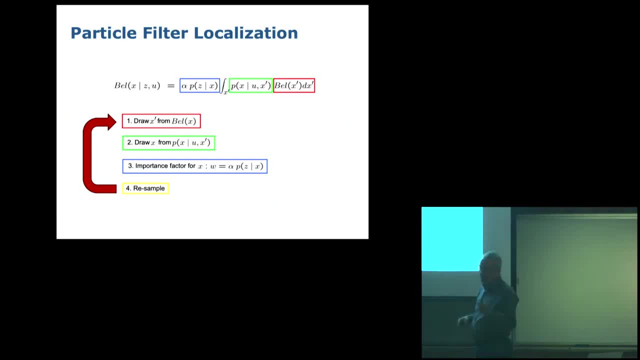 And we basically repeat this process right as long as we actually get updates from odometry or movements or sensor Or perceptions right. This is how it works And in practice, and that's what we are going to do now. 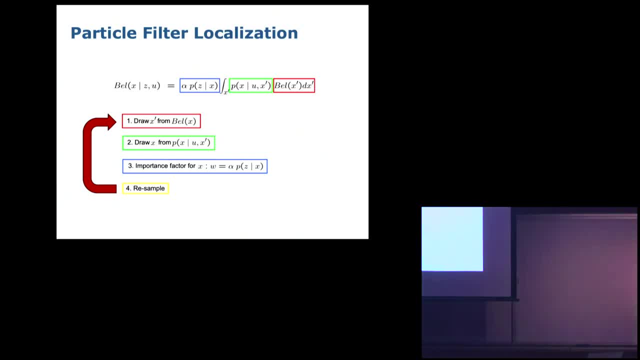 in this, in the next figure. this operation- because it's actually here we draw from the current belief, which in principle is a weighted set of particles, and there's a resampling operation- transforms this weighted set of particles into another weighted set of particles. 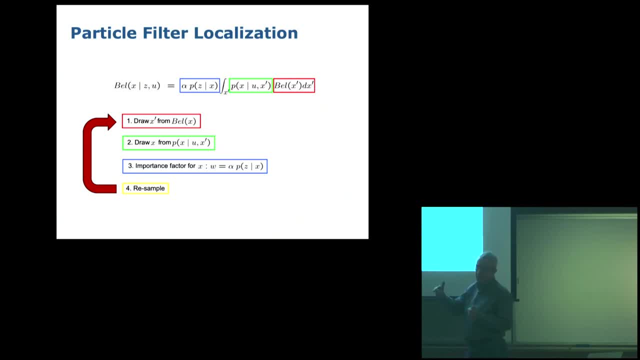 where the particles represent the very same distribution, where the particles represent the very same distribution, where the particles represent the very same distribution as the ones that we have already, however with uniform importance weights. So usually what happens is we get towers of different heights and this resampling operation. 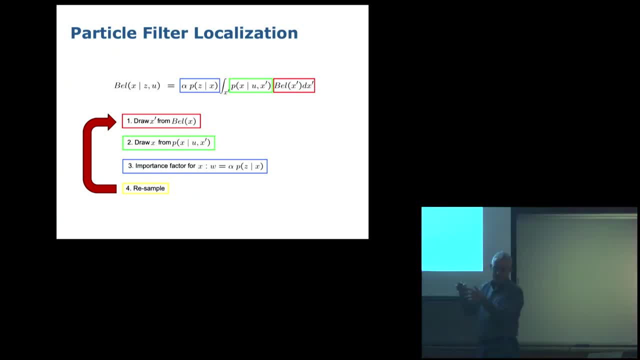 calculates new towers that all have the same height but represent the very same distribution. So that is what is happening. because we have to draw here and there. we basically perform that in one step. It's basically like in the visualization that you see. in a second it happens like this: 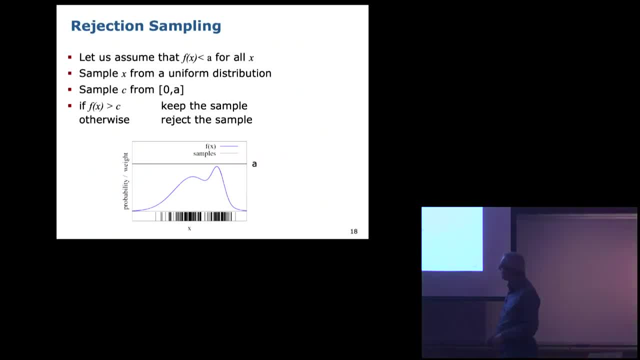 It happens like as one operation Coming back, like to that figure that we saw. sorry I forgot to remove that animation here, but in principle this is exactly like where we need this particular operation. Once we have this distribution, let's assume we hired an undergrad. 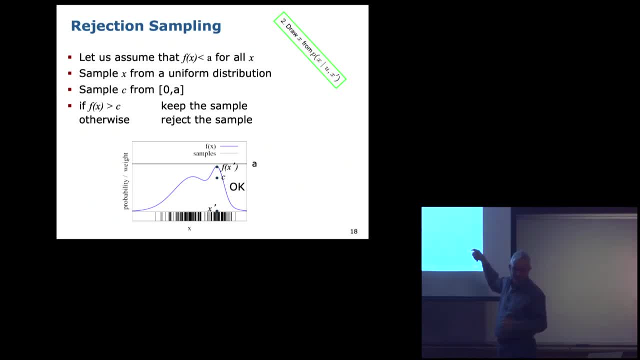 for coming up with this distribution over here and we use this scheme to actually sample from this. It's basically he gives us that distribution, that function, the implementation of that function, and we use this algorithm over here to calculate potentially new places for every hypothesis. 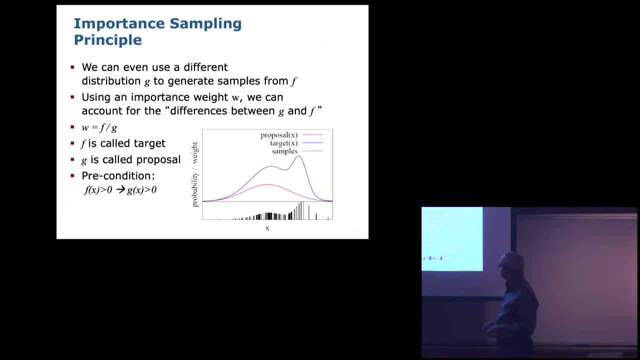 This is a scheme that we're using for that, And then you basically you need another undergrad to implement that observation likelihood model, and once we have that, we can calculate the importance, weights, And that's all you need to do. You plug this into your computer. 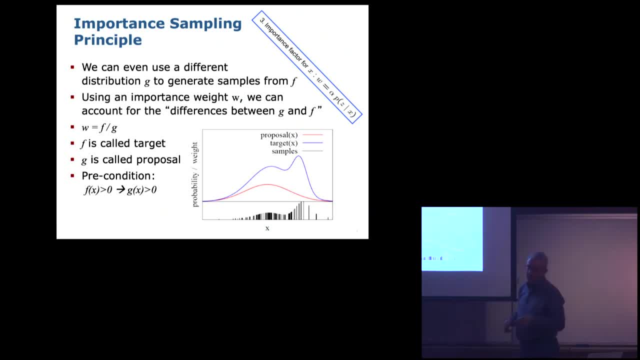 or into your particle filter algorithm and you can calculate the importance, weights, And that's all you need to do. You plug this into your computer or into your particle filter algorithm and then, from there on, you can actually estimate the position of the vehicle. 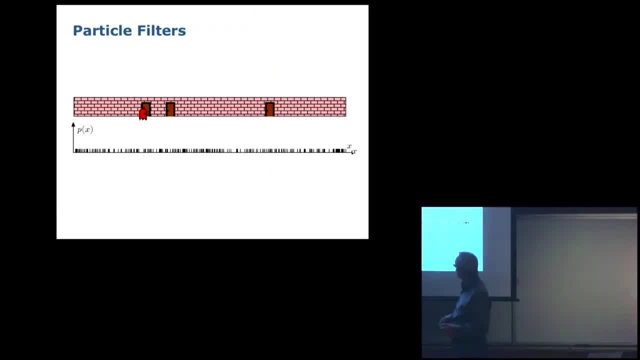 in the real world, Let it be a car or your robot at home, whatsoever. Here's another visualization. We saw this with the distribution, and here's the very same visualization with particles. Initially these are just randomly distributed particles. Doesn't matter if you use them. 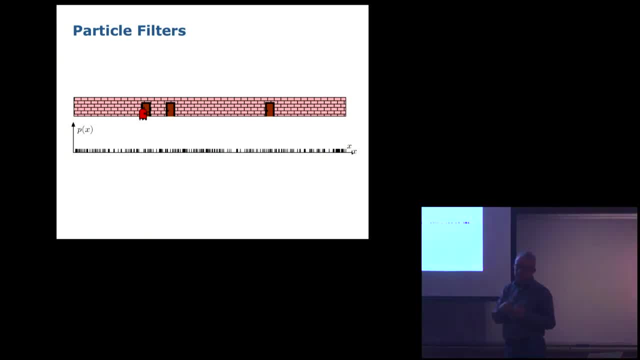 like if you calculate the uniform distribution by just going towards sampling or if you just use your random number generator in your computer for doing that. This is the second version. So the next step is like: let's assume again we have the observation first. 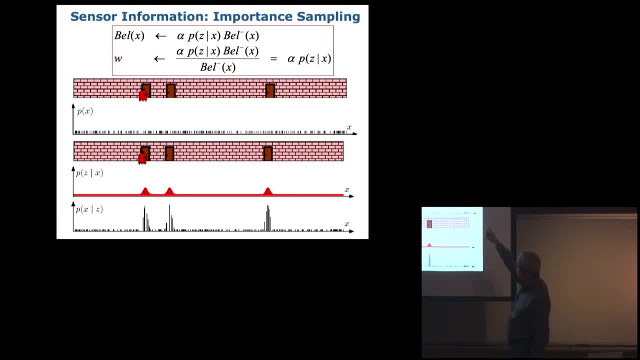 We calculate the importance, weight as just the observation likelihood, given that observation and the state of that particle or hypothesis, right? So that's basically this is our observation likelihood once again, and then in the end we get the observation likelihood. 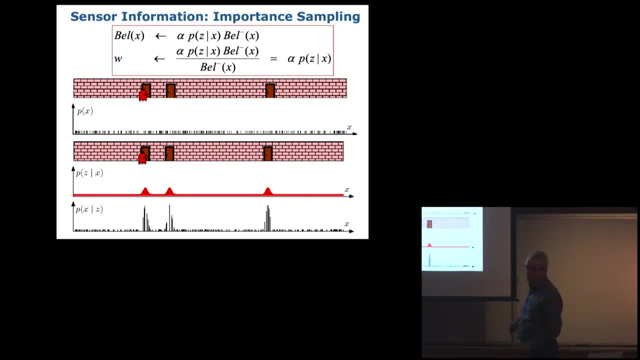 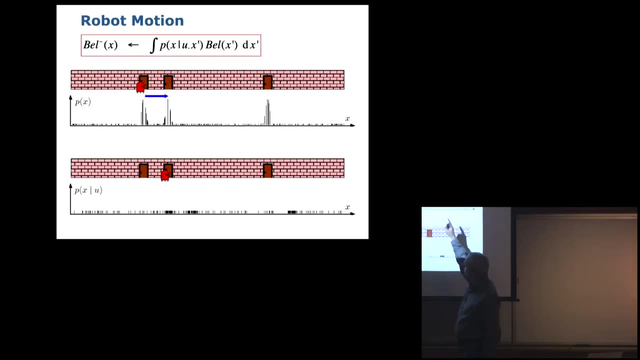 We get these towers with a height proportional to the observation likelihood, right. This is just because we normalized the weights so that they sum up to one overall hypothesis, right. And now the next step is that the robot moves, and in that step we actually need to pass the hypothesis. 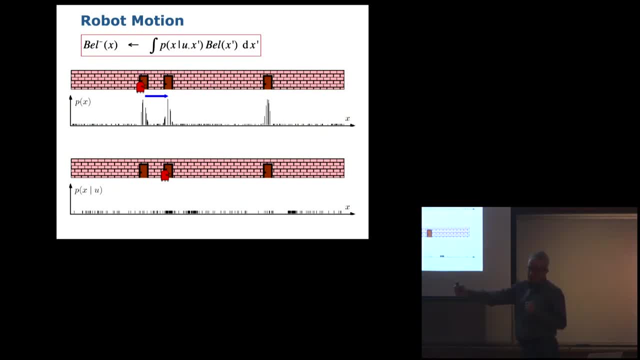 to that motion model. so we sample new potential states from that and at the very same time we perform the resampling operation, this magic thing that the robot converts weighted particles into a set of particles with equal weights that represent the very same distribution idea. 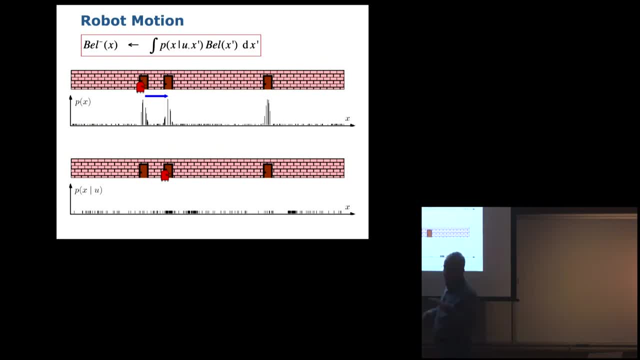 or an approximation, another approximation of that distribution with uniformly weighted particles. You will see how that algorithm works in a few seconds. So what happens now is the robot moves forward and we propagate the particles through that motion model and at the same time resample, in a way. 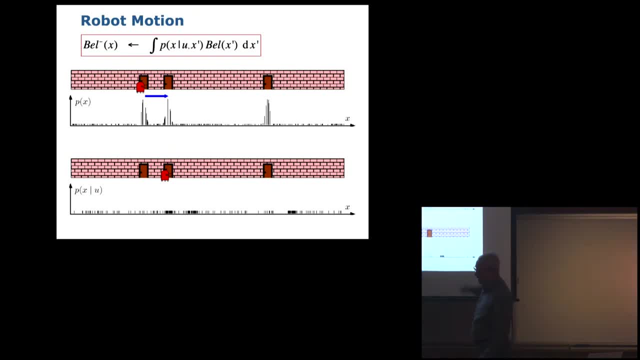 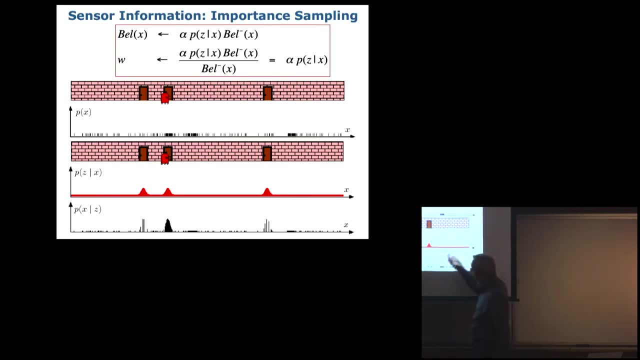 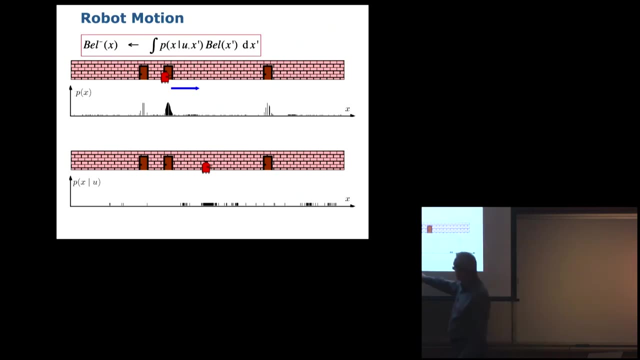 like with this deck of cards, we can now go back to the original operation and get particles, higher possibilities, distributed like this over here, right And again, like if you have another observation, like we weigh these particles, like another movement, and then you see that these particles typically cluster. 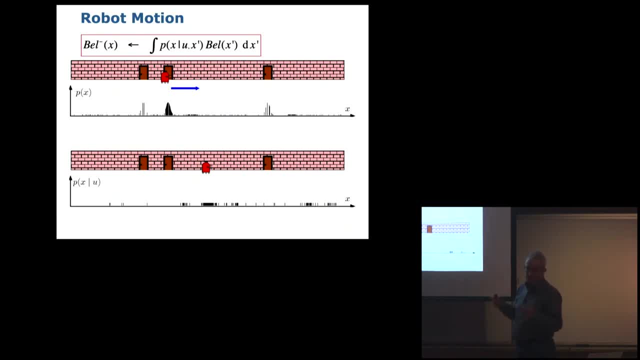 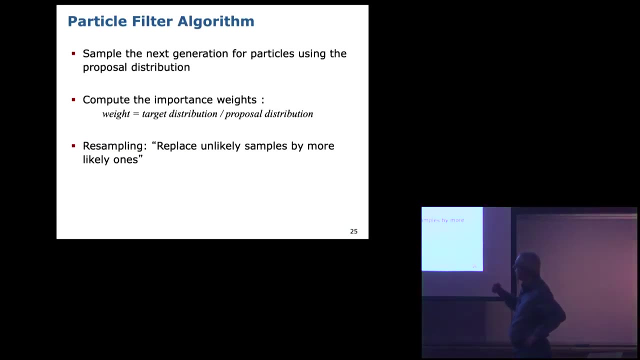 in places that are consistent with movements and observations, and as our observations were consistent with the real world, we do have a distribution. the true state is. so the particle filter algorithm is basically nothing else but then a procedure that, like, uses particles for representing the belief or hypotheses- weighted particles and the 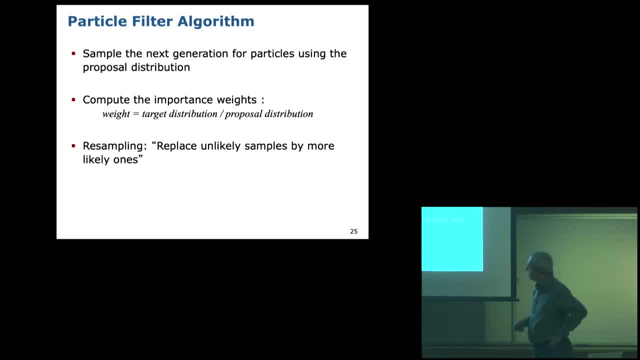 weight is the target distribution divided by a proposal. distribution that is, in the context of localization, is nothing else but for one observation: the observation likelihood of the latest measurement, given the state of the particle and the resampling operation. this magic thing that we only implicitly talked about thus far is the operation that replaces 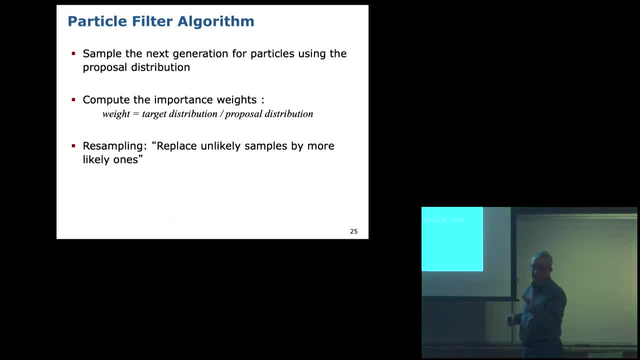 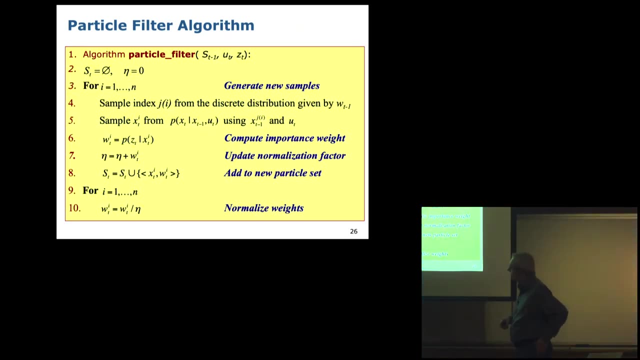 a particle set containing unlikely state hypotheses with likely ones, basically by drawing more likely cards from that deck of cards. and this is the algorithm over here. so you basically like, at the very first step is like that we perform this resampling operation like this: basically we sample from the current distance, from the current set of weighted 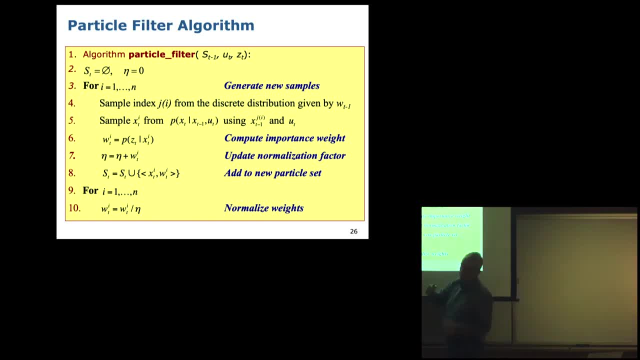 particles, like a number, which is basically index of a particle, and we draw that particle with the probability that is proportional to that importance. weight meaning: higher particles with higher weights are drawn more often than others. right, this is this index j that we calculate. we then take xj right, which is like xt. we calculate xt from the previous. 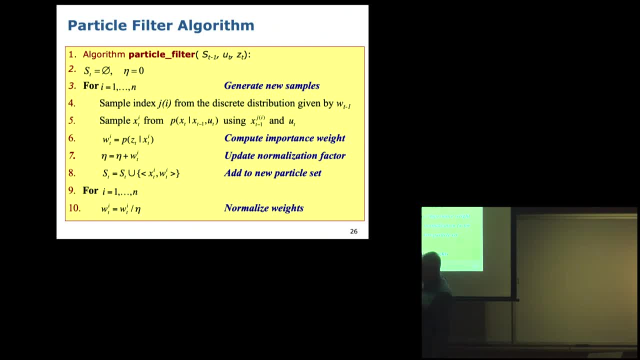 one that we draw from that particle set, passing it through that motion model. with the rejection sampling principle. we calculate the importance of weight, which is proportional to the observation likelihood. we normalize the importance of weights right, that's why we calculate this. we sum all the importance weights up and add this new particle to the particle, to the new particle set. 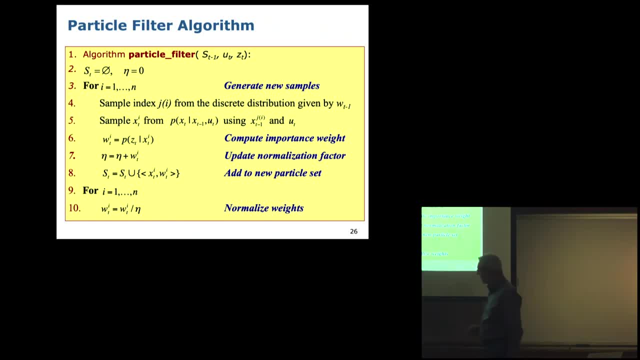 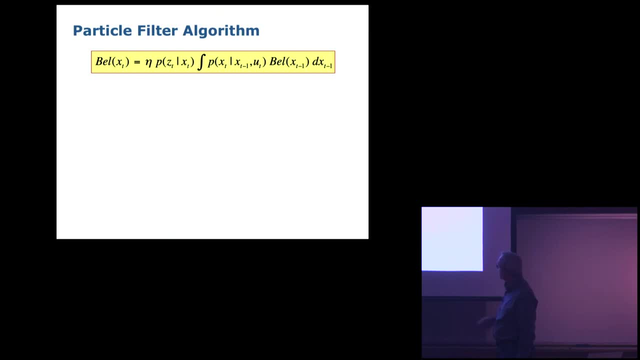 right, this is the normalization operation down here. it's basically that. what we are doing- just to- to sum this up here, I call this works- is like: in the first place, what we are doing is we draw a particle from that existing set of particles, right, we pass it through that motion model. we say: 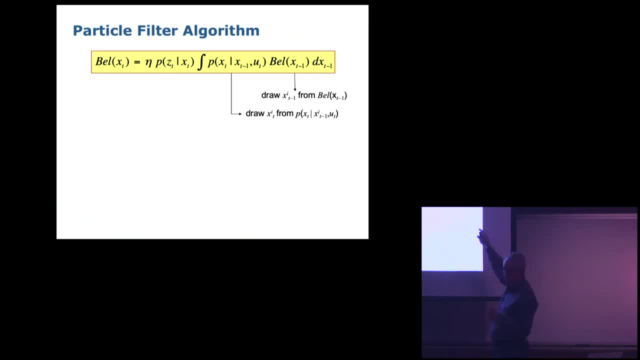 draw a new pose according to the pose of that particle and the action carried out by the robot, we get a new state or pose of the vehicle. then we calculate the importance vector or vector, which is like: if you do the math exactly, then it turns out to be just the. the observation likelihood of your measurement is that. 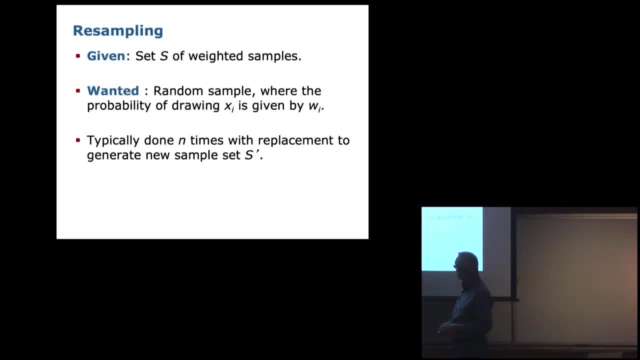 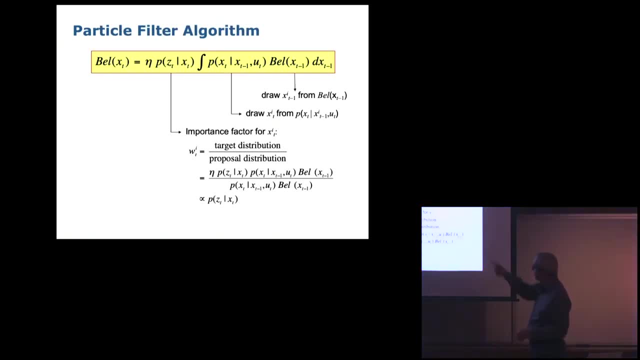 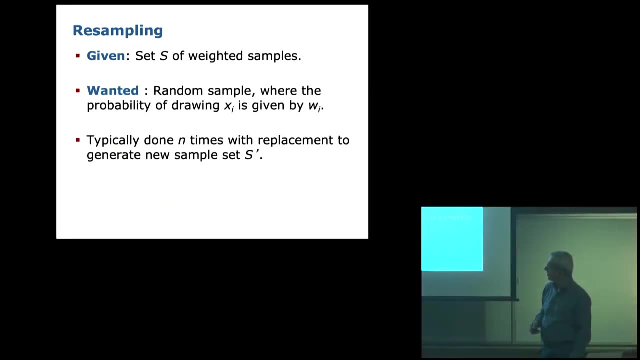 he given that state of the particle, and that gives you the sorry hey, that gives you the new set of the new belief. and let me see. the next is the resampling operation, and I was told that we're going to do a short break in between five minutes, seven. I do over always seven minutes in Freiburg, which is like 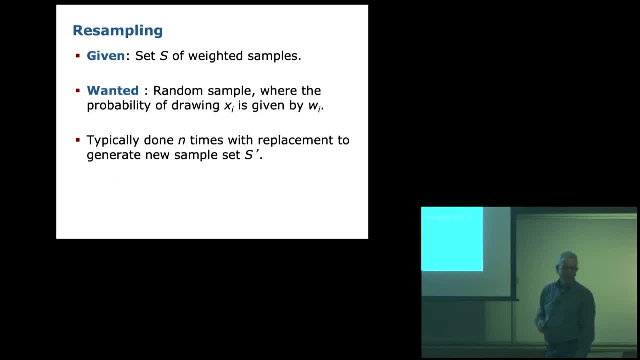 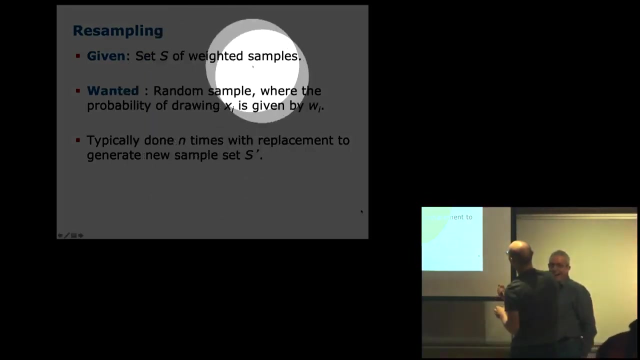 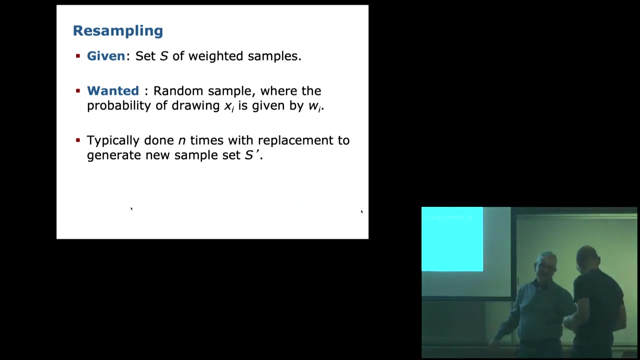 getting to the bathroom and back and all the operations in between you. seven minutes. okay, let's do 12 at that. according to that clock, 57 to according to mine. you know what the advantage is. you do not need to point at the screen as well. yeah, and there's. you know, to often you have these presentations when you have a. 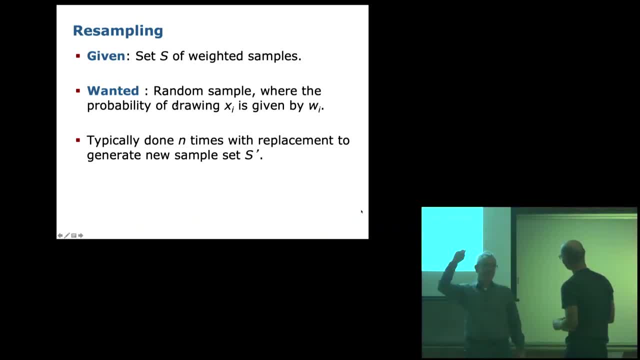 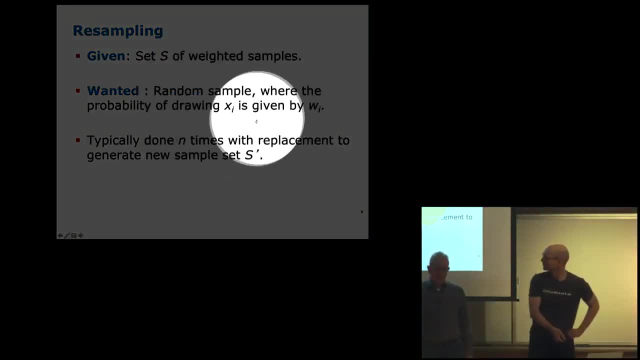 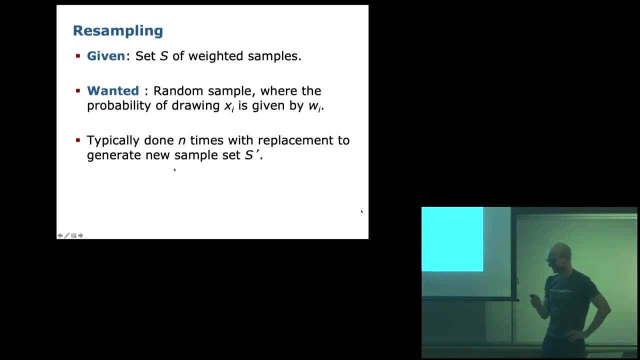 big screen in front of you. then you can stand there and point there, otherwise you have to turn around, Point here. Yeah, Wow, if anyone wants to try it, it's pretty cool, but you can program it. it also has like a red dot, if you want it. this guy. 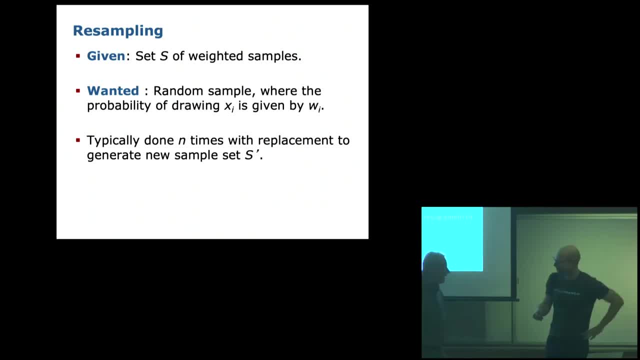 mamming operation is to, So you need to have something bright to calibrate on it. No, it's just like a lot more complicated. No, it's just like a lot more complicated. like an IMU, it is just like it. I think it initializes at the last position and 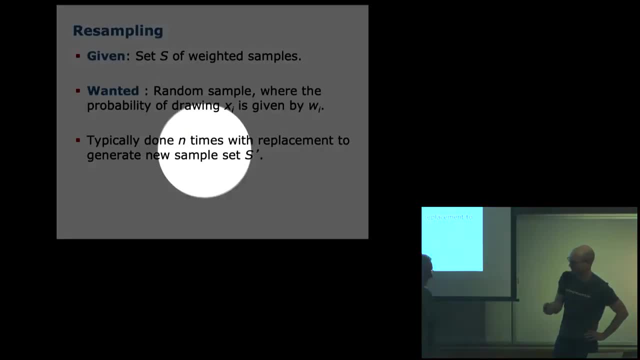 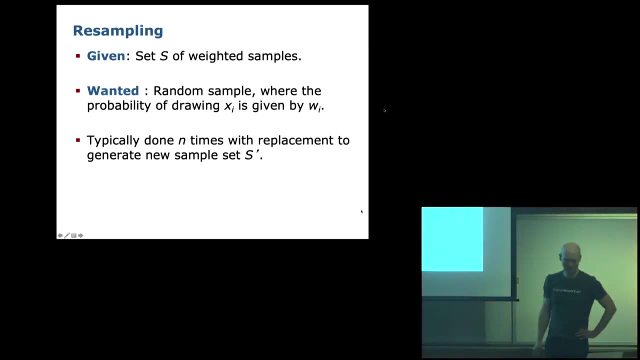 then it takes your movement to see when you put them. I click this way. yeah, it is important because it is directly done on the graphics. I see it's just wherever you start is the middle of my screen or some part of the scan. so the only problem is then you have this presentation mode. position would mean I 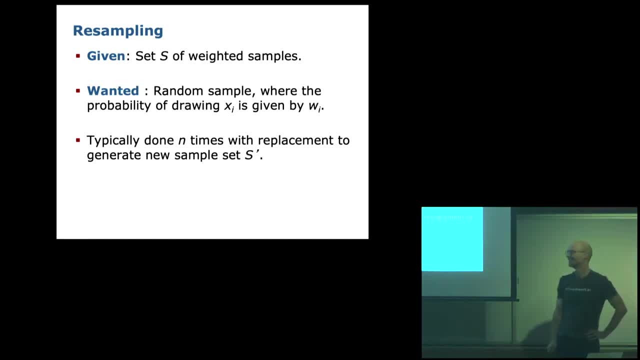 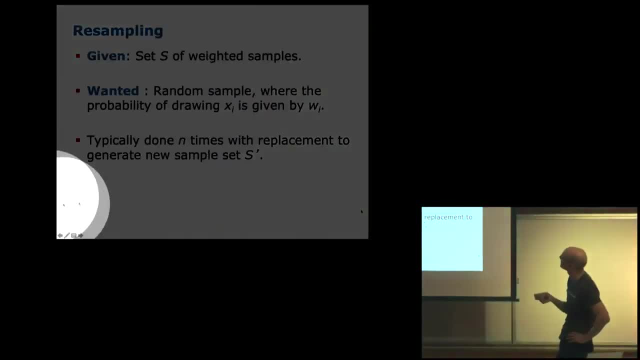 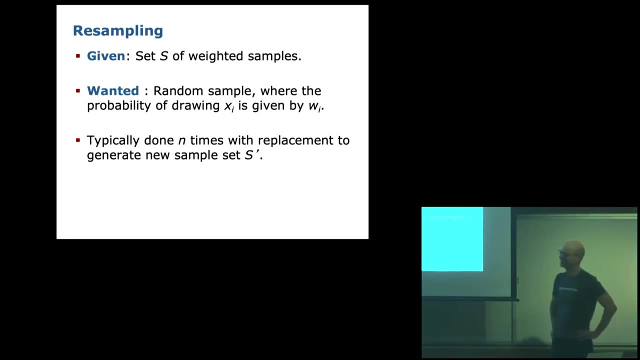 now cannot see my next slide, which is like: I think it is also possible doing that, but it's my third presentation I'm giving, but it's pretty cool, so why? particularly when you recall things and you do it, then it's actually also in there, otherwise, when you could point it. oh, so the yeah, because it is recorded it. 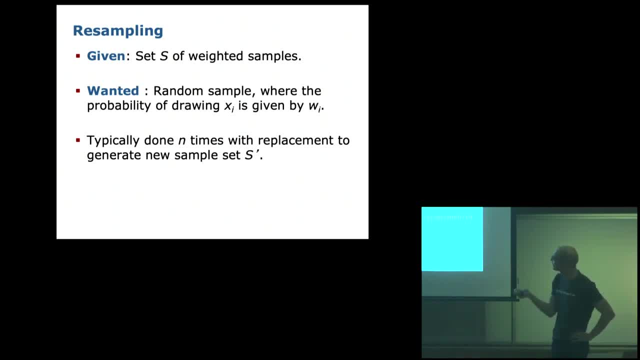 is recorded through here directly. yeah, so whenever people watching it on the video see it too. oh Yeah, I bought one for my lab as well and it disappeared. You need to buy 40, I guess. What is it called Logitech? No, Logitech. 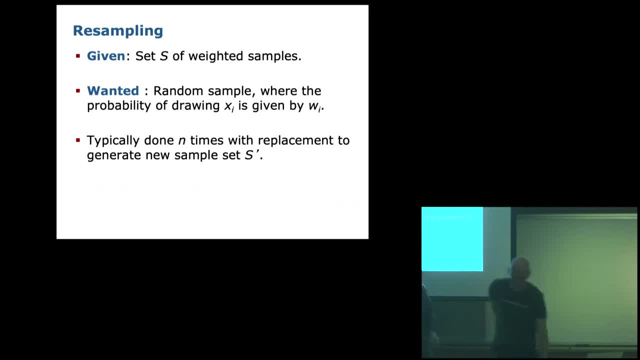 Logitech: All right, Next lecture, But it doesn't work well with Hangout. when you do these Google slides, You got a minute. Yeah, Yeah, I think I found one I have been thinking about. 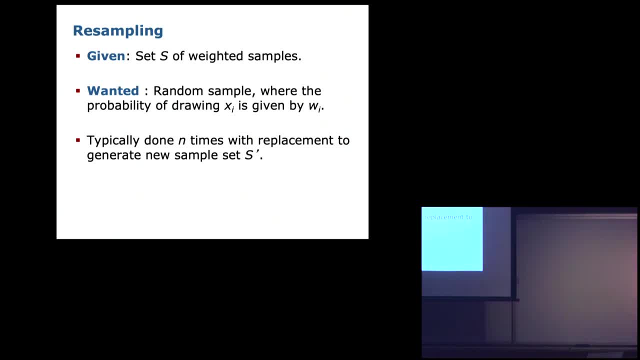 So I'm more thinking about you. know we use the same methodology but apply it to like knowing of the optimization, so that we have a better form. 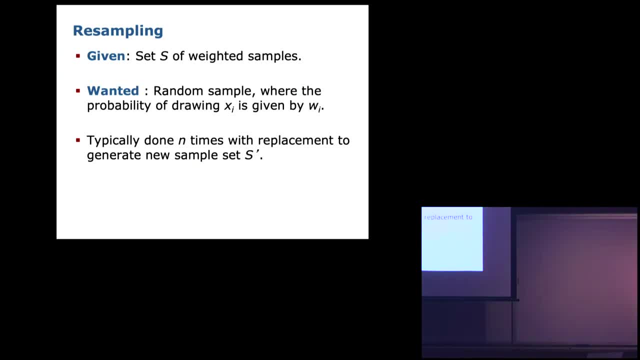 Yeah, It should definitely be possible. Okay, Right, Because in that paper I don't think there's any claim to like how the environment was carried out. You know- And I'm thinking because we have a car ourselves- 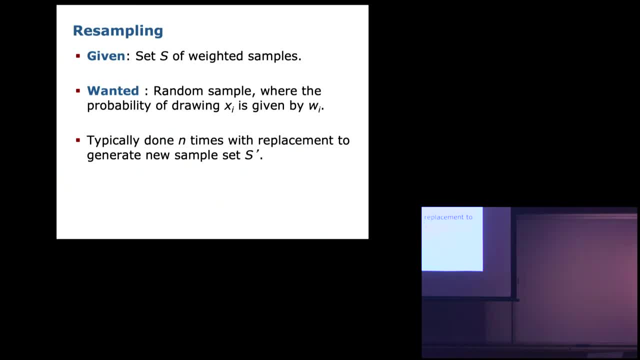 And we have some. So what about this into say like 20 seconds each? So I run a small for 20 seconds And I compare with my, And then whatever RPK I have And then see like my reward will go. 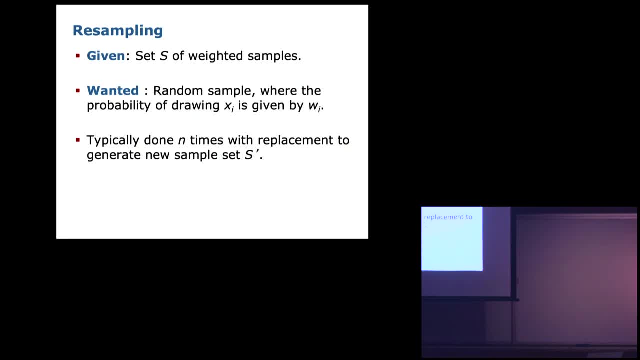 And then it actively removes the All right. So Because for the 285, the proposal came out, But for this course I think the proposal should go out for like a week. Yeah, Thank you so much, And I see you were. 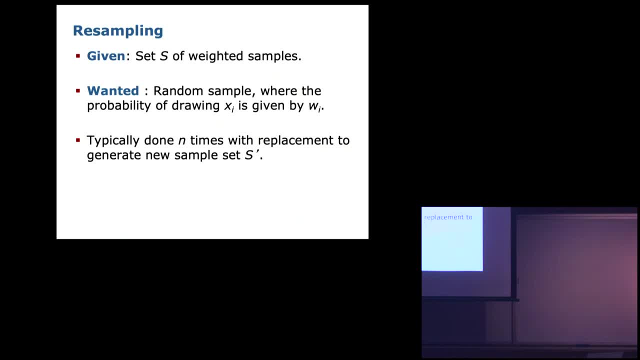 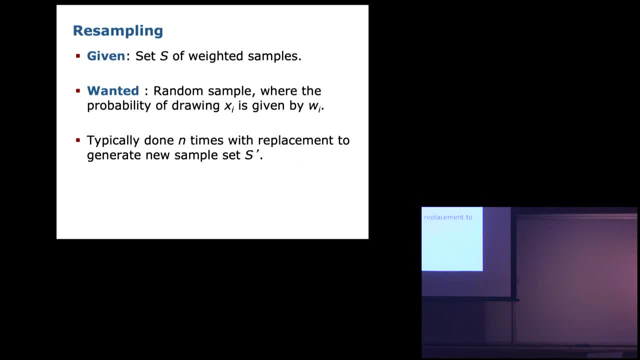 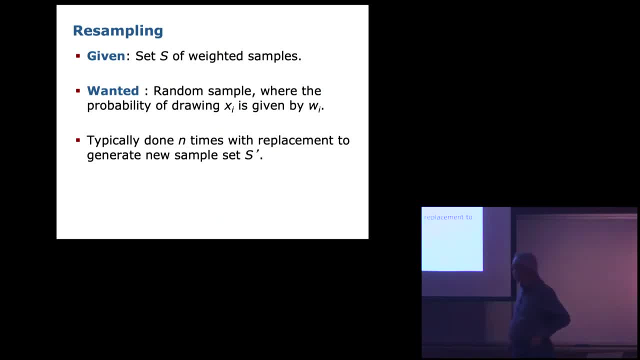 57. Way to go. We're German and start on time. Not really, Not really Good. The Swiss would really start on time. Okay, So that operation that we haven't talked about in detail is a resampling operation, and this algorithm is also actually. 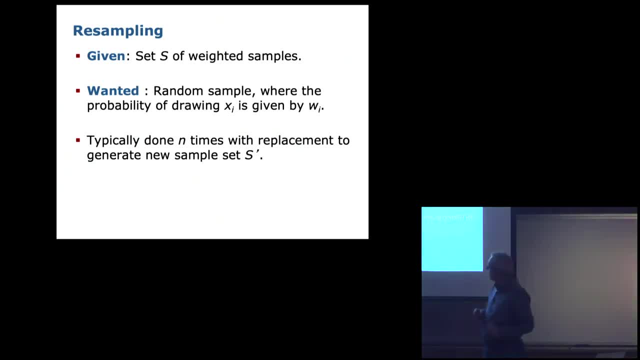 pretty cool and how this is done. We're going to talk about two variants of that, and the first one is a rather naive one, and the second- the second one- is a little bit more fancy, and then we will talk about the difference or the properties of those. 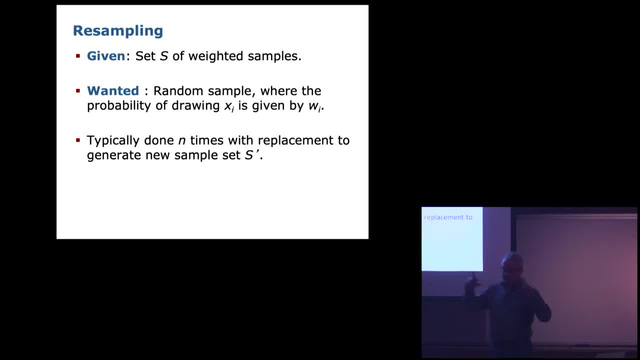 So what we typically have is we do have a set of weighted particles with uneven importance weights, and what we want to have is typically a set of particles that is distributed according to this weighted particle set, with the importance weights that are uniform, And the reason why this is so important is that 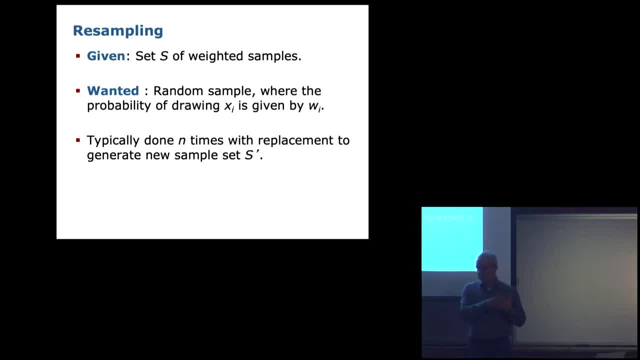 The reason why we want to have this like: assume that we let this algorithm run without this operation, So these particles will basically spread out according to our motion model. We sample from that motion model, So the positions are determined from that sampling operation or the states. 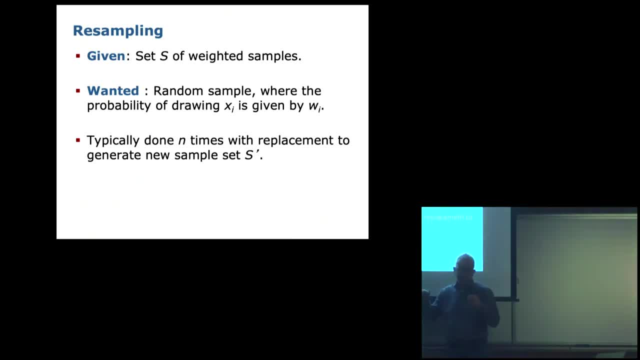 And they all have different importance waves And what happens is typically that some particles get into spaces of this or areas of that configuration space of the system. that is extremely unlikely. So we will have, like, very, very high differences or large differences between the importance waves. 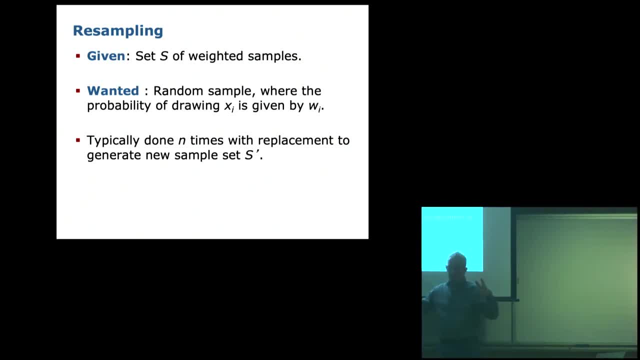 And some particles. basically, if you think about this distribution, are in areas where we have a very, very low likelihood, Which means that they actually do not contribute to the approximation of that distribution. Removing these hypotheses would actually not help us a lot when it comes to like the accuracy of that representation. 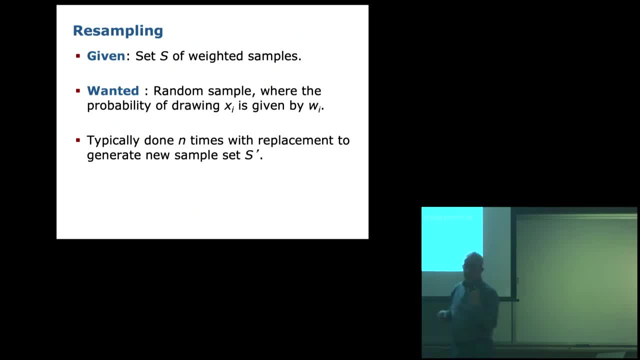 So what we want to have is basically particles that are close to the peaks of that distribution, so that we actually can get more details about how the distribution actually looks like. And this is why we need this resampling operation, And what we do is basically, we take 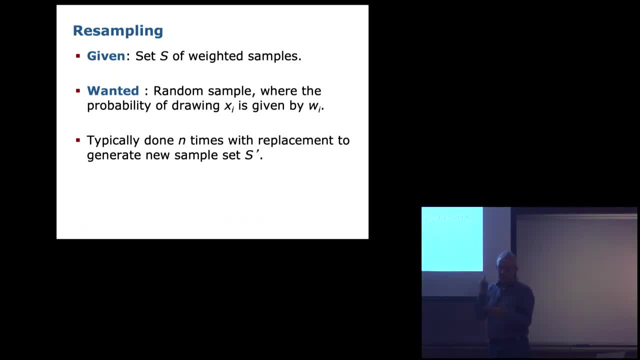 like with these cart, a deck of cards, right, You multiply every like, every particle, according to or proportional to that importance, weight, And that depends solely on the memory that you have and the resolution that you want to have. And then we draw from this deck of cards randomly. 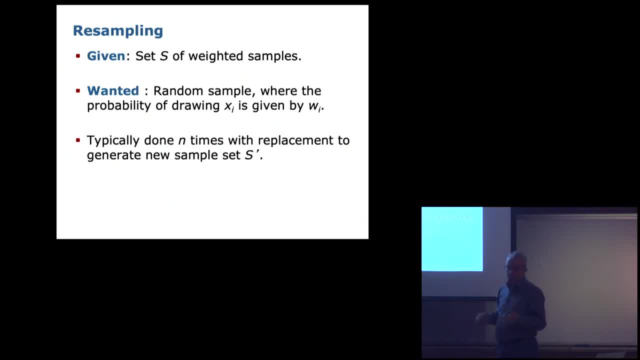 in order to figure out which particles should actually be in the new particle set. This is basically what this operation is about, And like from a more like algorithmic point of view, that is, we are in that in the following regime right. 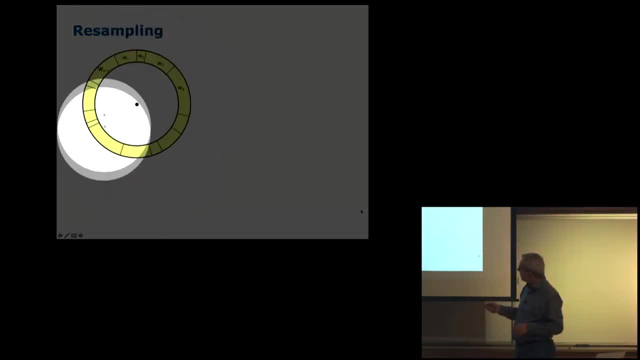 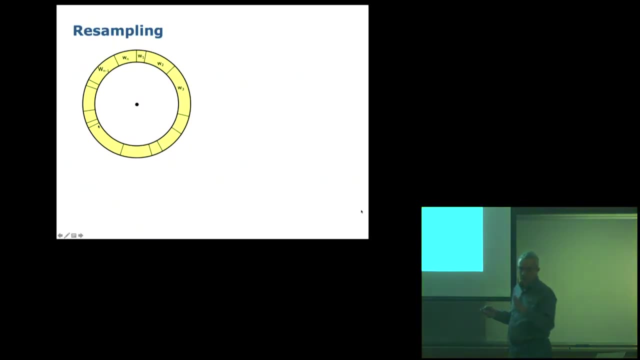 We have like a set of particles right, So W1 to Wn, right, And they. we arrange them now in a circle and you can regard this as a roulette wheel. right Where the holes in that wheel are, their size is proportional to the importance, weight. 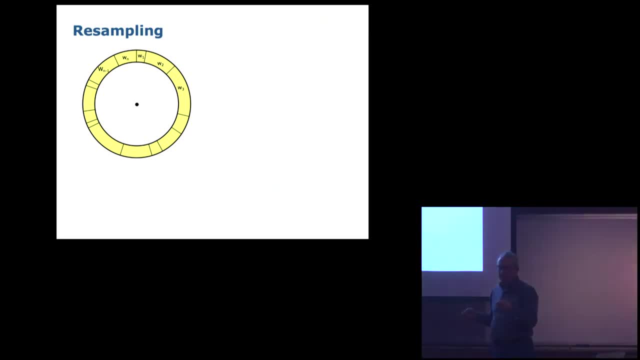 And if you now throw a sphere into that roulette wheel, right, it will end up in these bins with a probability that is proportional to this right. So that's what we do. This is the importance. weights Under the assumption. yeah. 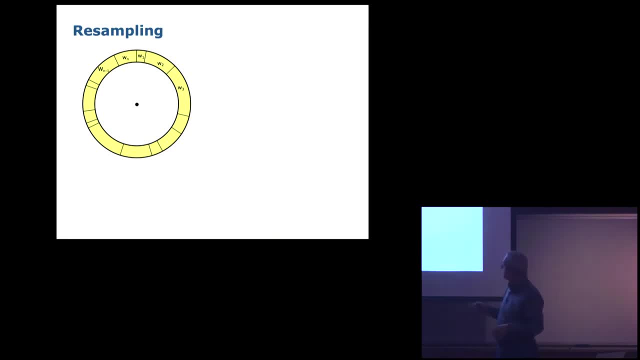 or exactly the importance weights when they sum up to one, Which basically means, mathematically, what we do is we just draw an angle right, Like this one over here, And then we need to calculate the bin in which that angle falls right. 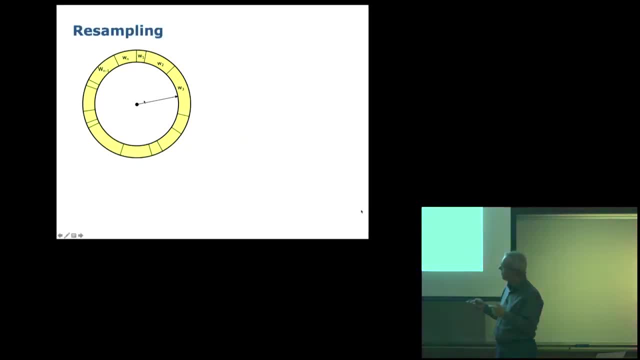 So in this case it would be the bin three right For particle three would be taken Basically just you draw a card from that deck and then it's basically the number of cards- equal cards- in that deck is the size of that bin, you know. 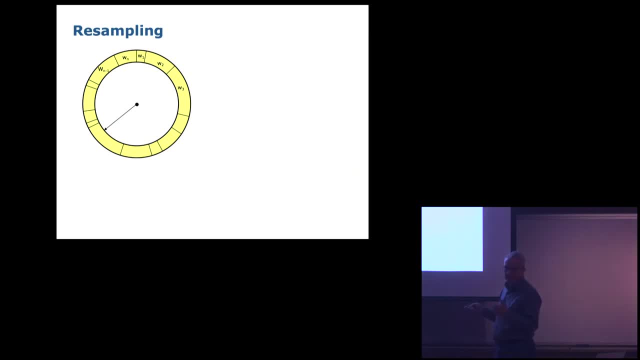 And so we repeat this N times, and by doing so we get like N new particles right. So the operations that we need to do is like drawing an angle, or if you arrange them in an array, right All these particles, you actually wanna draw a number. 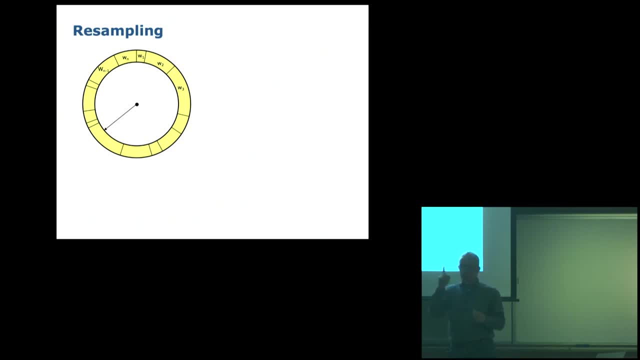 between zero and one and you wanna know which particle is that, into which bin this number falls right. The question is: how expensive is that operation, If you do wanna implement that right, Drawing an angle, figuring out which bin is it? 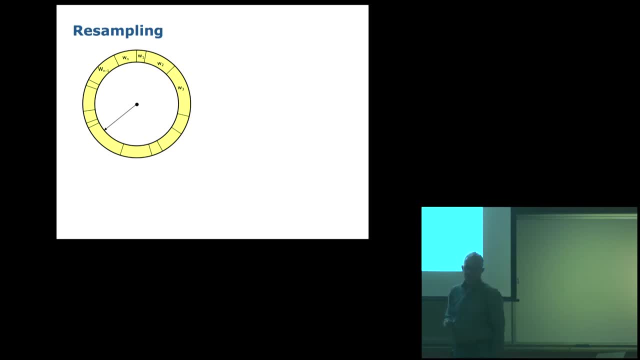 What is the cost of that operation? For just that, the search is the number of particles. If you implement it in an array, you run through that array and check: does it fall into that bin? right, Yeah, So that's the cost of that operation, right? 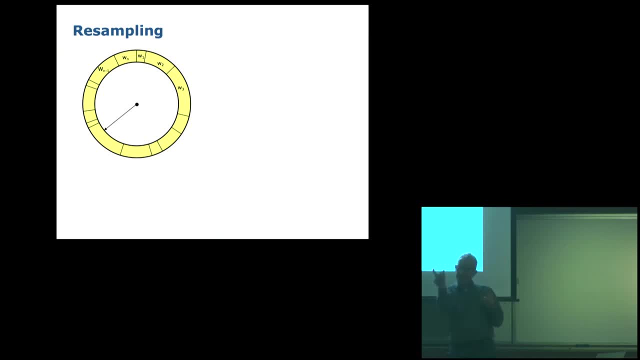 So that's the cost of that operation, right? So that's the cost of that operation, right. Yeah, That was what you. that's great, And you need to do this N times, so it would be N squared. Someone said N squared. 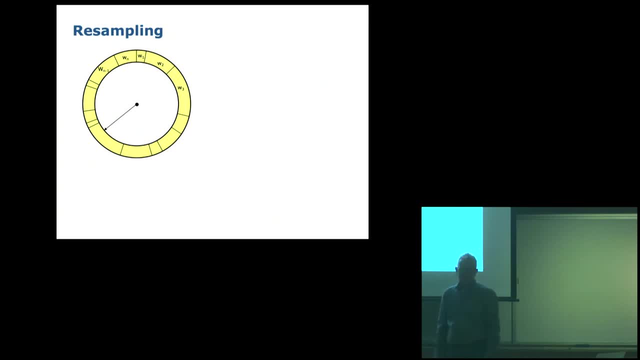 Can you do this more efficiently? So I give you a hint. So imagine we, instead of calculating, looking just at the importance weight, we look at the right borders of the importance weight and their positions, all right, Which basically is an ordered set of numbers, all right. 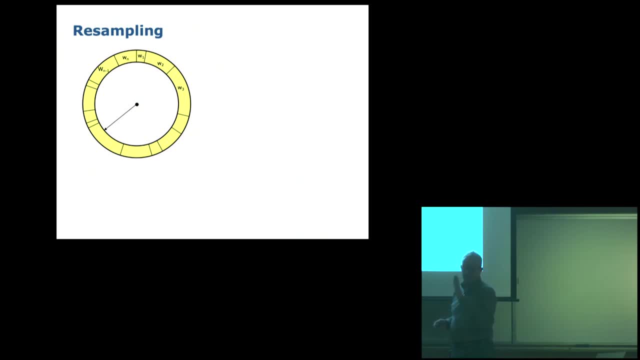 All we need to store in this array is just like where it ends. We get the start from the where it ends of the previous one, right, And if you don't search in such an ordered set, That's log N. That's log N. 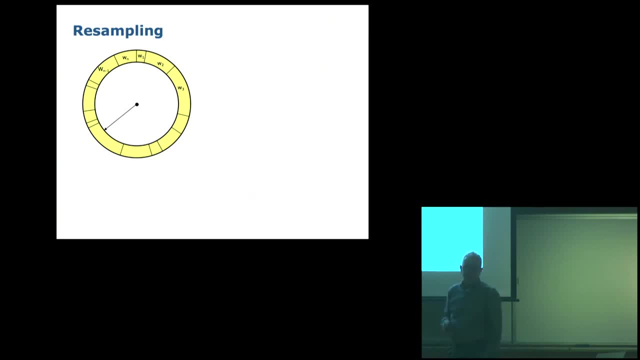 And the procedure is Binary search. Binary search- yeah, So you can do this in log N. Yeah, Which is cool. Log is virtually constant for every number that we can imagine. But on the other hand, if you sit in front of your computer, 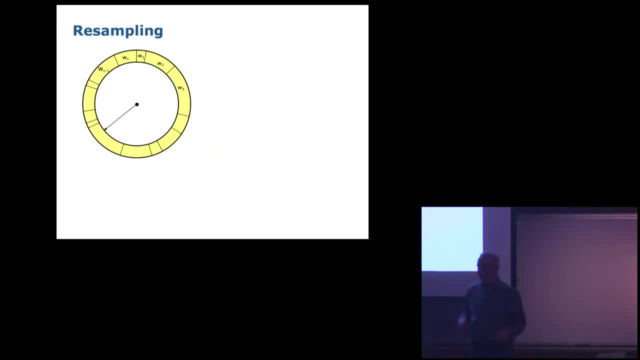 students hate log N because even if it's a 10, it is like a factor of 10 that it takes longer. So that's why people don't like log. So that's basically that procedure. It's a roulette wheel: binary search and log N. 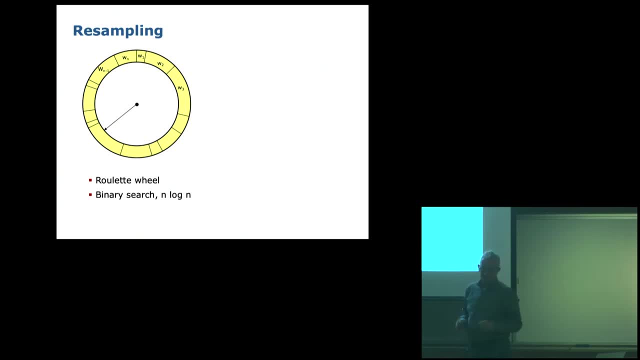 is the operation, But there, interestingly, is a faster version of that, And this version works as follows. So all we need to do is we need to sample one angle between 1 and 1 divided by N, N being the number of particles. 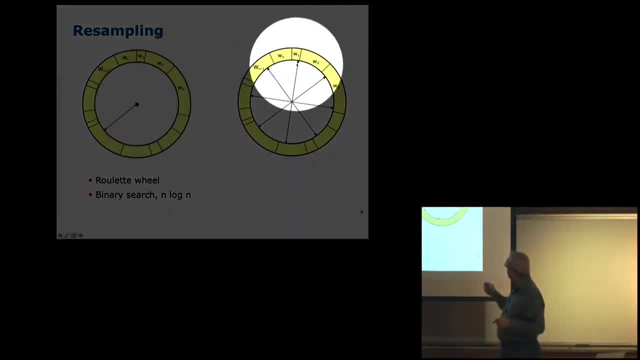 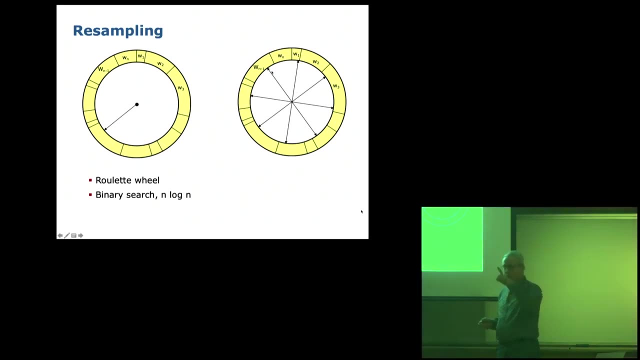 And then we advance in a constant fashion, basically by 1 divided by N, And we do this N times, And wherever every particle like in whose bin we then step, we're doing, that operation is the one that we keep, And my argument is that this operation 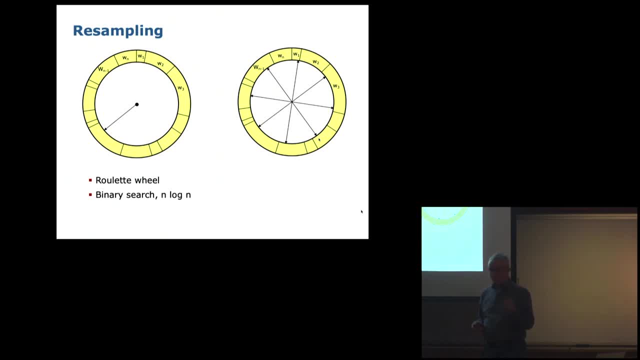 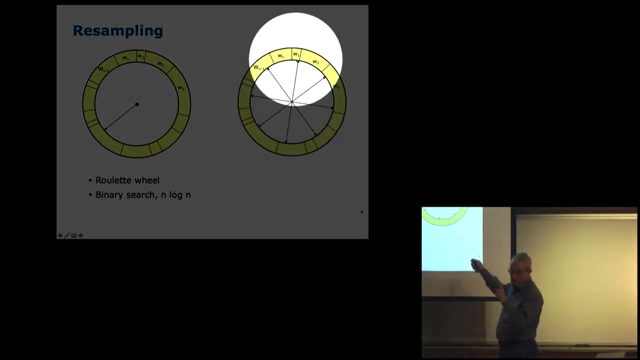 can be done faster than log N per particle. Why is that the case? Could you say that again? Yeah, So we start with. 1 divided by N is the first angle. It's randomly chosen angle between 0 and 1 divided by N. 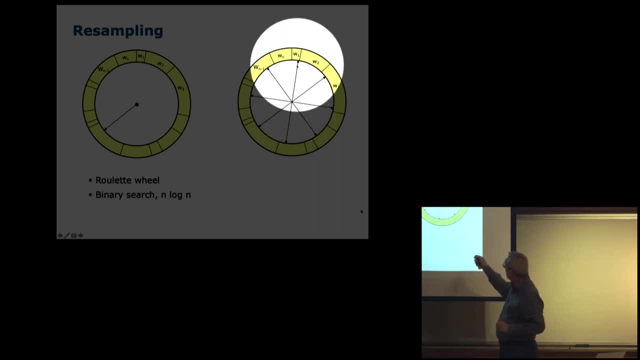 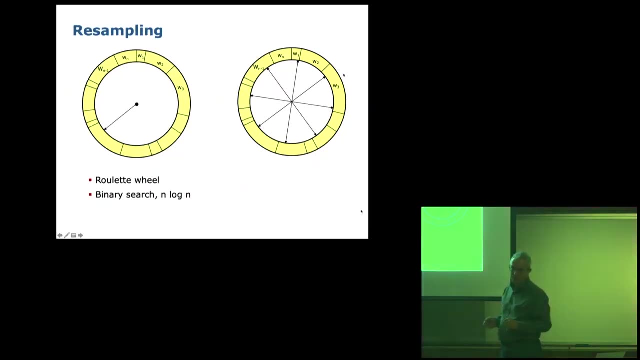 That's this angle over here, like the difference from the vertical. And then we advance by 1 divided by N and check into which particle that falls or which particle's bin that falls. And then we advance by 1 divided by N again. 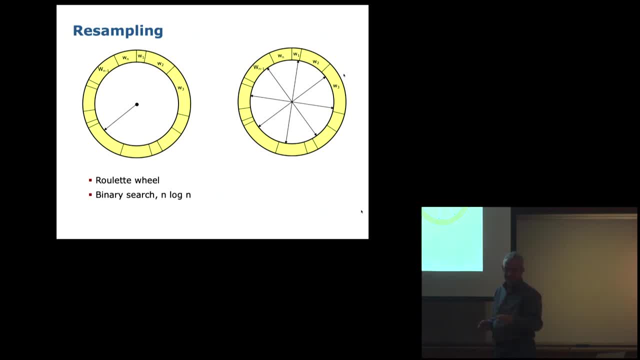 So this time it's just linear total, because you search each of the spokes of the wheel. Yeah, And how often do we need to touch Just once? Yeah, Some are touched twice, but some are skipped, But we never go back. 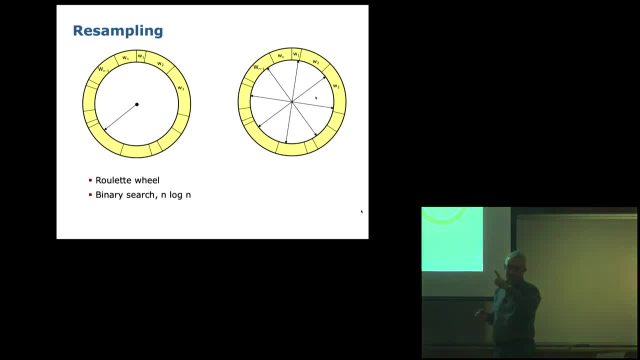 We never go backwards Because we only go forward, And we need to do this N times. we actually end up with an operation that is constant per particle. And this has another advantage, And we will talk about this in a very few seconds. 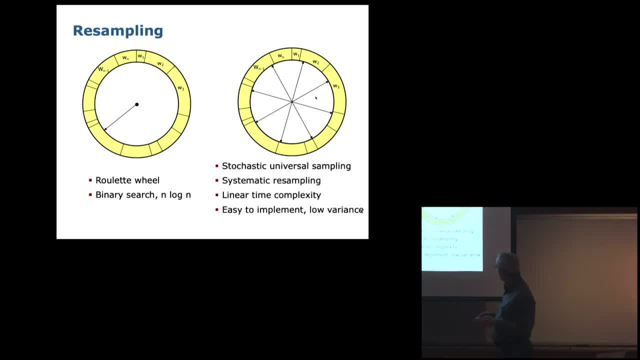 So basically, these are different versions of this, And then this is called stochastic, universal sampling or systematic sampling. It has linear time complexity in the number of particles, Yeah, And that's why professors always tend to say it's easy to implement and has a low variance. 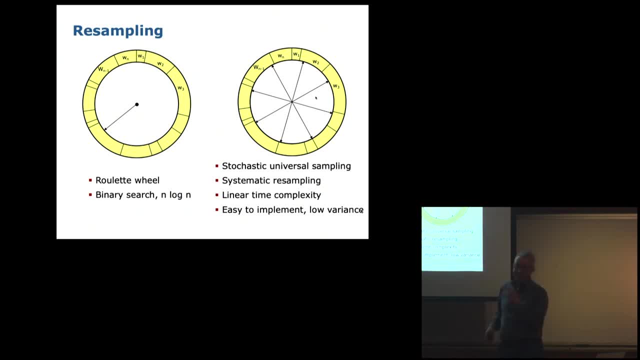 And the low variance is actually the key, And we will talk about this easy implementation in a second And I will point you to pitfalls there as well. I stepped into them as well when I implemented that, But it has low variance. So let's assume we perform. 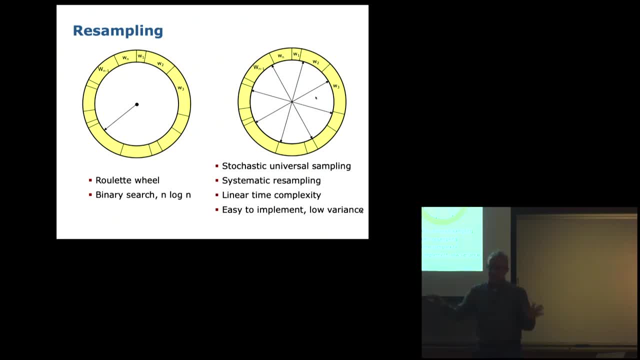 We have a weighted set of particles, And it doesn't matter now as to whether the weights are uniform or non-uniform, You just perform resampling operations. So let's assume what we do now is: we have a set of particles, We perform a resampling operation. 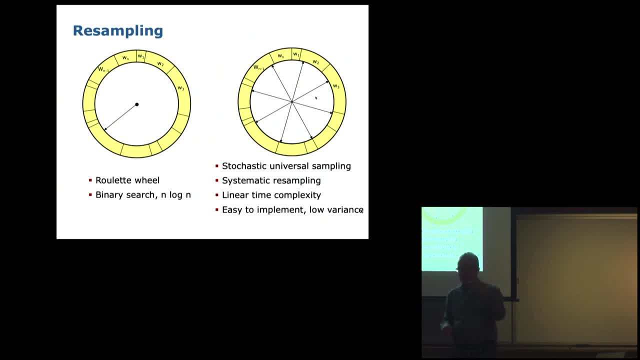 And then we repeat the resampling operation, Although these particles have the uniform weights already. nobody hinders us from doing this. That would just mean that these bins have all the very same size. And now let's assume we go back to that roulette wheel. 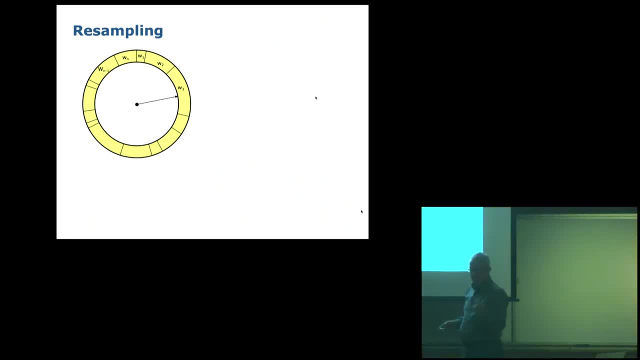 So what we are doing there is we are basically drawing angles and checking in which bin that falls and keeping that particles, And we are withdrawing all particles that don't get selected by this arc or this angle that we have there, by this arrow. 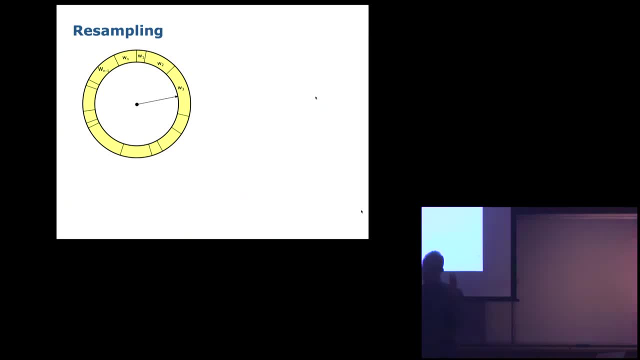 So if we do have n different, let's assume these are different particles And we perform this operation once. So what is going to happen In terms of? I know this is difficult to answer In terms of the diversity of particles. let's assume we have n different particles. 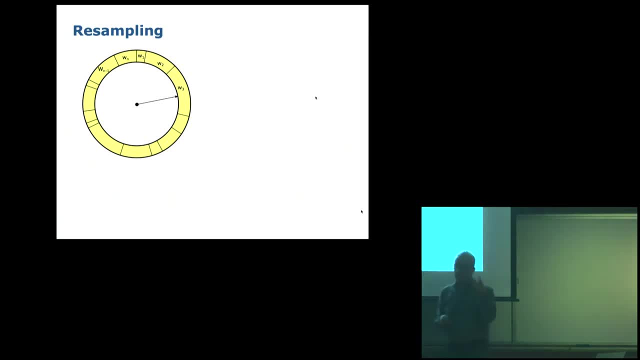 and they are actually different. And we perform this operation once, drawing n angles. How many different particles are we going to have afterwards? Slightly less. No, It is way less than that. How much that is, But it's not guaranteed that we will. 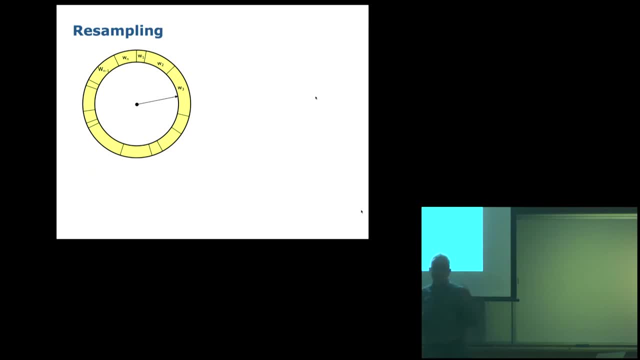 have n different particles And as time goes to infinity, how many different particles will we have if we do this infinitely often? Different ones, Like only one, Only one, Which means that we are going to lose diversity And in the end, we will have all the functional approximation. 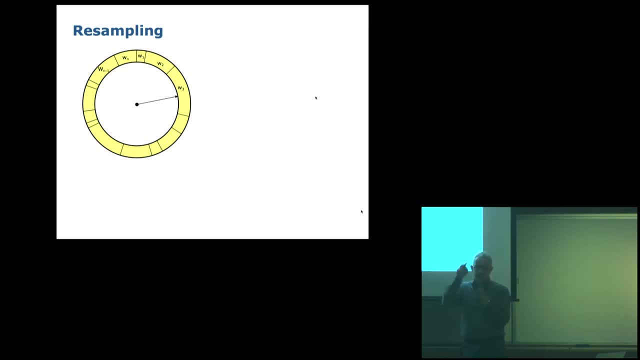 will be just the direct. We are going to lose the distribution at the peak of that particle set. ideally It doesn't need to be just. if you choose the wrong one, then you might lose the maximum likelihood particle If you perform the very same operation with this scheme. 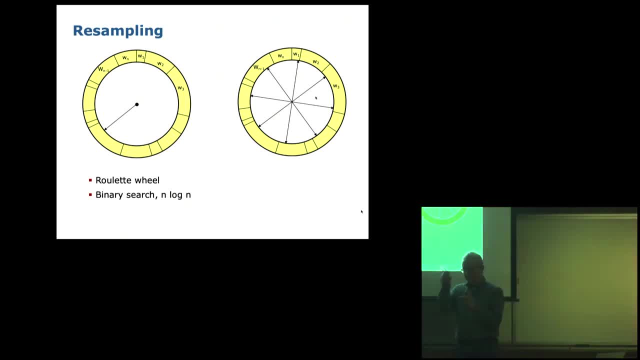 over here. so we draw an angle between and. now let's assume that all the particles have the very same weight and we have n different ones. All right, It's the very same weight. That means the weight of every particle is 1 divided by n. 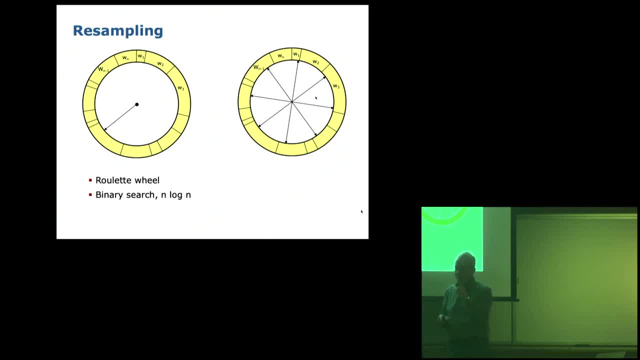 The first angle is drawn between 0 and 1 divided by n, And that's easy to implement, means we need to carefully think about the left and right border of that. That would be in the algorithm in a second, So let's assume we do this correctly. 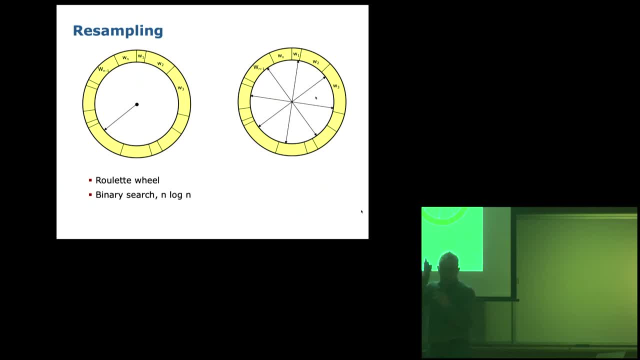 like dealing with the borders, Because if you exactly hit the border, if you choose 1 divided by n, we need to know: is this the left one or the right one? We need to be consistent about that. But let's assume we have done this properly. 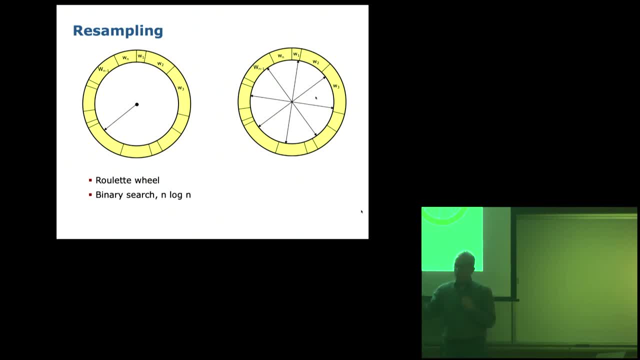 What is going to happen if we perform one resampling operation? All the particles have 1 divided by n as importance weight and they are all different. We do this once we have how many different particles n? So this is why that says low variance here. 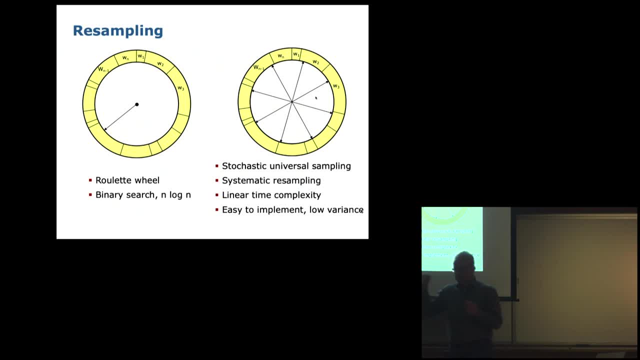 You're basically keeping the variance of that of that particle set And it is independent of how often we sample It might be. with this roulette wheel approach, In the worst case we are going to end up even after one resampling operation. 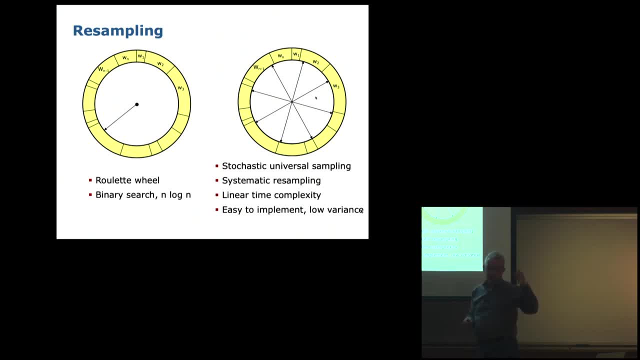 we end up having a diversity of just one particle Because all the arrows fall into just one bin. Nobody tells our random number generator that it is not supposed to do that. It has relatively low likelihood. but if you repeat that, then the variance about the particles 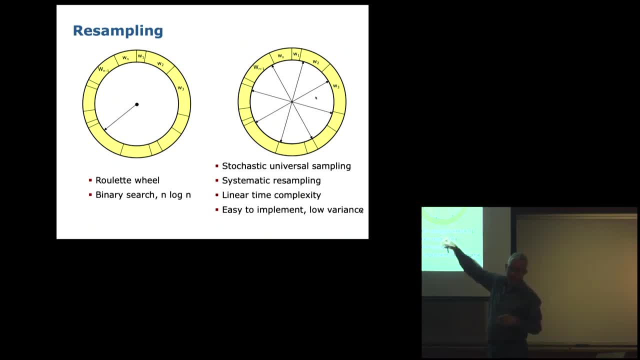 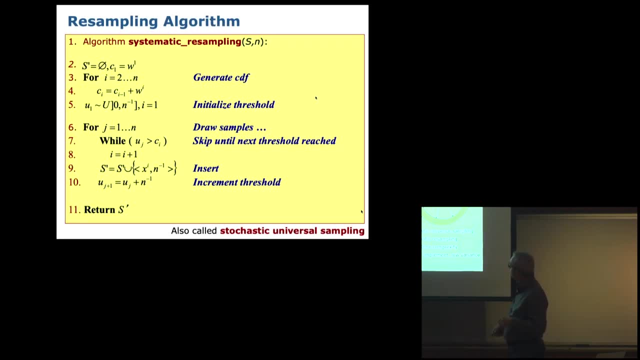 that you're going to have is you're going to have a lot of variance With this approach. it's substantially lower than with the left-hand side one And it's faster And, coming back to, easy to implement. this is actually how it works. 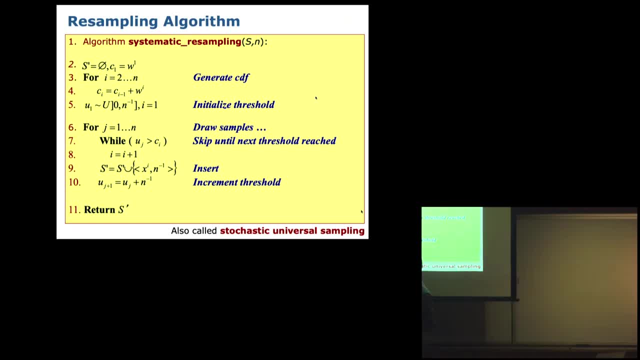 And you need to initialize these thresholds. In this case, I exclude the 0 and include the 1 divided by n. You keep this being consistent overall. then you actually- and this is the operation where you actually sum up the c's- 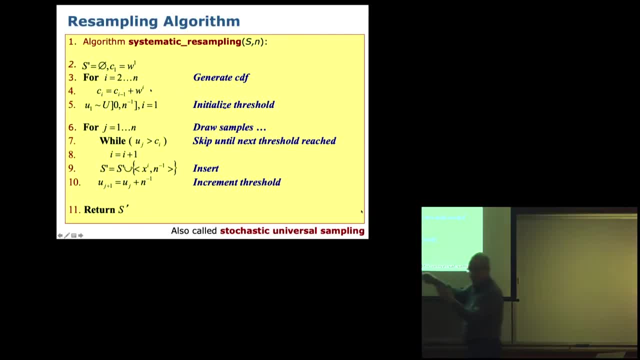 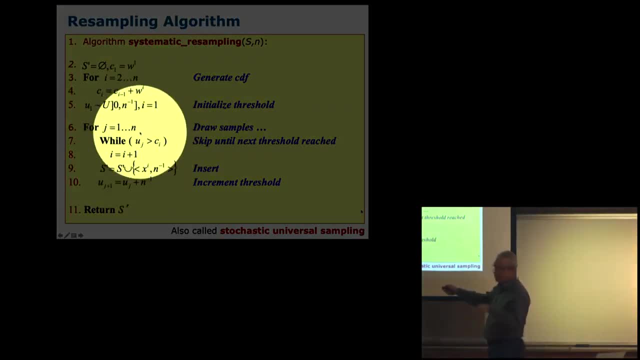 which are calculated over the. this is basically calculating the right-hand side borders of this, And then we run through the samples and skip the ones that we step over. That is this wide loop over here, And the ones we end in are those ones we keep. 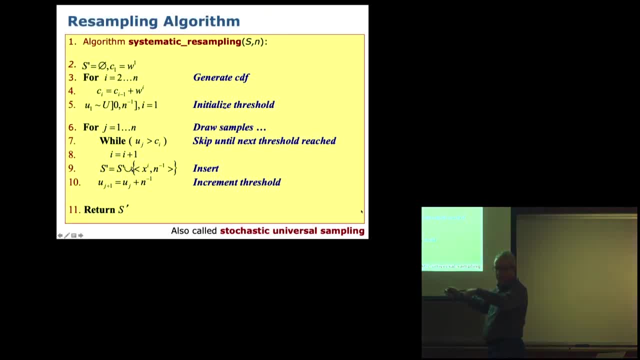 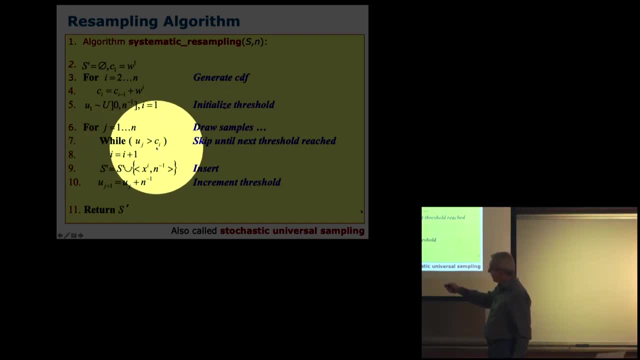 And then we increment this threshold, We have 1 divided by n. We could basically go to the next arrow, And you can see here that we never go back. We skip over some. So in the end we touch every of these c? i's which are calculated. 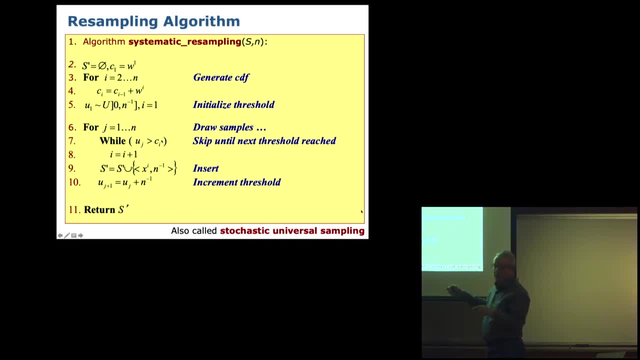 over the right-hand side borders of that interval, So we run just once over the entire particle set. Easy to implement is exactly that. Requires an afternoon also, depending on how skilled you are and debugging and all these kind of things, But this is basically the operation that is typically. 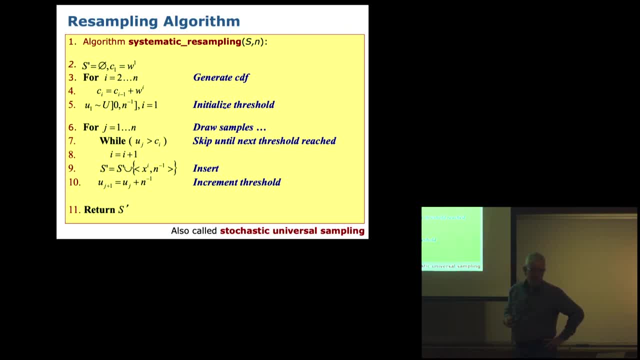 used in that context. Yeah, Is there any in any way that the other way of sampling would ever be preferred, Or is this just strictly better? I think I've never seen a case where the other one would be of advantage. It is particularly when you think about I mean, 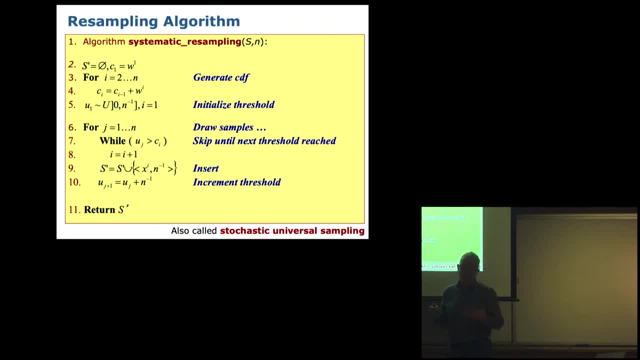 you're basically losing states And you're basically losing diversity. I mean every type of redundancy. if you think about this as a function, approximation basically prevents you from having a sample somewhere else that might provide you with a better way of approximating that function. 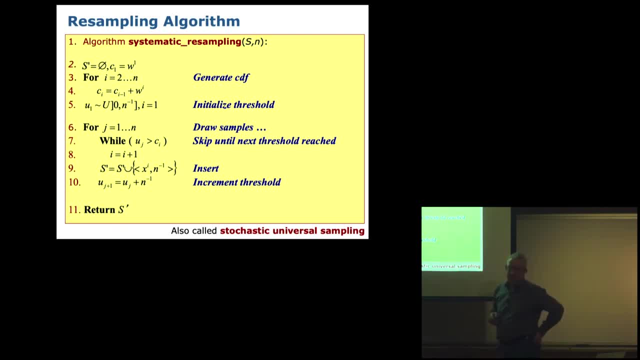 I never encountered any case or any paper that said that that other approach is actually better. But you might need to ask mathematicians about that, But my intuition is that no, That's a good question. So this is the way it works And what we're going to look at now. 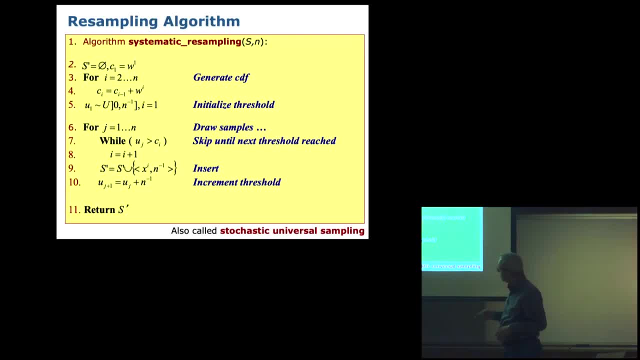 is how this can actually be used for, And the other thing is when you do. the other answer to this is in other contexts, when you are not just using this for localization purposes. these particle filters are extremely powerful Right now, when we speak about localization. 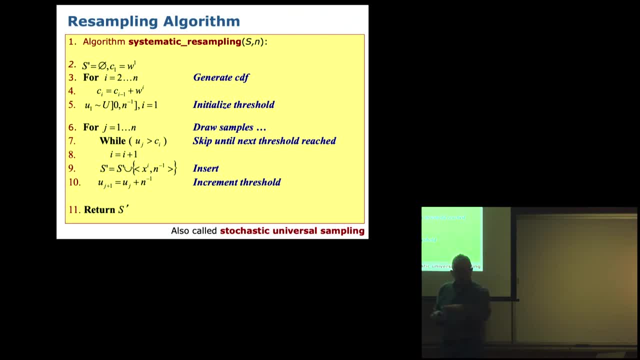 that is a relatively small state space for a vehicle living on a plane That is x and y plus the orientation, And so it's a three-dimensional state. And I mean throwing away three-dimensional states is not very costly. But if you think about alternative applications, 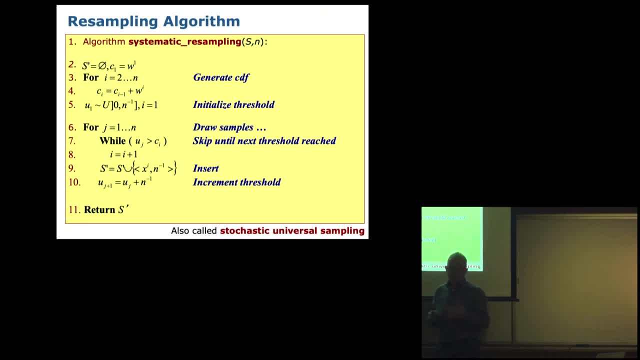 with higher dimensionals. So, for example, if you think about flying robots like flying vehicles, six-dimensional, Or it could even be when you do this in other contexts or when you add variables. For example, you can use particle filters also. 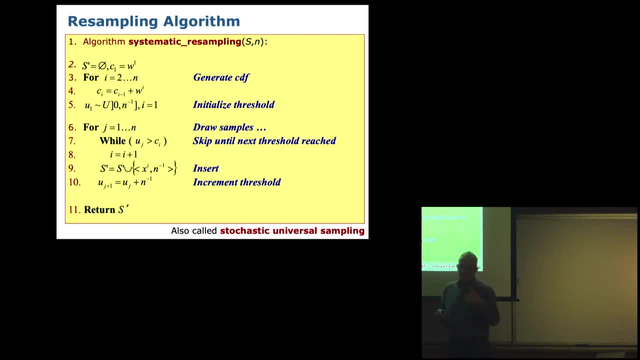 to estimate additional components of the state space. So we have, for example, used this for estimating the diameter of the tires of a vehicle, And the advantage of that is if you think about, for example, a stock lifter that goes from A to B. 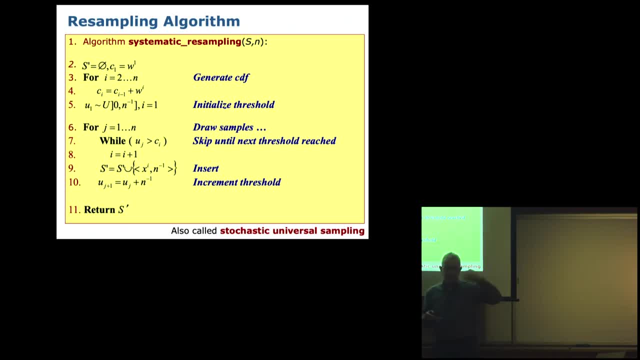 and lifts up the heavy loads, and when it picks up a load then actually the diameter of the wheel shrinks, which means that you need to have a different motion model or transition model, Because when you sample from a model that takes into account the wheel diameter, 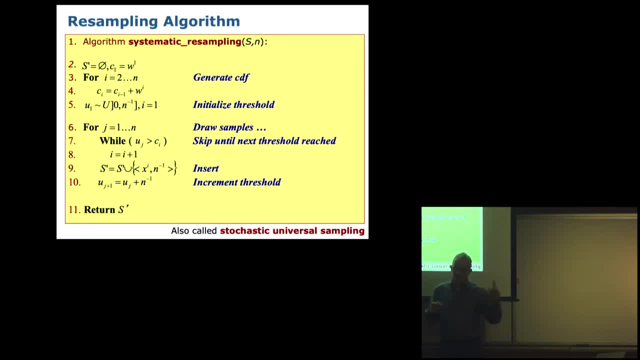 then you can actually have better predictions and have the particles in better places, which means that your, the state space is higher dimensional and you invest a lot of time computing these higher dimensions And then throwing away particles just based on a resampling operation. 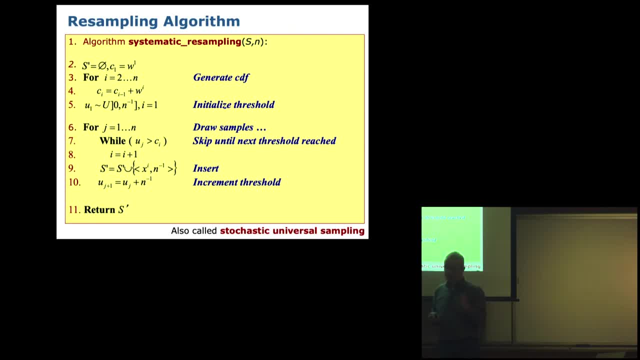 might then be not very, very effective And it can be really expensive. People have also used this for SLAM- simultaneous localization and mapping, And then in the particle filter context, the entire map becomes part of the state of the. you know. 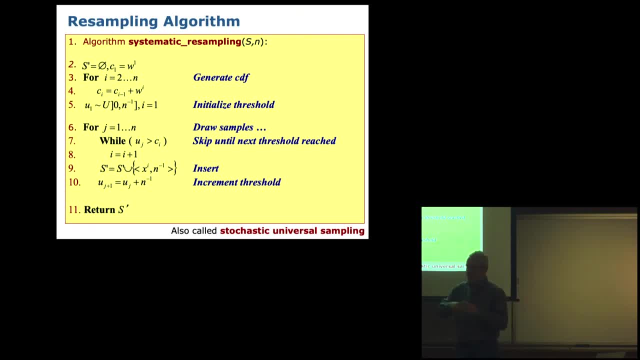 of a particle, which then means that when you perform this resampling operation in the wrong fashion, you throw away an entire map And that can be a huge fraction of your memory. So you invest a lot of calculations into these individual states that you then 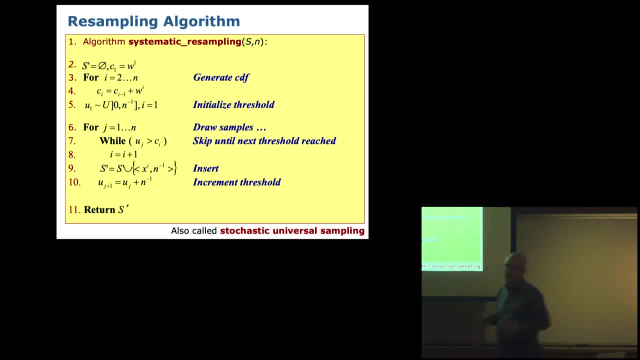 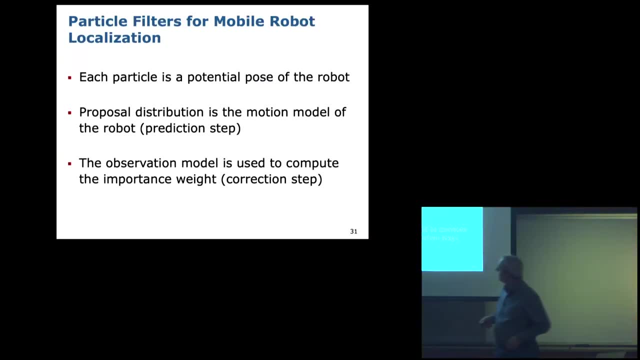 throw away using a suboptimal resampling operation. So typically you need to be very careful about that. So again, like in localization, and just to give you like a few examples, that actually works in practice and can be used on real robots like that is how this is done. 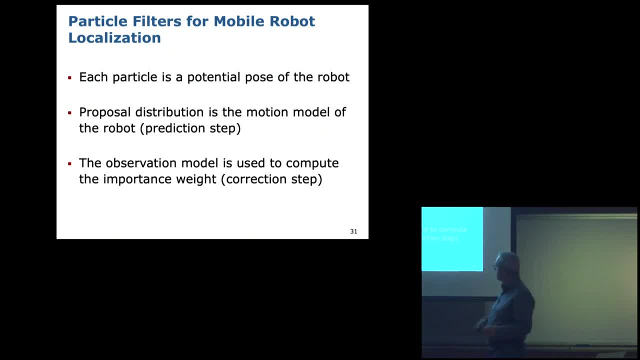 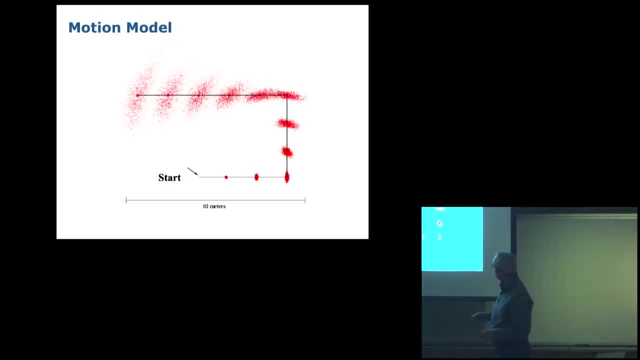 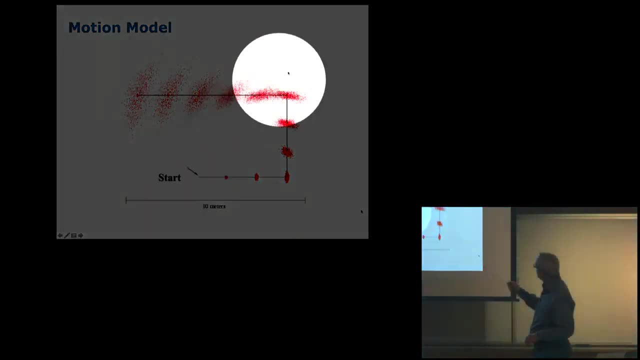 The proposal distribution is just the motion model And the observation model is used to calculate the importance weights. So motion models typically like this is. when you look at papers, they often refer to these banana-shaped distributions And the best spot here is like this part. 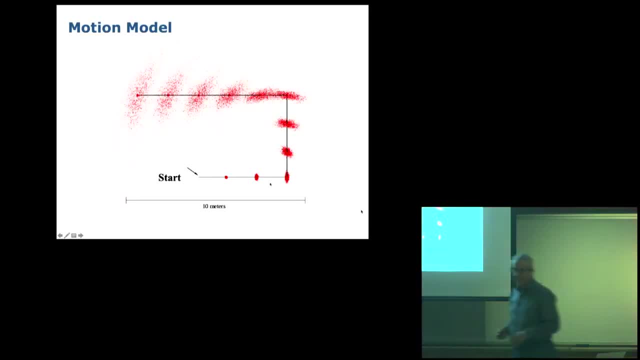 Or here you also have kind of like a little banana over here, That's kind of dessert banana that you have there, And so this is a 2D representation of a 3D state. So this is a robot. actually performs translational errors in x and y and a rotational error. 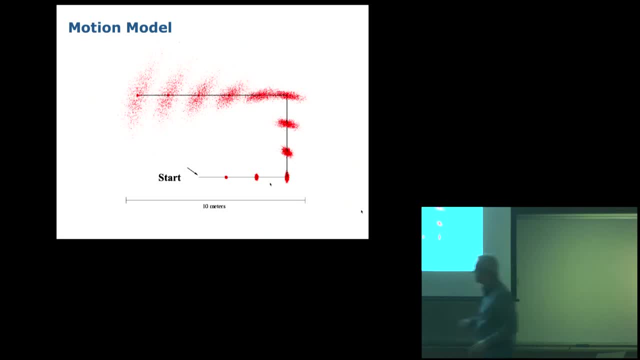 And it's just a projection of these particles onto the 2D space, And this is actually calculated from this function, p of x, prime given. So this is a 3D representation of a 3D state in x and u, And there's 10,000 particles starting at 0, 0, 0.. 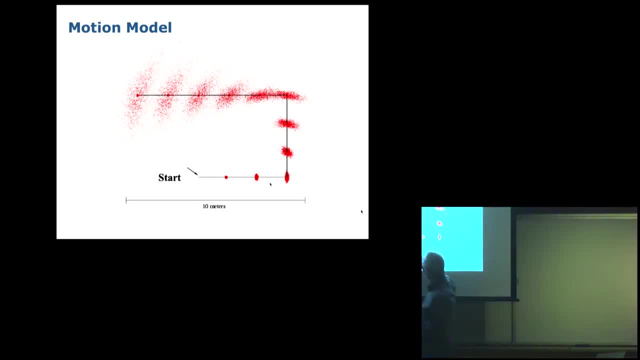 And then we pass all of them through that motion model once And in the very first case that gives a distribution like this one over here, And if we again pass those again through that transition model, we get a distribution like this over here: 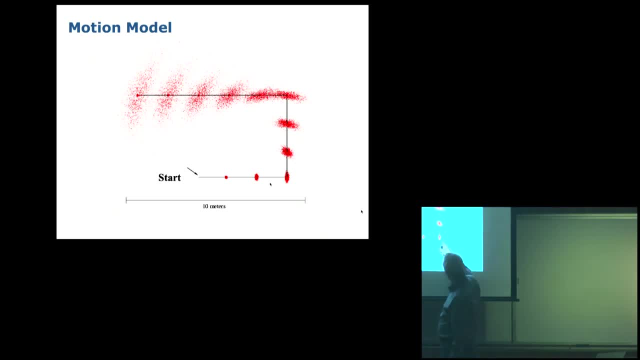 And in the third step, a distribution like this over here, And this distribution indicates something about the angular versus translational error. So when it looks like a vertical, like a banana, that is kind of like a banana, is that because in practice, 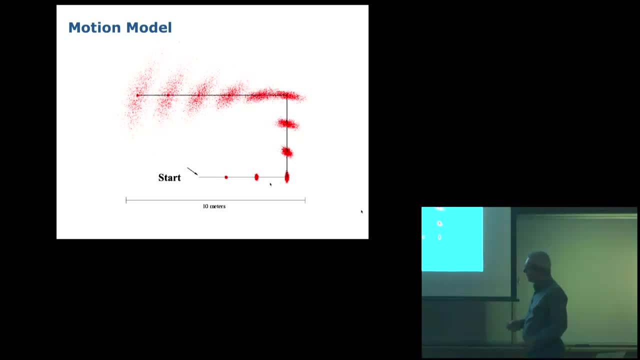 it's a little bit curved here And so that is basically the case because we have a relatively high error in rotation here. So that model, this is a robot that it does relatively high rotational errors If you have low rotational errors in your transition model. 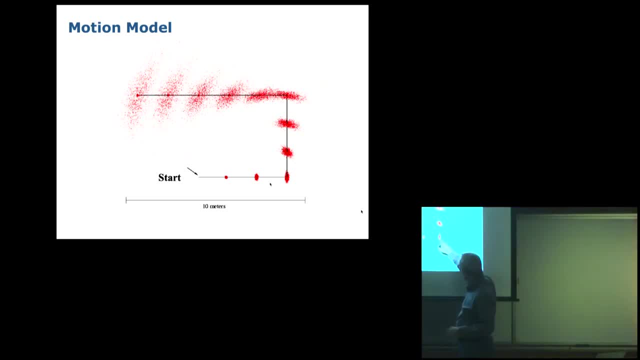 then those particles will be peaked And this distribution will be more longitudinal, because I mean it's more, let's say more circular, because x and y might be the very same, depending if you have more in x, which would be that direction. 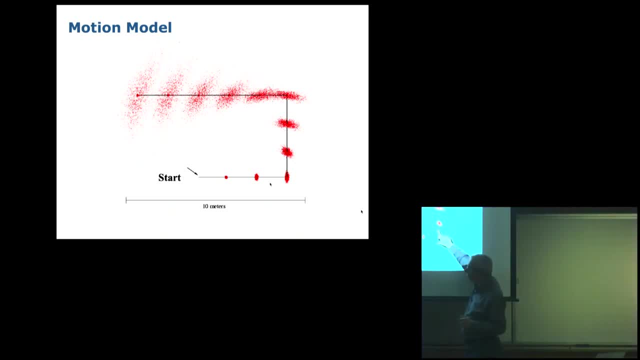 and it would be more longitudinal. if you have rotational errors And that forces it to elongate along the y-axis in this plot? Yeah, In this case, because every particle is equally likely. when you resemble, you have to just quick-hide, right. 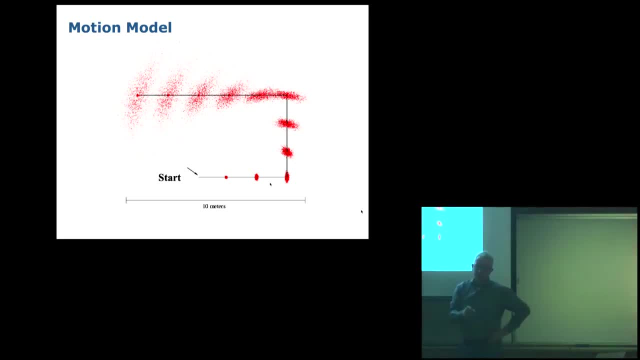 Actually that is just like. there's the advantage of the particle filter over other representations like histograms. It just stores x, y and theta. It's just real numbers that you have. Every particle is a triple of real numbers: x, y. 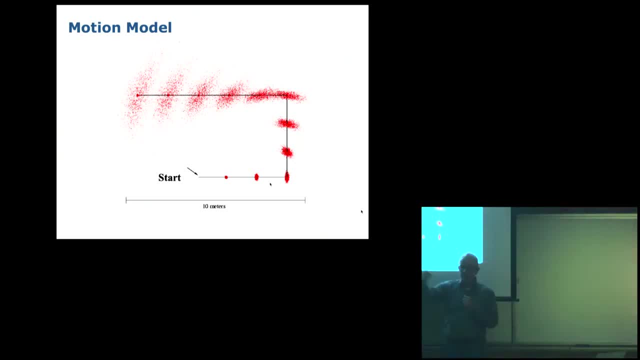 and theta the orientation. And then you use this rejection sampling scheme through that function p of x, prime given x and u, You pass it through. or basically we tend to say: we calculate a potentially new space according to that transition model. 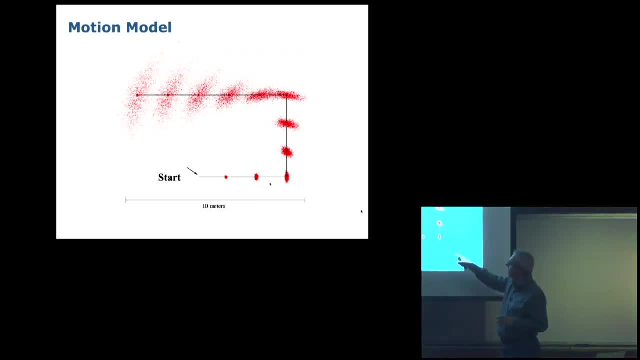 That needs to be carefully designed. This is basically like the repeated operation of p, of x, prime given x and u, And here we sample that set from this set And basically what we are asking is: where would this particle end up, given the operation by the robot? 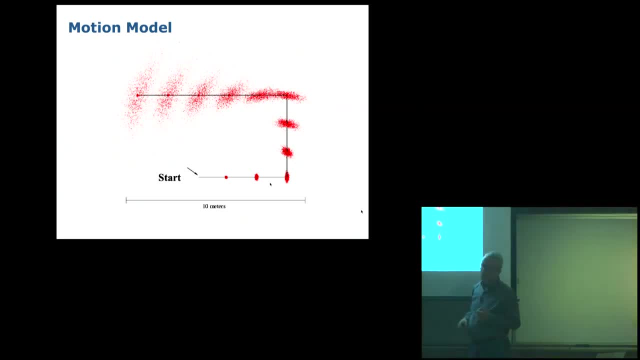 And this is basically that black line over here. I do not know what the units were. It's just for, say, it's 10 meters here, maybe something like 2 meters or something like that. Well, it's actually according to a motion model. 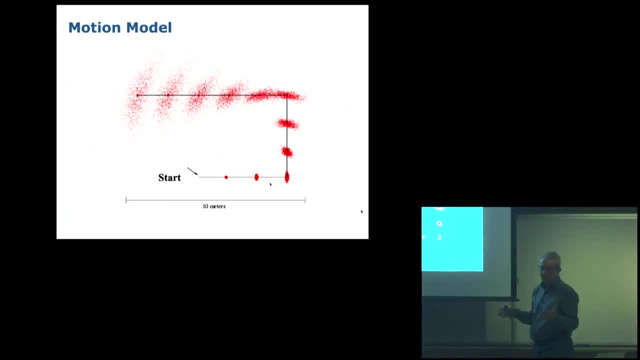 where you can say, for example, a very, very simplistic one could be in every step. we do have a normally distributed Gaussian error In the translation in x, a normally distributed muted error in y and a normally distributed muted error. 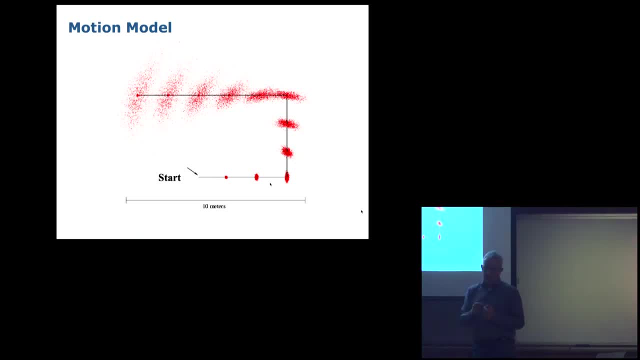 in the rotation of the vehicle. So basically, use a normal distribution. You assume these errors to be independent. So if you take your current hypothesis- x and y in theta- and you draw on x prime, y prime and theta prime, 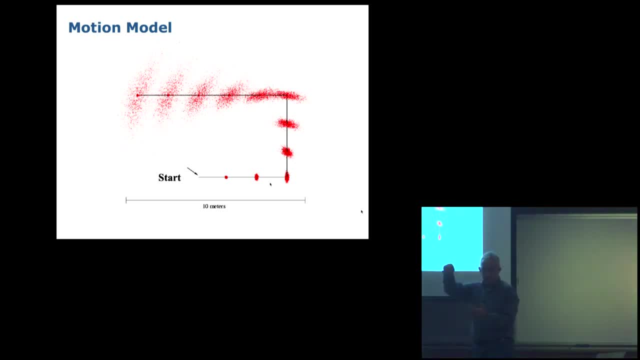 according to this Gaussian, which is centered at 2 meters and then for x, and centered at 0 for y, with different standard deviations, and centered at 0 for the angle as well, or the angle offset, And then you add those to your current hypothesis or particle. 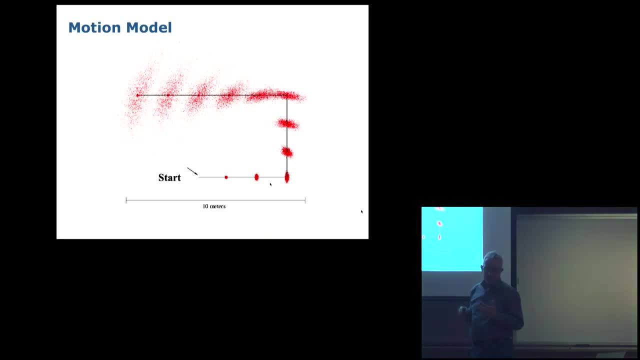 And this is where these positions end up. It's basically that operation. Does that answer your question? So that might be a motion model And this is one of the observation models that you might use. So this is just the statistics of how often you actually 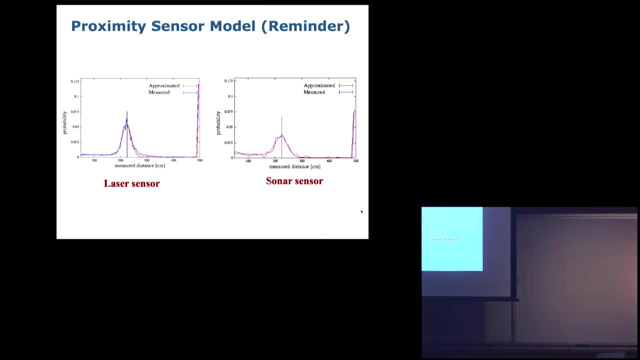 measure a certain distance, given your map tells you how far things are away, given that state of the particle. So, given you have a map, if I do have an ultrasound sensor and it tells me it's going to be 3 and 1, 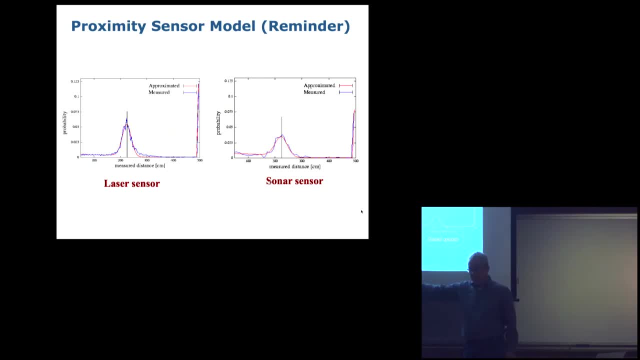 half meters up to that wall over there and my sensor points into that direction, given the state that I'm currently in. if another state looks like that, then the distance is larger, so it will have a lower likelihood And in fact those states where I'm exactly 3 and 1 half meters. 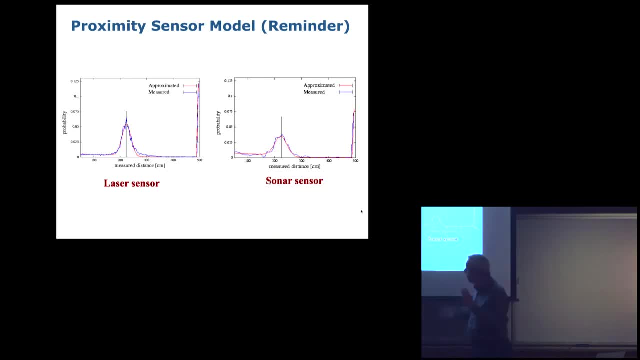 away from that. they are actually extremely likely, or more likely than others. And here is that plot, for I think this is. it doesn't matter, this is 2 meter 30 or so, So it's basically according to the state of the particle. 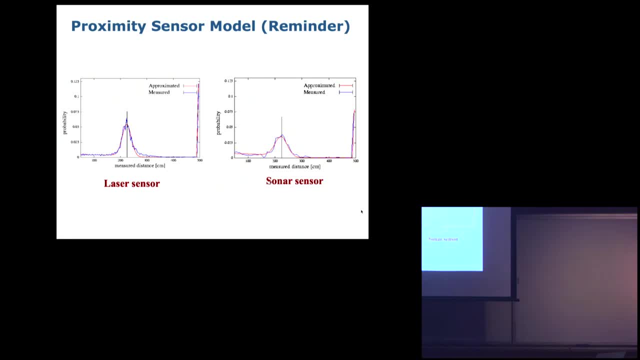 in the direction of the measurement. that would be, I would expect In the map to measure 2 meters and 30 centimeters, something like that over here, And then we can read from this function- this red function is a typical likelihood model. 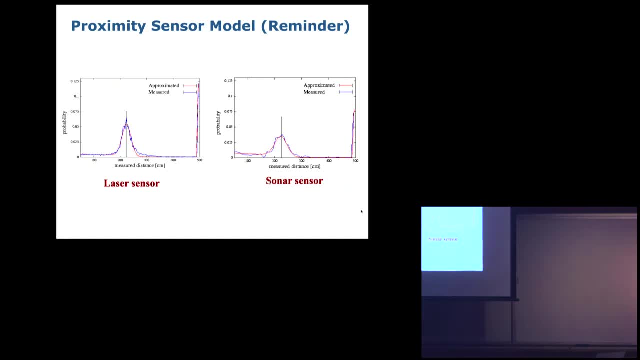 We look at. if the sensor measures like 2 meters, then that would be the importance weight. This can be done, implemented very, very effectively, in just lookup tables. You basically can discretize your observation likelihood in case of low dimensional ones and then just convert it. 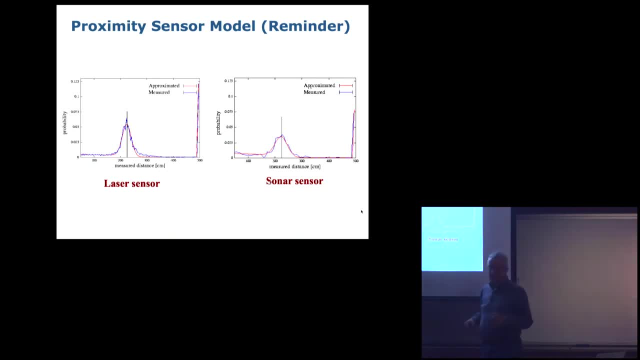 into a lookup. So every operation here for that likelihood importance, weight calculation is just a lookup in a table. It's super fast And you need to pre-calculate this for all distances. It takes a little bit of space, but it can be done very, very effectively. 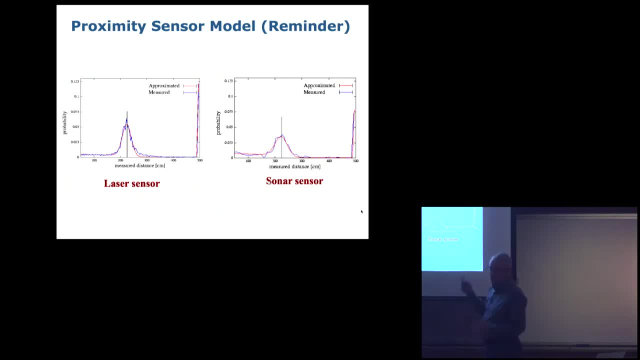 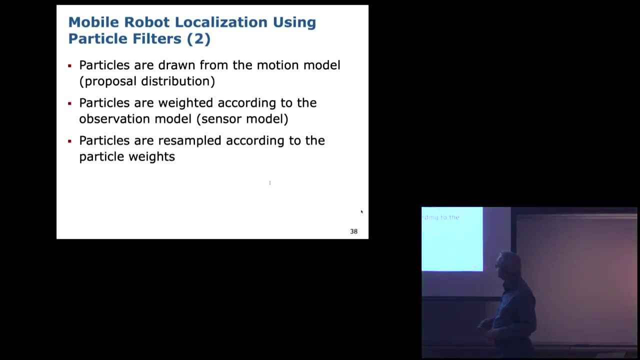 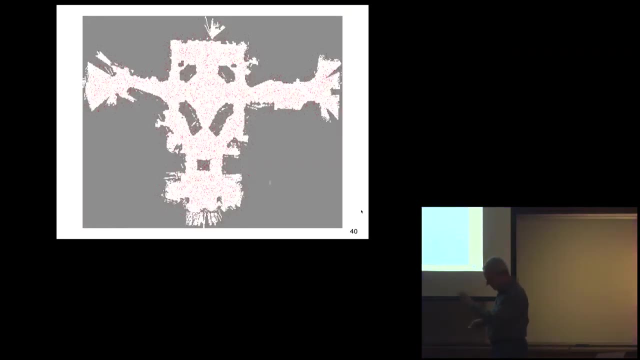 if you have dense depth measurements, for example. So this is a way how to get these importance weights. So, again, this is with the operation that we want And what we are interested in now resampling. We spoke about this And this is an example of an application of this. 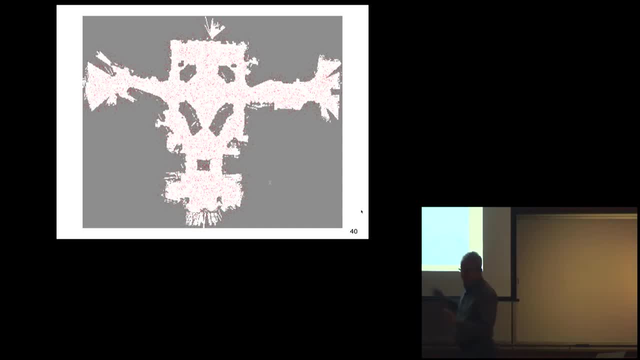 This is a real data set. It's actually more than 20 years old. this data set And these figures that you see here is one of the very first applications of this used in that case, data from Minerva, a robot that we 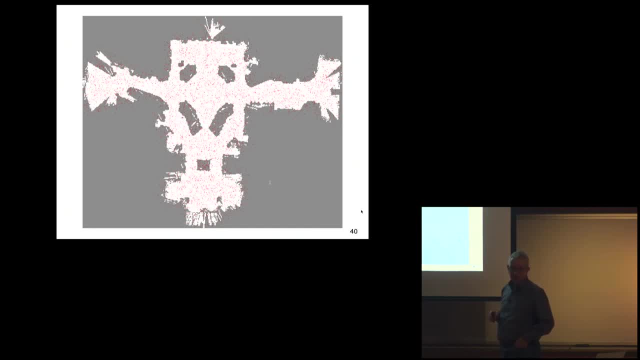 installed in the Smithsonian Museum of American History in Washington DC As a tour guide And you can see, in some cases, spurious measurements simply because people walk through that museum as well, And the goal of that robot is actually to perform global localization. 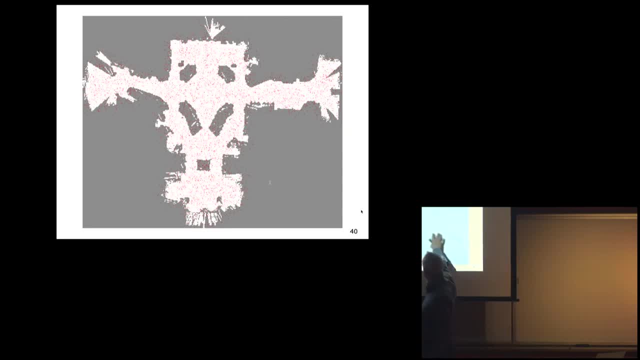 So it uses its laser range scanner to measure distances. You see in gray the map that we used. So basically, it just displays the borders there And just for visualization purposes, it transitions between white and gray. It's actually where the surface of the obstacles are. 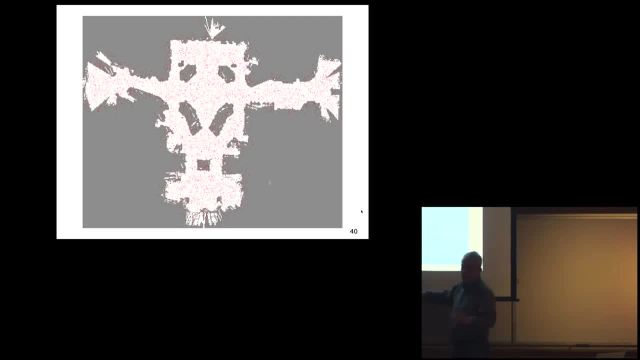 So what we have now, in the very beginning, is a randomly distributed set of particles, Random in x, y and orientation. Orientation is something we don't show here. So the first step, this is the first measurement actually depicted at the most likely state. 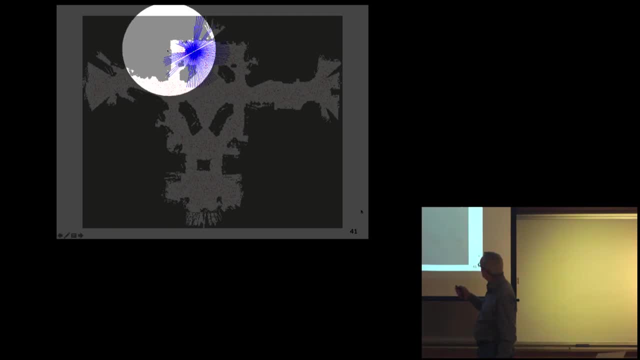 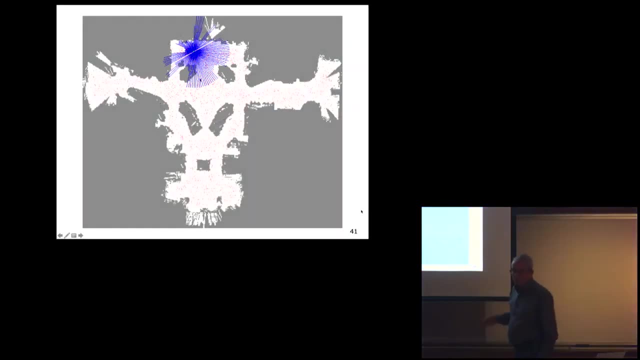 It turns out that these are actually us over here. We had our desks at that spot, So that corner is actually this one over here, So it's relatively close to the true pose. The problem typically is that you never have a hypothesis at the exact right spot. 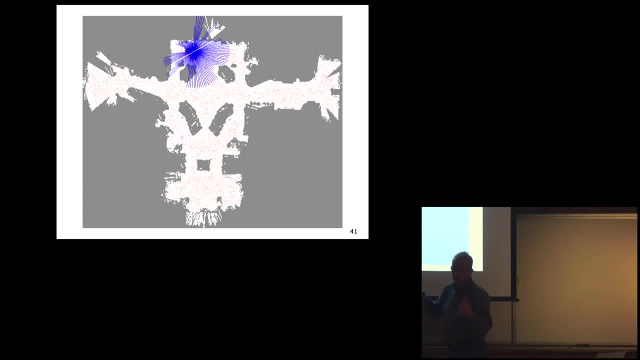 in the very beginning. So it's kind of like a trade-off between how many particles you need or you want for initialization purposes And also what your computation time is that you can spend on a vehicle. Turns out that- And you will see that over time- these particle sets actually 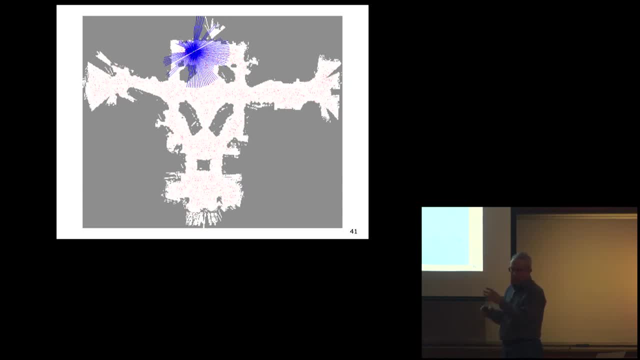 converge to the true pose of the vehicle And all these particles are located at the true spot of the vehicle, which means that for approximation purposes you do not need to have 10,000 particles, as long as you are confident or the system is confident. 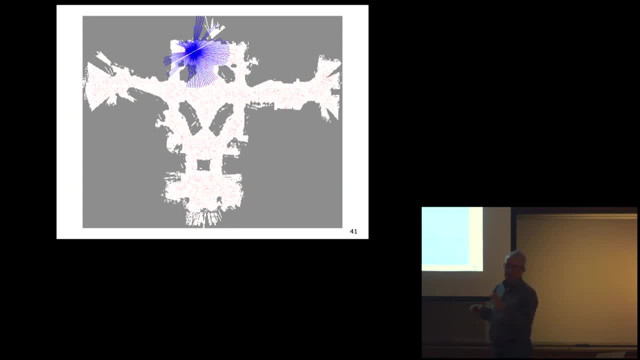 where the robot is, And this is why there are also schemes of dynamically adapting and adjusting the number of hypotheses or particles and so on and so forth. But let's First of all look at how that works. So we get: the robot is always depicted. 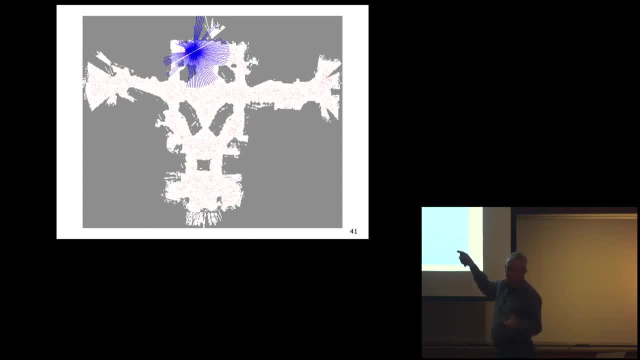 at the particle that is most happy. And the most happy particle is that one with the highest importance weight. And already here we see orientation is kind of OK-ish And it's close to where it is. So what we do is we weigh these hypotheses. 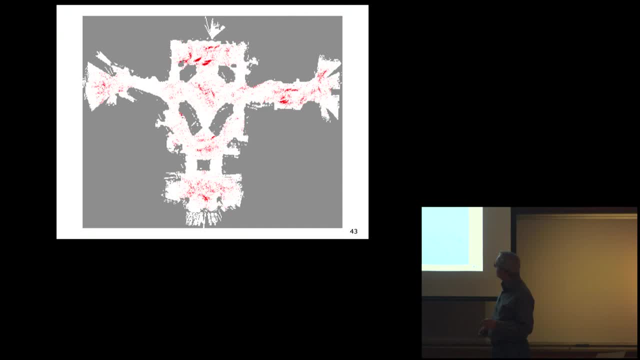 And darker means higher weight, And then we resample. We will see this in a second. Then you will actually see a better contrast there, But here you can see a couple of hypotheses emerging. So next step is that we calculate the importance. 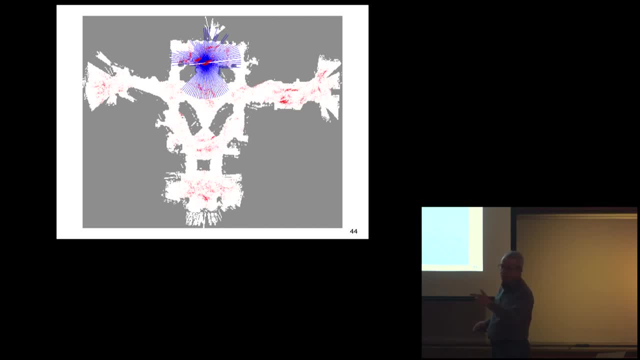 weight again resample and then propagate according to the movement. You see now that we are actually closer to the true pose, And the interesting aspect now is by the fact that through that resampling operation we get more and diverse particles in the areas of high likelihood there's. 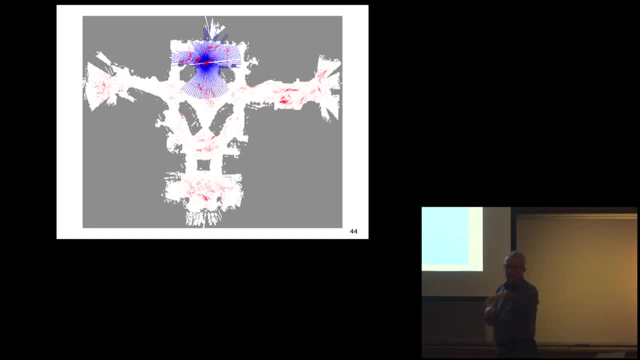 a higher chance of actually getting closer to the true pose of the vehicle. So we accumulate more particles in the relevant areas of the belief there, Which means we actually kind of like, if you think about this, we are in a gradient and getting closer to the true pose. 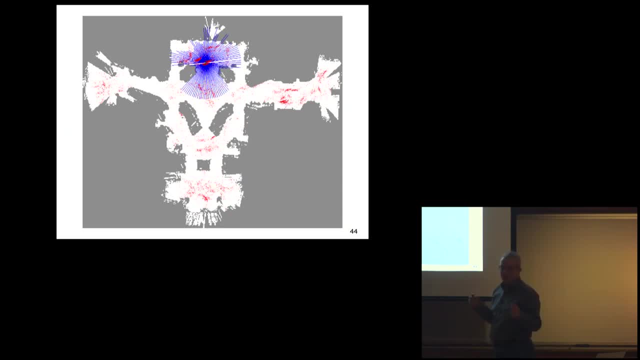 And there's a disadvantage of the particle filter: You never get the maximum of that, the maximum likelihood. You can only get an approximation of that And for that you would need to have like optimization-based approaches, like smoothing techniques. 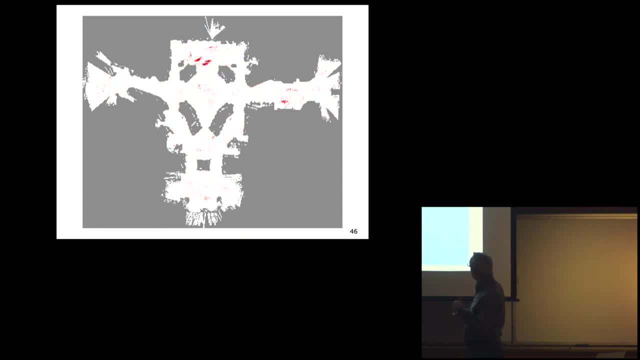 So next again is like: weighted according to resampling operation, propagating the particles, And now you see how dense that gets. So all the 10,000 particles are close to where the robot actually is, Actually nicely fits. Map is not accurate, as you see. 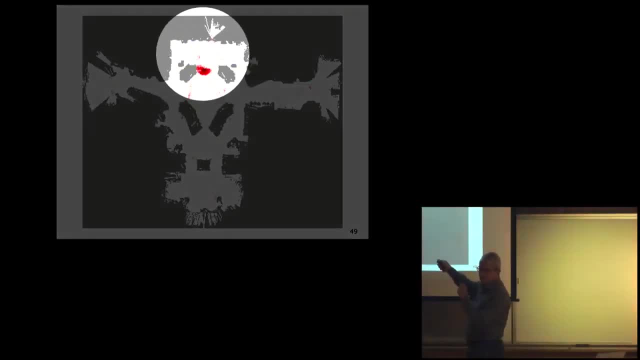 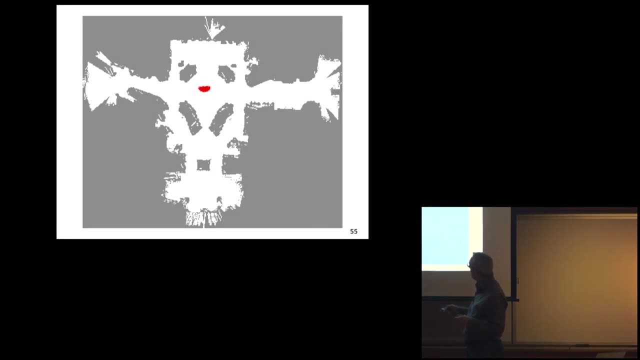 Here now you can see carefully that in the center it's actually darker. And if you keep going, All right, OK. So it keeps accumulating the particles. And then, whenever you do this prediction operation, the particles spread out because of the uncertainty. 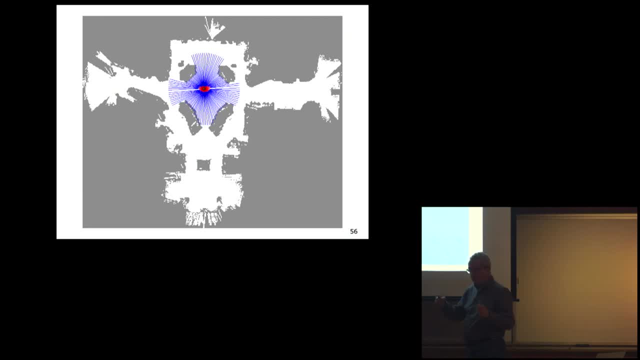 in the robot's motions. It's kind of like a trade-off between the prediction, where you actually try to capture everything that might happen from step t to t plus 1. Then you have the correction, the perception, that tells you what actually happened. 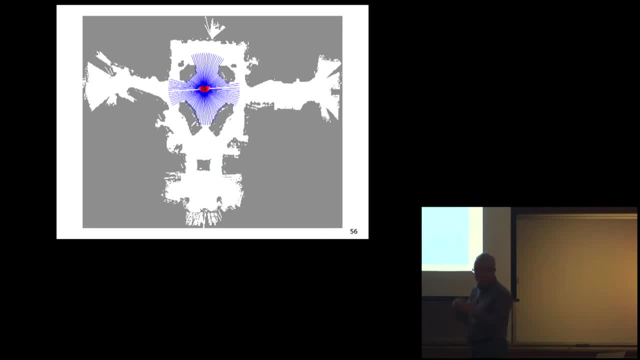 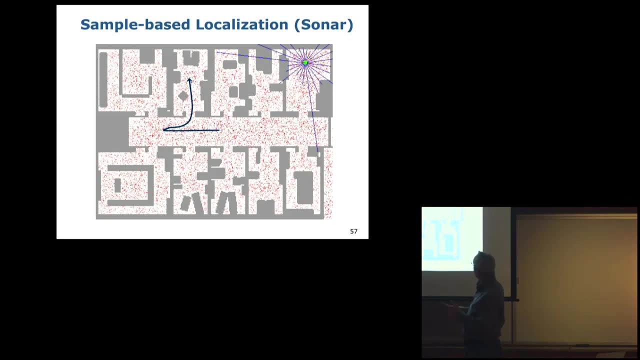 And that focuses your display So you can see that the robot is now in the center of the space again. And when you implement this, you need to carefully design those two components. This is why they are so super important. And here's another example of one of the famous videos. 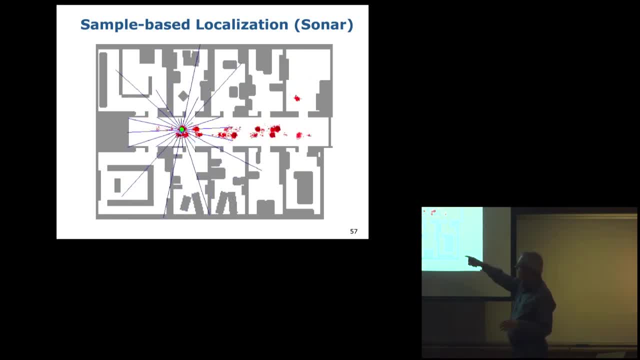 of a robot performing global localization in a highly symmetric corridor environment with ultrasound sensors. And you see all these hypotheses, multiple hypotheses, simply because the robot doesn't know exactly in front of which door it is, And so you can see the measurements going through the doorways. 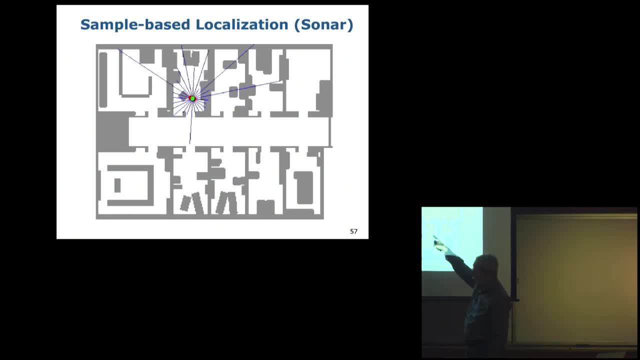 And the corridor is also rotationally symmetric. That's why we have two peaks, And those can only be distinguished by entering one of those two rooms. Interestingly because of the higher uncertainty there. at the end the particle set also bifurcates. 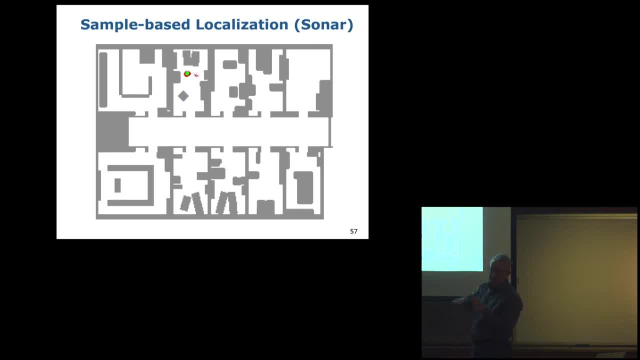 It's happening now. Do you see that? Because it might be the case that the robot actually had turned right, although the measurements are turning left, And then like, if you keep going, that actually sorts. It typically sorts out, But that doesn't mean that it always converges. 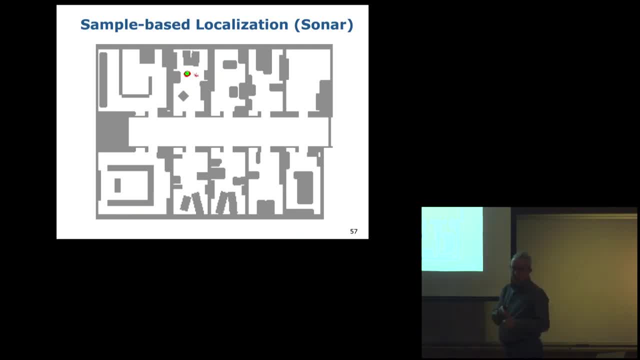 Even a particle filter can diverge in cases where your motion model is not correct. You're overly optimistic with the motion model. That is a typical source of divergence, And the other one is if your observation model is not correct or maybe also too strict, if it's too peaked. 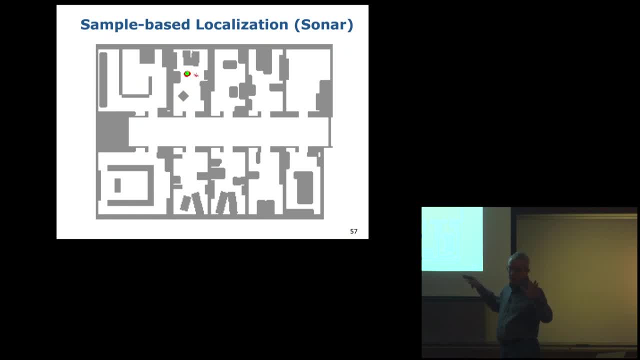 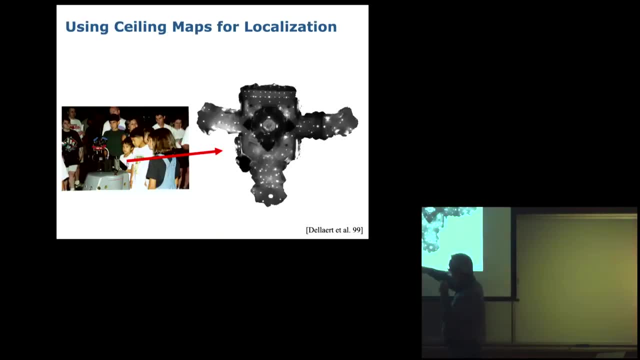 then you throw away too many particles in the reset And that's not a sampling operation. So you might be overly confident about where you are. And here's another example, also from Minerva. This was a robot, very same environment, And it's actually a super simplistic sensor model. 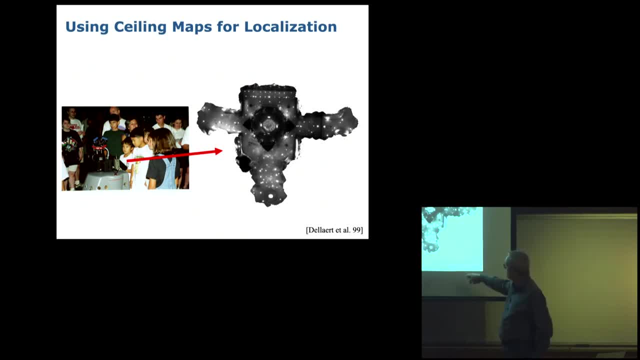 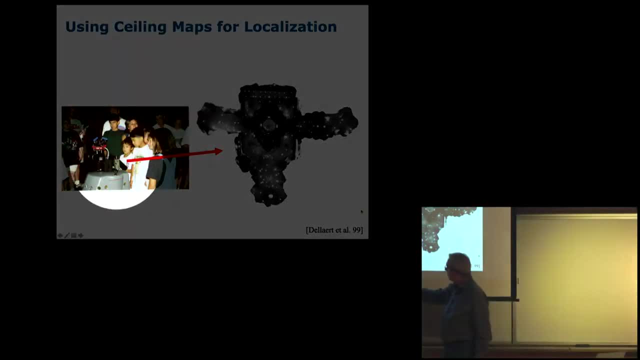 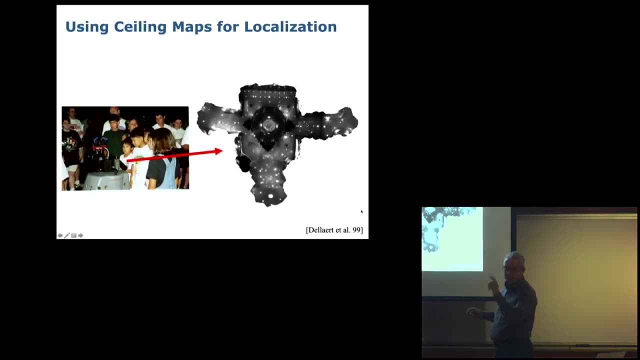 that is a ceiling mosaic at that time generated by Frank Delaert of the upward-facing camera over here And from that we took all the pictures And Frank was interested in mosaicing. He generated the ceiling mosaic of the Smithsonian. 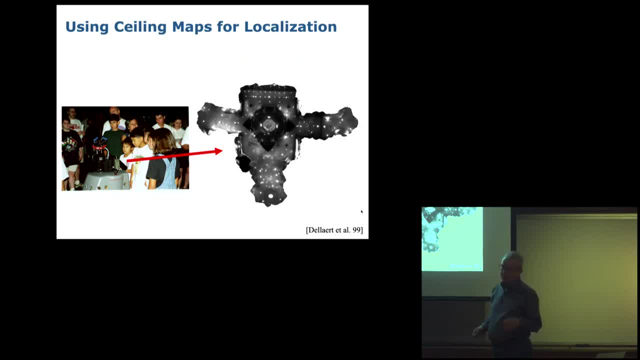 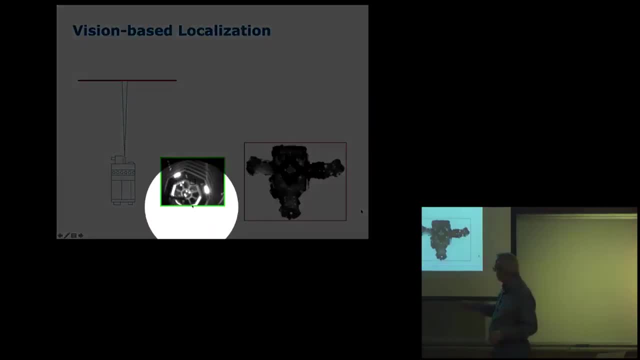 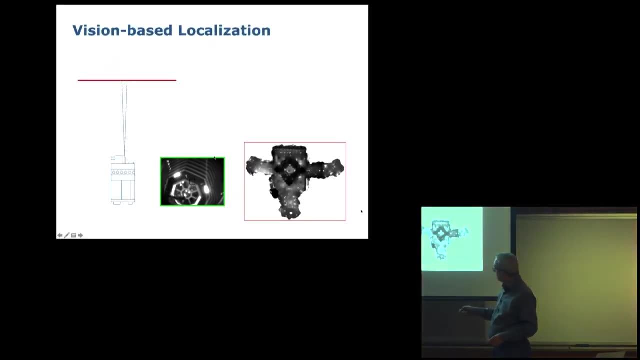 And you see all the lights in there. And then I designed a super simplistic model for that. We basically took the center part of that image, of the current image, blurred because the robot is in motion and the floor wasn't even. So I took those. 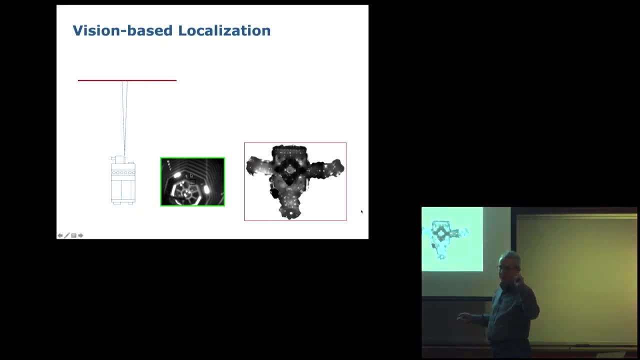 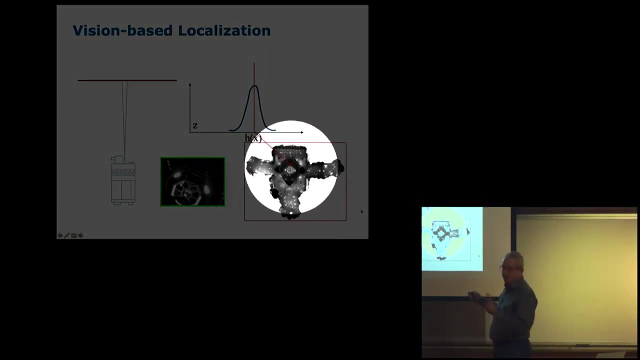 I think it was 10 by 10 pixels over here and calculated the average intensity of that image. And then I had a very, very simplistic error function which is basically nothing else but a Gaussian. I looked up: given the state of the particle. 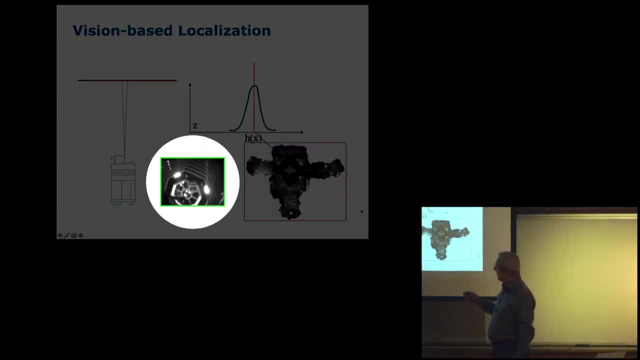 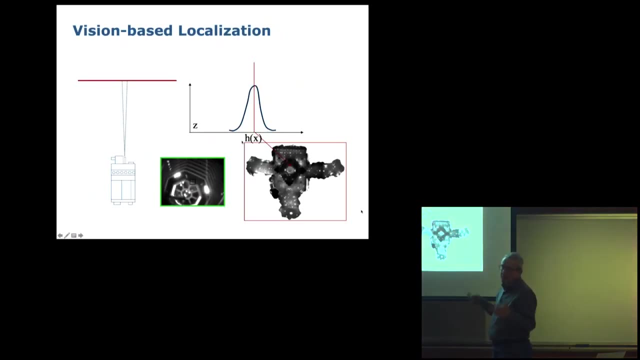 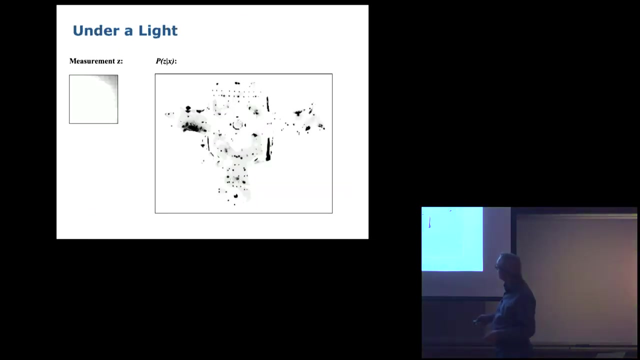 what would the intensity in the mosaic? what is the intensity that? the average intensity that I measure, And then I used the Gaussian to basically do. it's basically the square distance of those individual pixels, And then that gives you the likelihood. And once you do this, I hope this video runs. 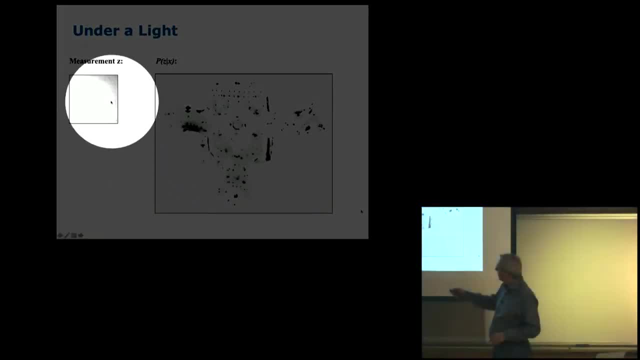 So there are a couple of measurements. that's actually interesting. If this is your center image, then maybe it's more 20 by 20 pixels or so, And then you can actually calculate p of z given x, given that mosaic. So, for example, this is when you're under a light. 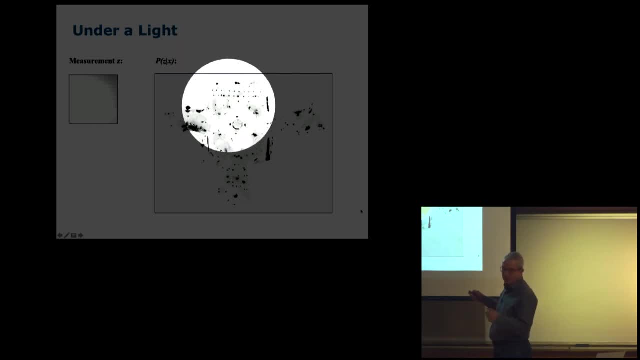 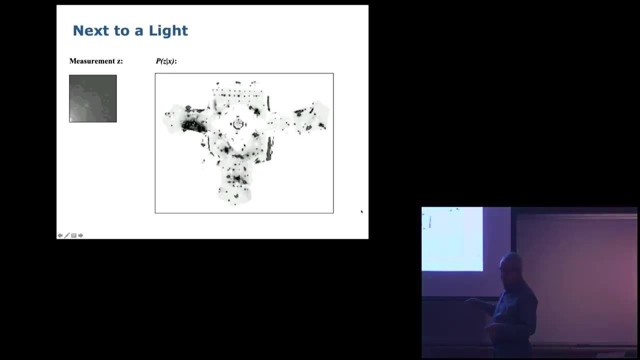 And actually there where lights are, it's dark means high probability, And when it's dark it's a low probability. And then you do have next to a light. Then you can actually see in that distribution that there are black circles around. 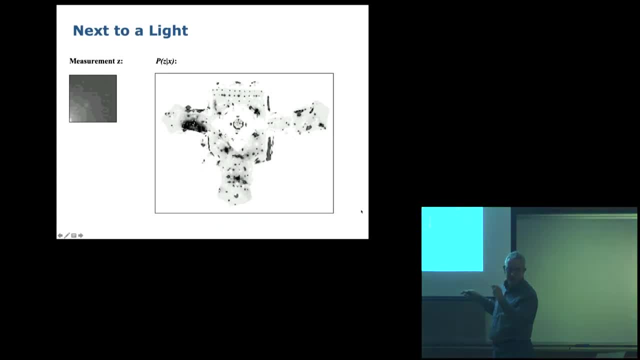 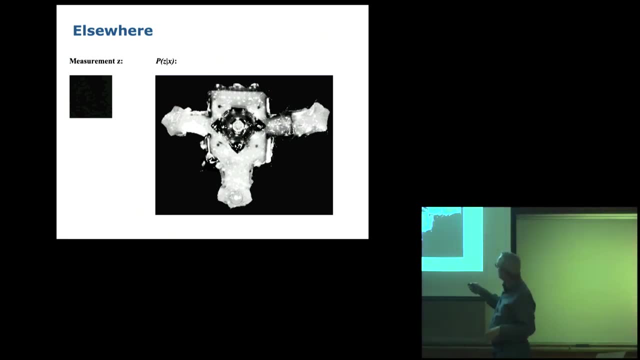 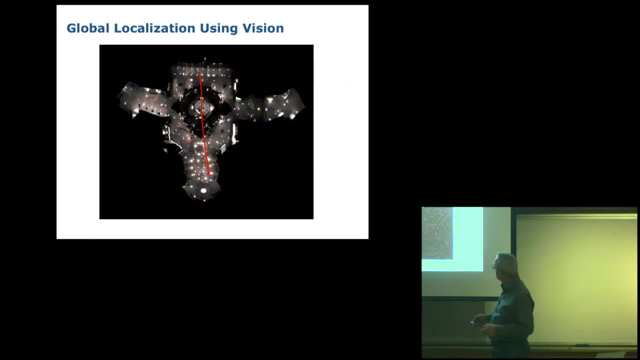 the lights. So everywhere where you are around close to a light, it's higher likelihood than anywhere else. And this is if you are under, when there's no light, then lights have very, very low likelihood, And if you let this run, this is a true trajectory. 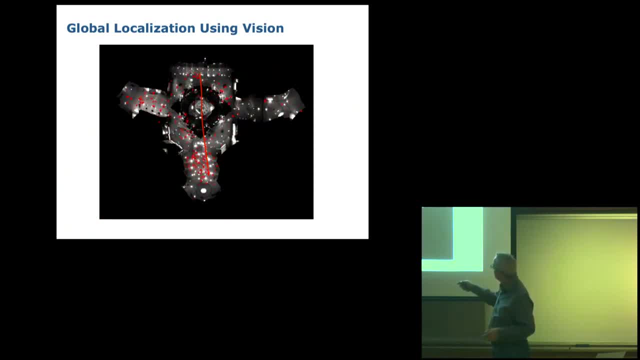 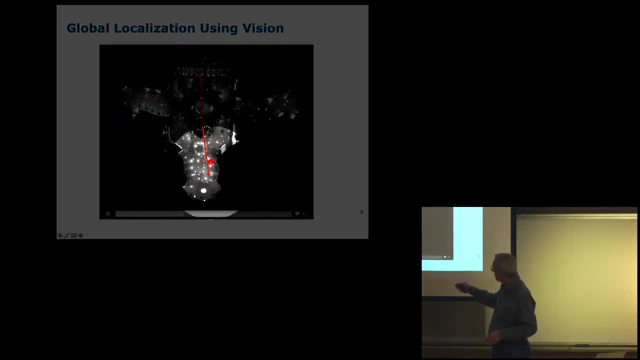 I think again 10,000 particles. So there's a yellow dot in here. that's here This thing is. it's hard to see, but you can see from time to time it was screen grabbing and it was not that good at that time. 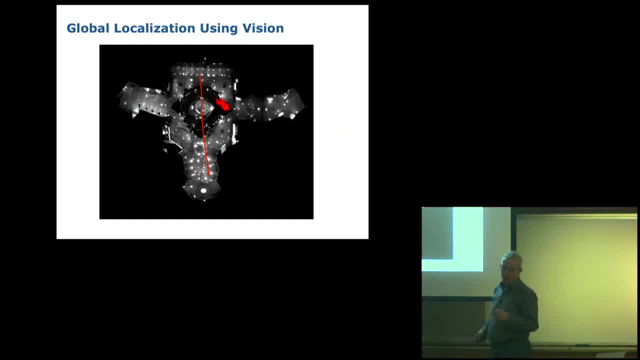 So you can actually just with this super simplistic model, you can perform global localization as a robot just based on ceiling lights. And this is something that differentiates the particle filter from other types of filters, like Kalman filter: that it is inherently able for doing this. 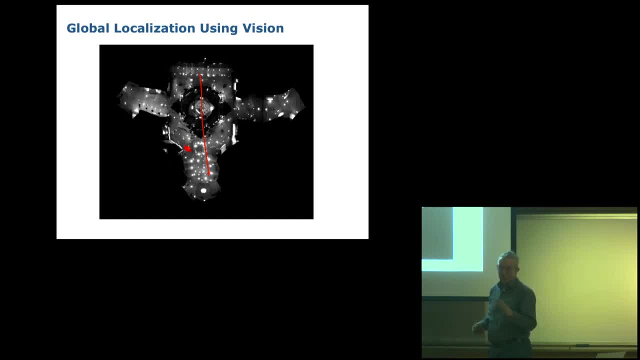 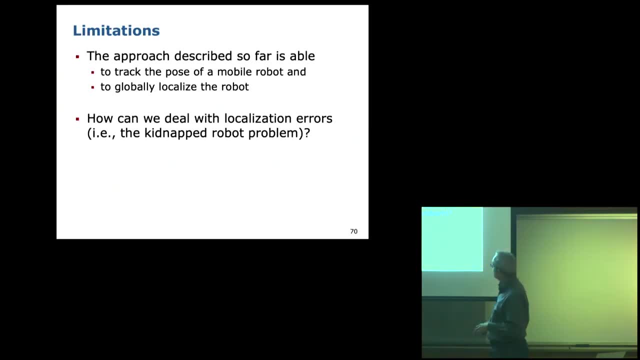 A Kalman filter can also do global localization. It doesn't mean that it cannot do, but because of the low amount of linearity it's actually more complicated. So what we basically can do, as we have shown, is we can do global localization, which? 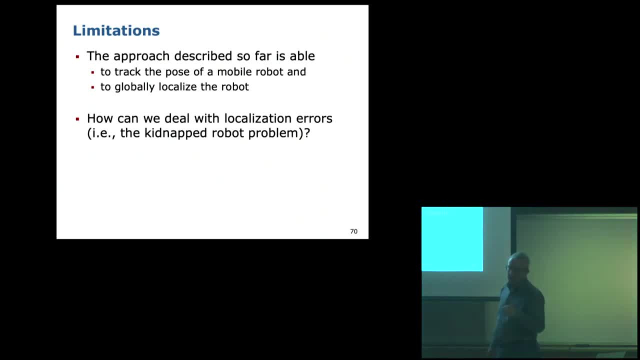 is pretty interesting, So you can initialize it and it can keep track. There are extensions for that for dealing with localization errors. Kidnapped robot- problem that's popular in robot soccer, where you take the robot, put it to another place. 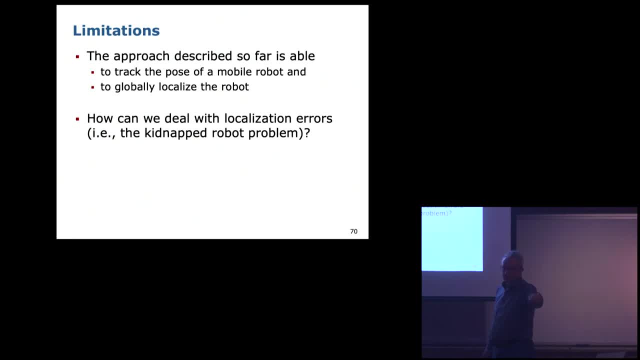 and the robot has to figure out that it made an error Right Or that it's somewhere else. now There's several ways of doing this. People have started modifying that particle filter algorithm, but that's actually the wrong way. The right way for doing this is changing your transition model. 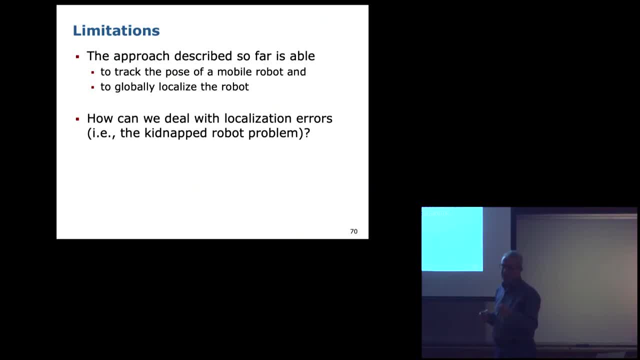 And one way would be to basically guessing at every point in time that you are teleported somewhere else, meaning that you need to have in your motion model, need to have a component that says: I'm not taking your odometry, I'm guessing a random spot from time to time. 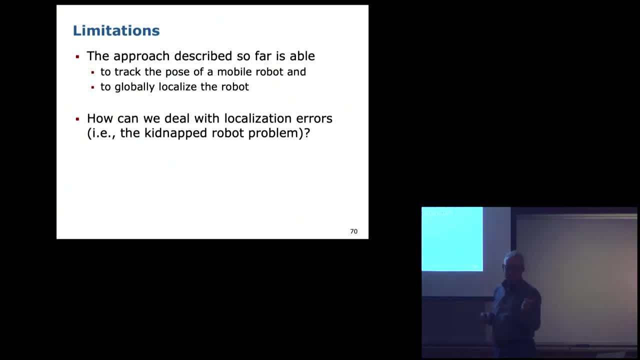 And then you would actually at every time step you would guess that robot is somewhere else. One minute, yeah, we'll be done in a minute, And there's one approach for doing this. disadvantage is that the robot actually at every point in time. 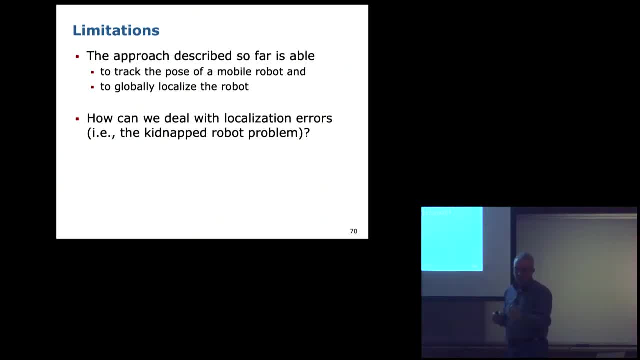 guesses. oh, I might be in the Starbucks next door or so. And if all of a sudden the measurements are consistent with that for whatsoever reason, because there are people around and it looks like the Starbucks restaurant, and all of a sudden, all the probability? 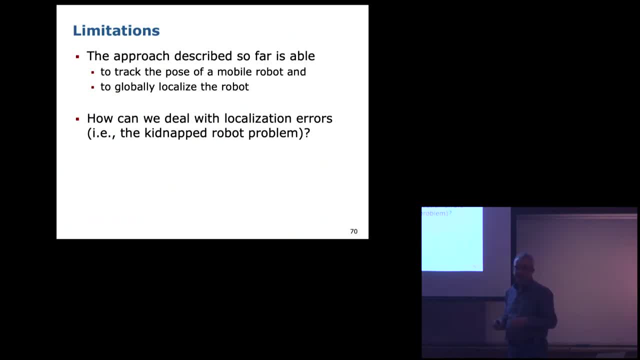 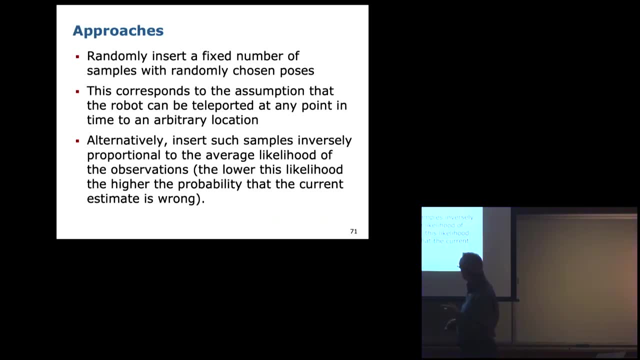 marks will shift over and the robot will actually believe it has been transited, And there's no reason for doing this when the robot is actually happy with its observations. So what people have been doing is either what I mentioned- randomly guessing new places- or the alternative. 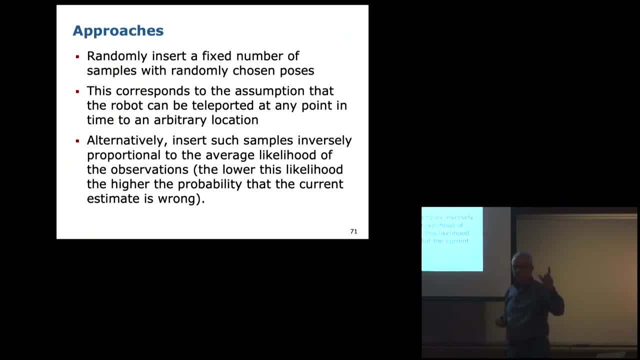 is to look at the average likelihood of your observations. Basically, if they drop, meaning that the robot is unhappy with its observations, Nothing fits really, And that is something that you can do. You generate the statistics about what is a typical observation likelihood that I 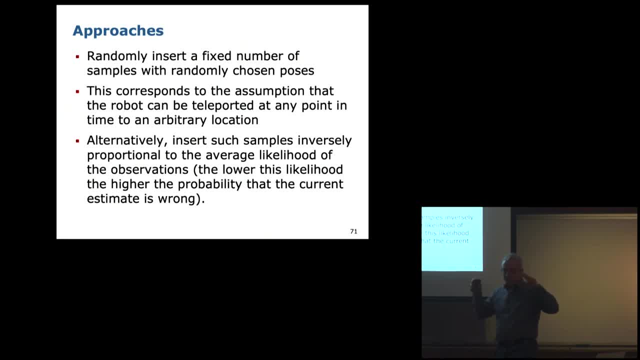 have when I'm happy. Then when you get below that threshold, you would even learn that You could basically say: OK, I'm proportional to that. I'm guessing random locations And the more unhappy I get, the more willing I am to accept being somewhere else. 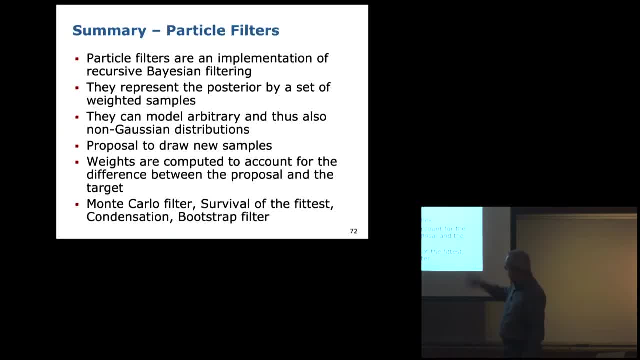 And that's actually the most robust approach for doing that. That is the summary, And with that I'm basically done. I hope you enjoyed it. I did it And, yeah, see you. Sorry, Let's go. Thank you, Professor.